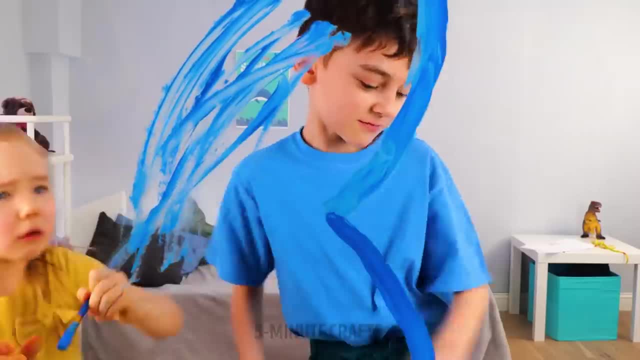 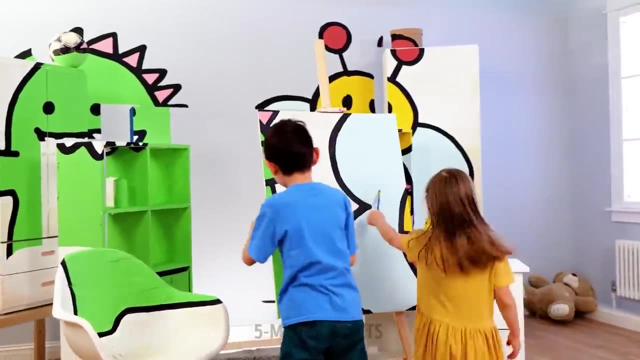 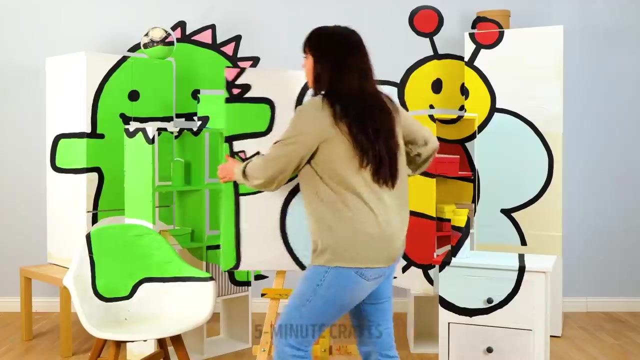 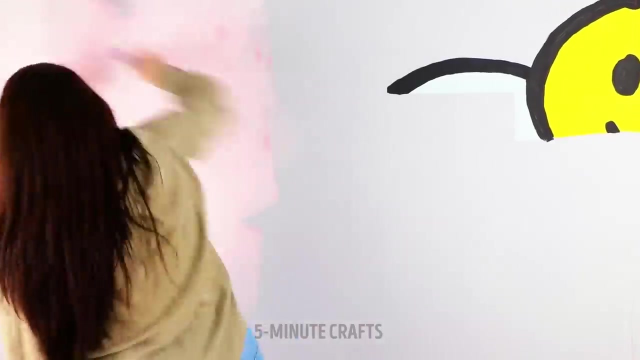 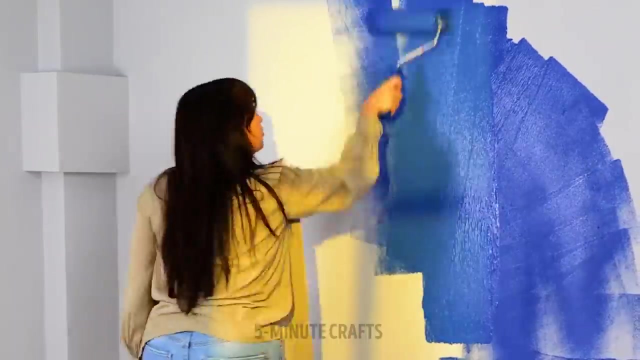 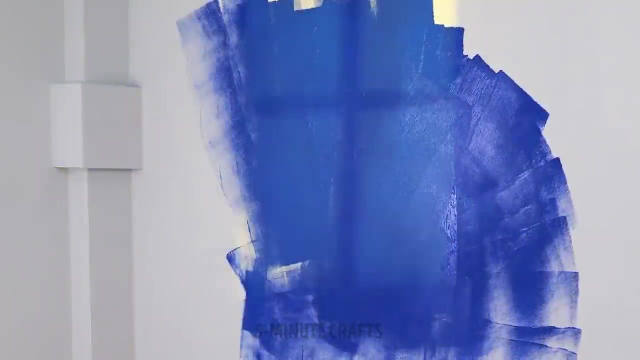 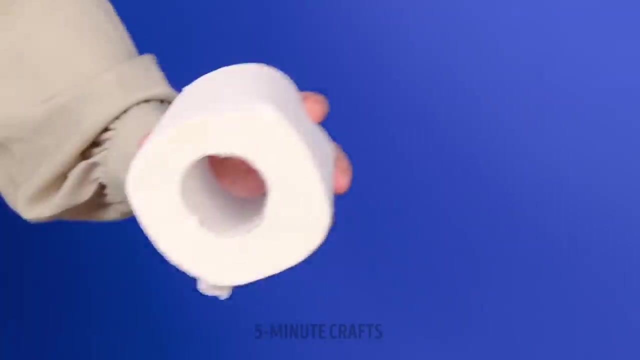 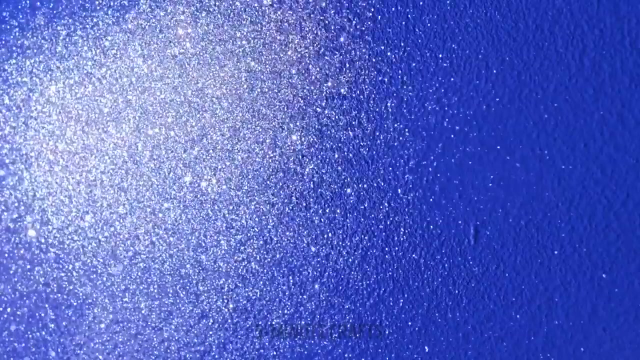 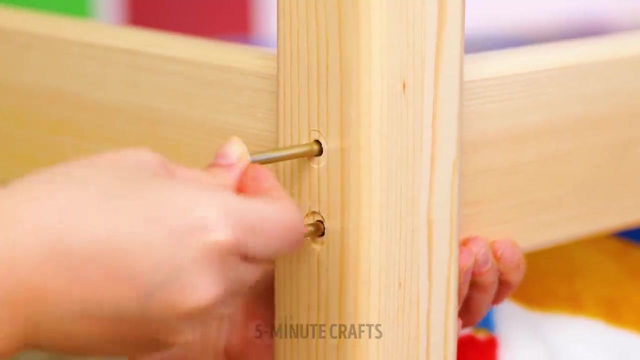 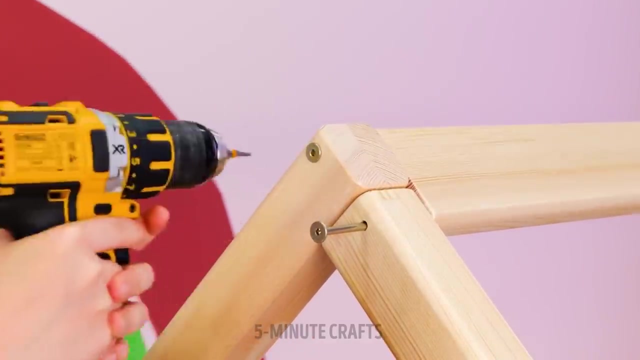 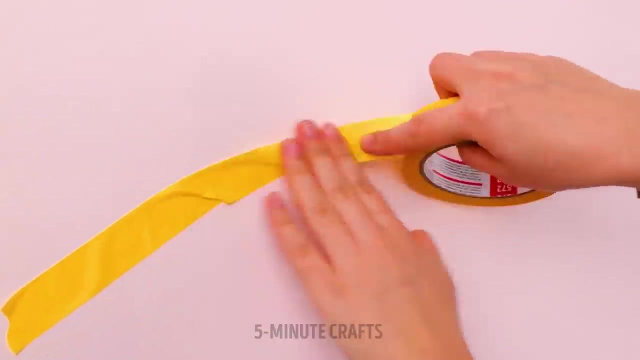 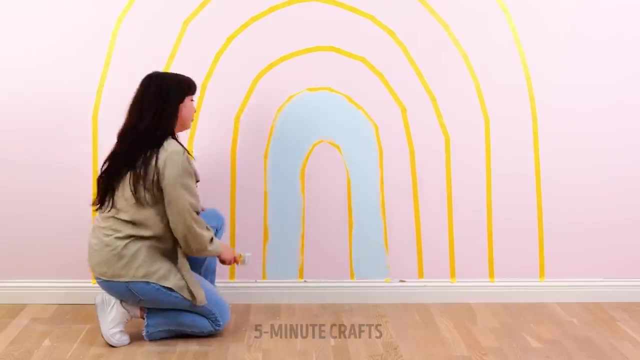 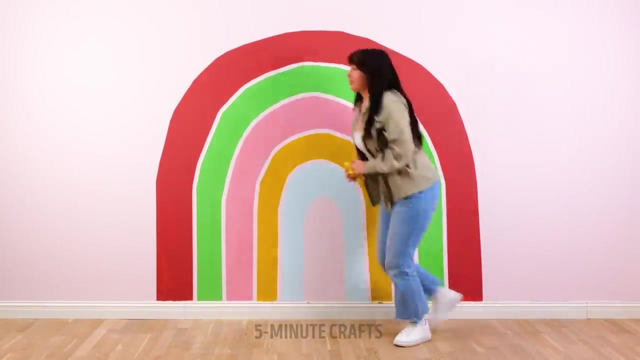 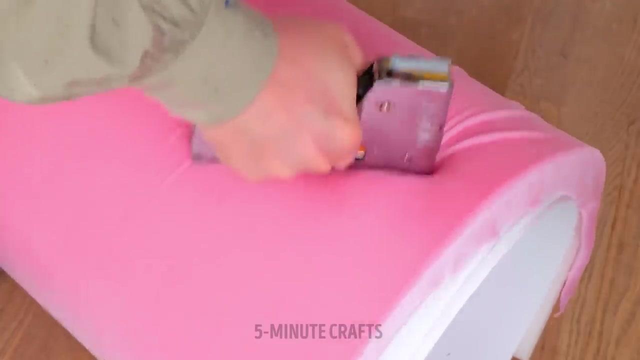 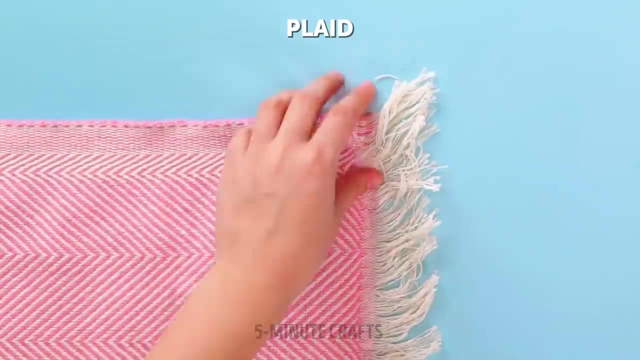 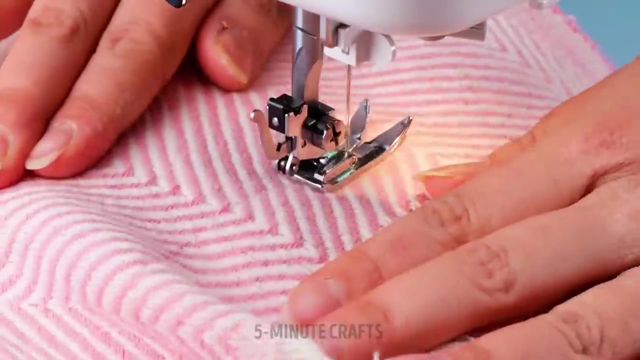 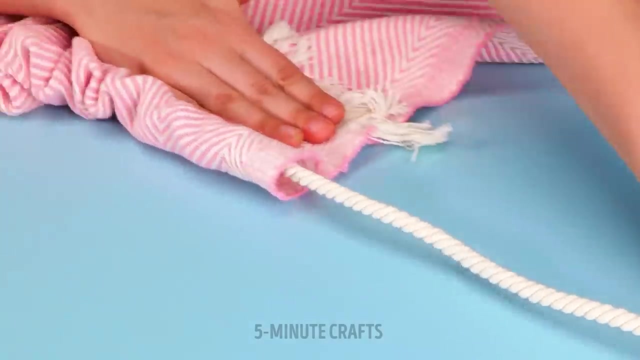 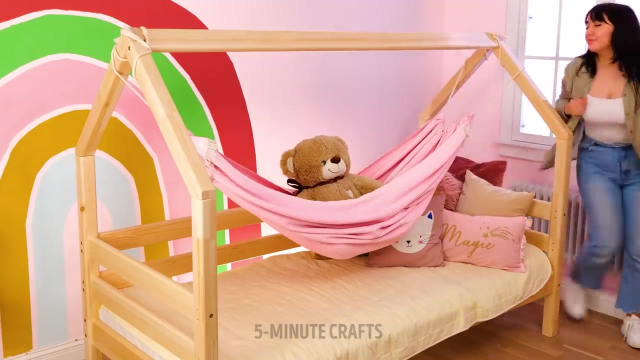 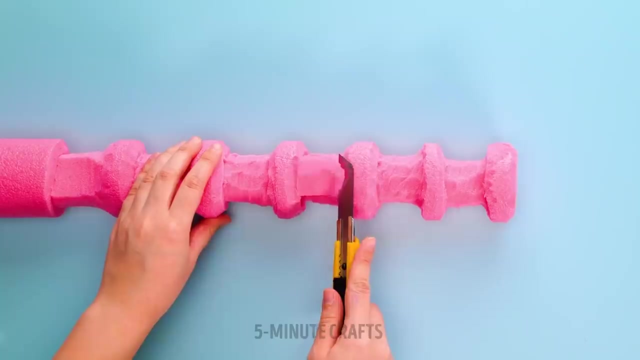 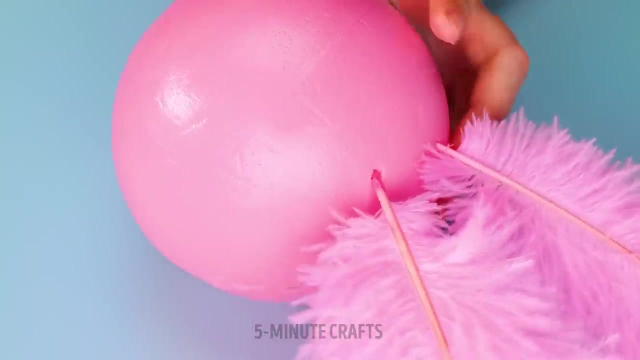 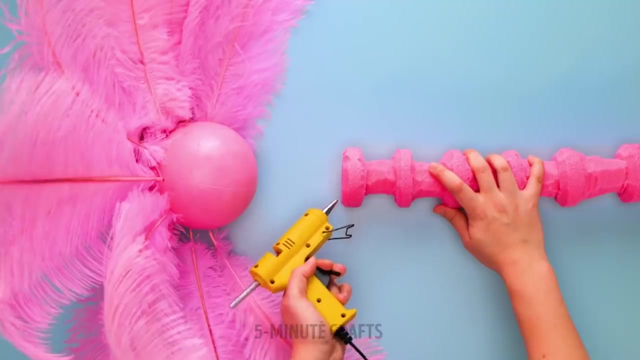 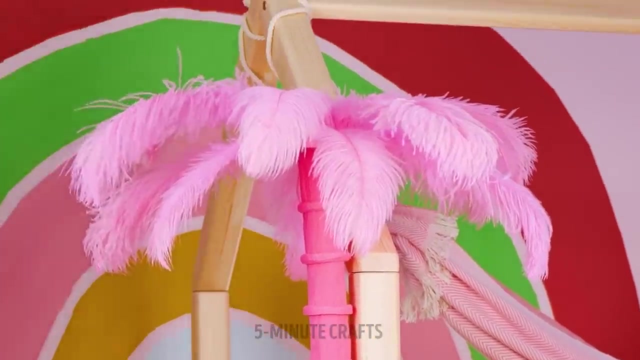 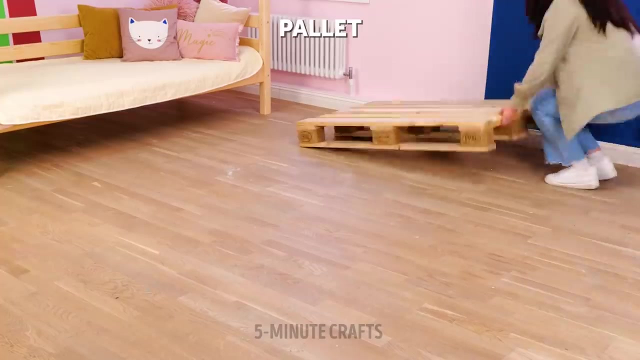 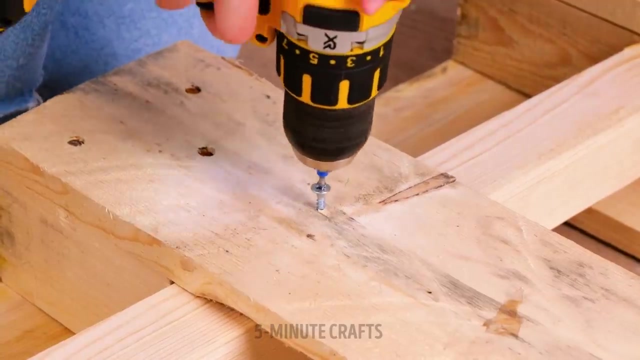 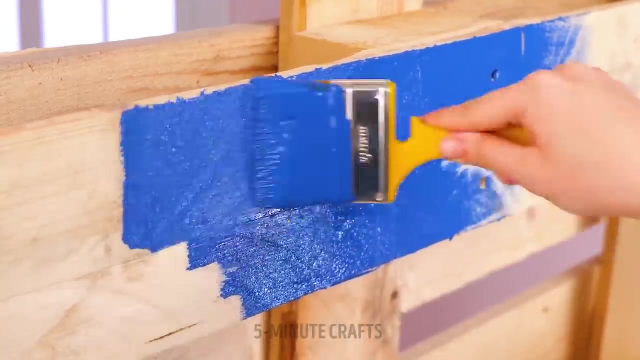 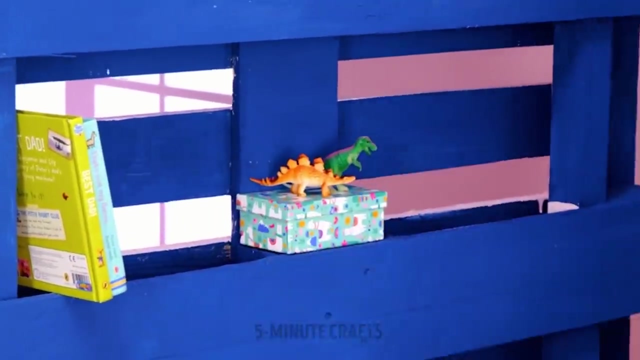 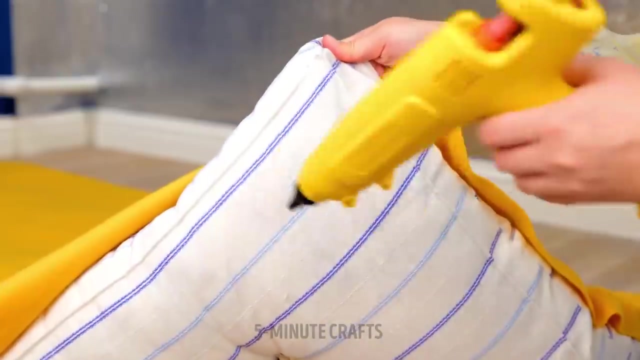 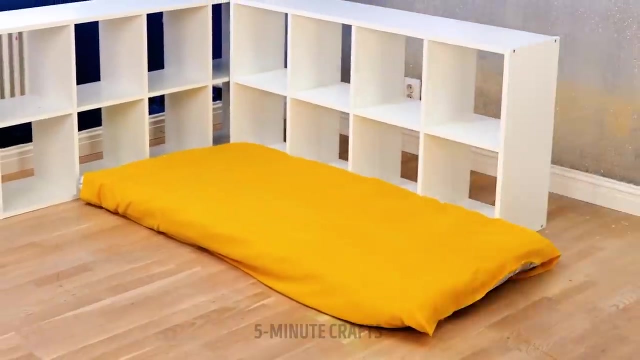 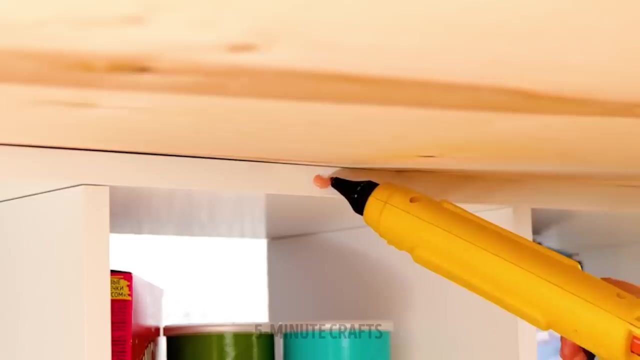 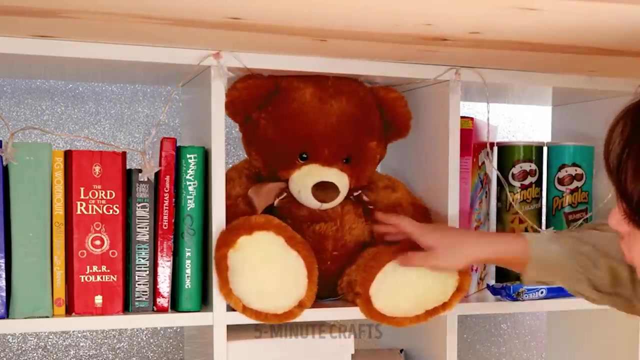 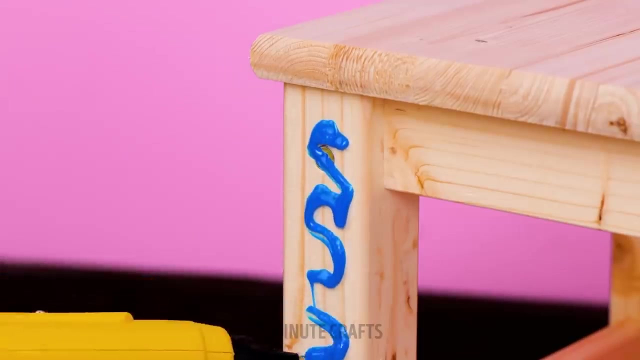 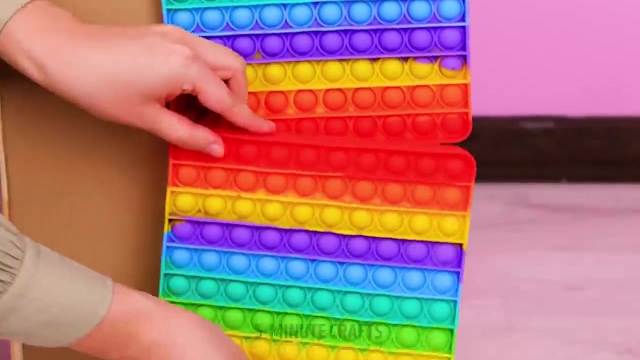 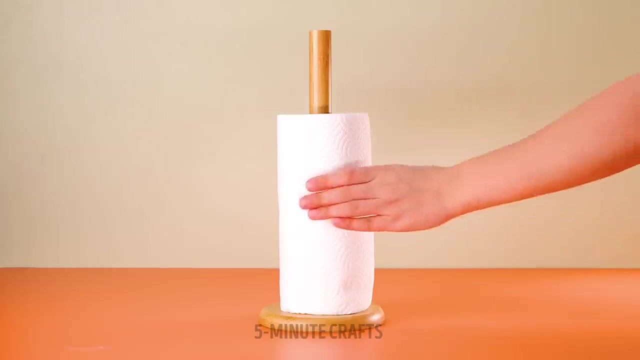 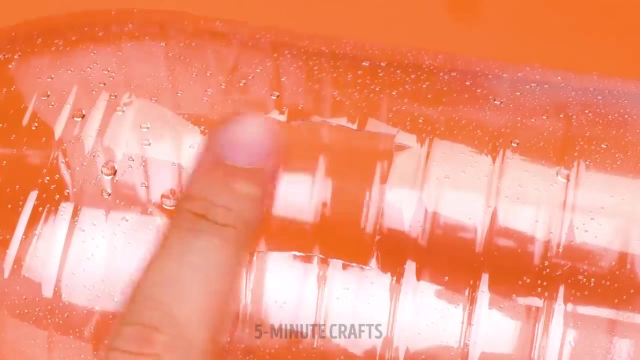 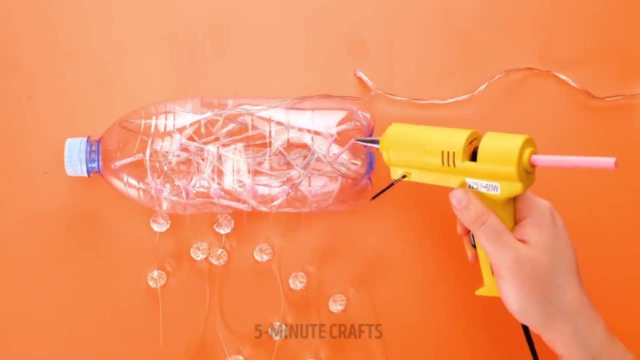 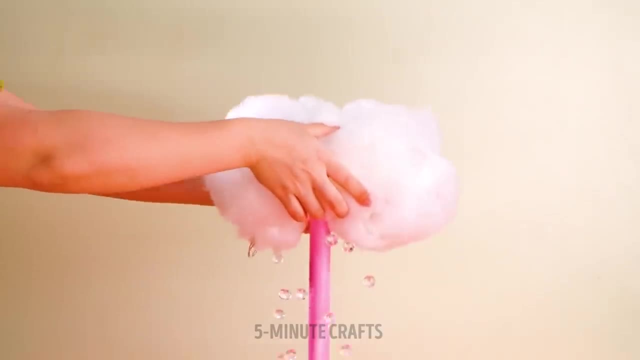 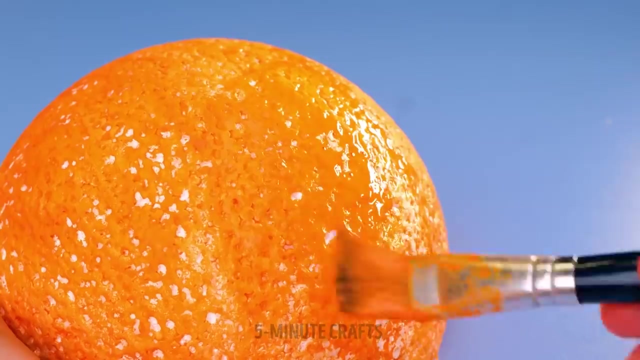 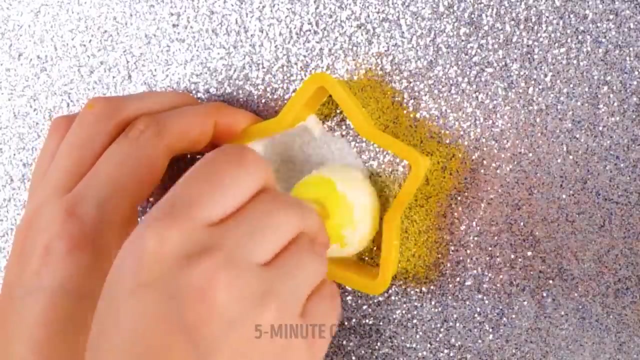 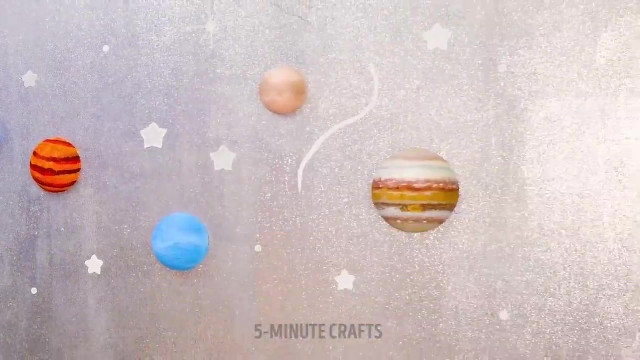 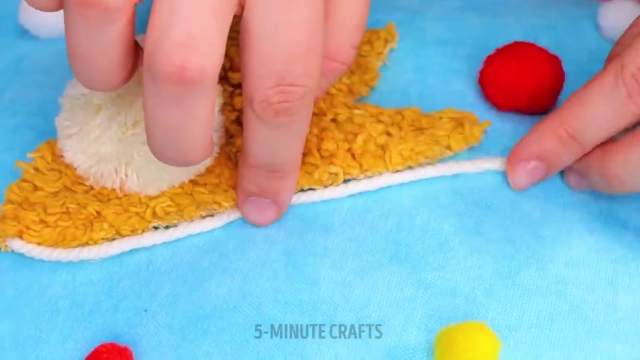 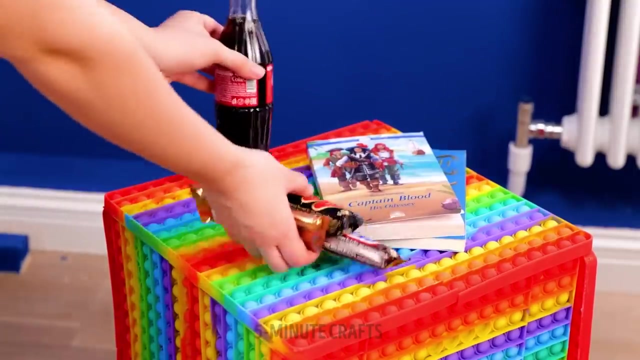 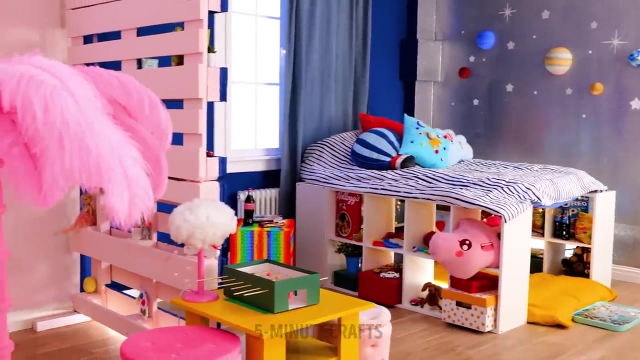 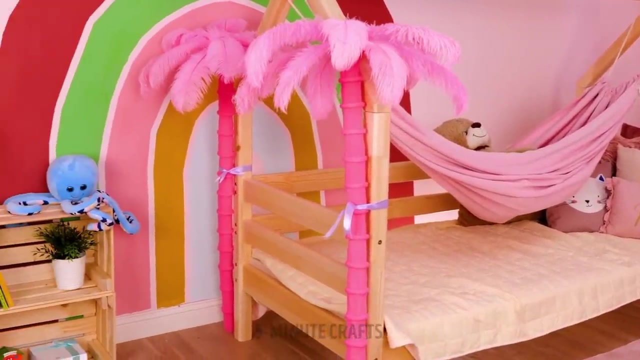 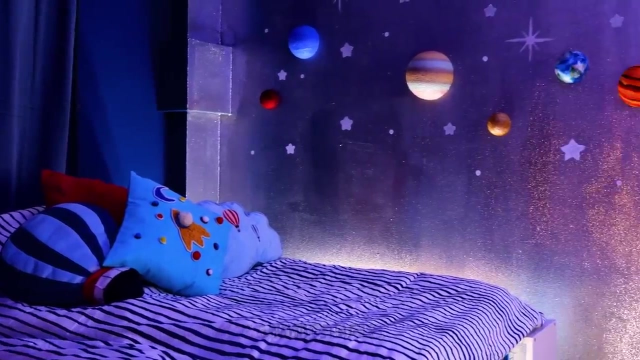 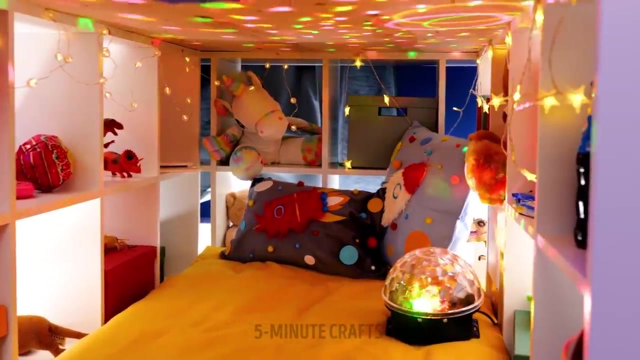 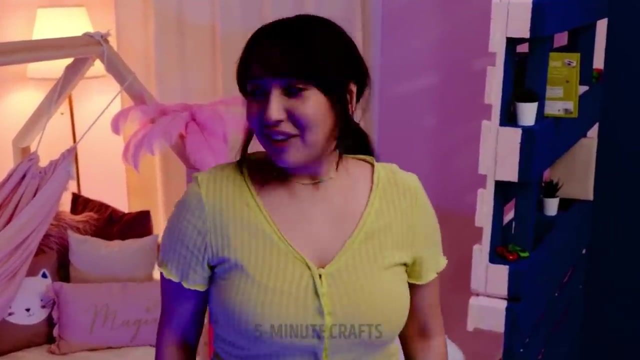 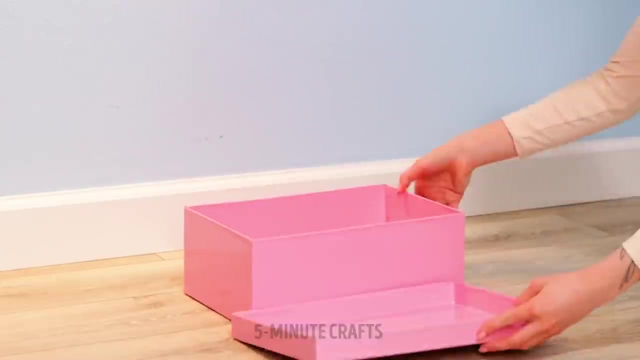 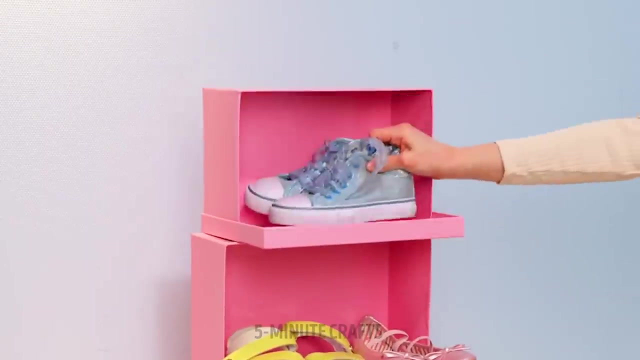 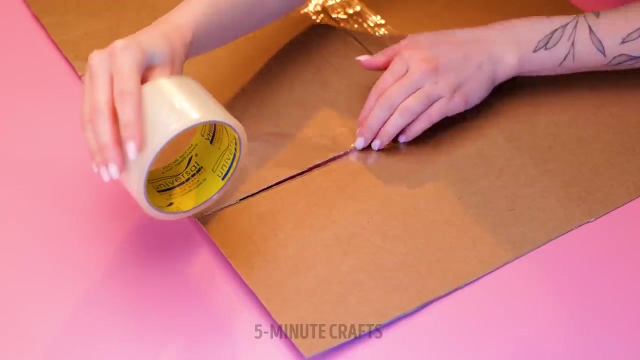 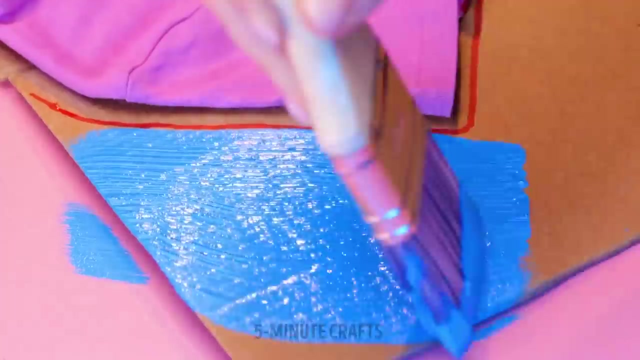 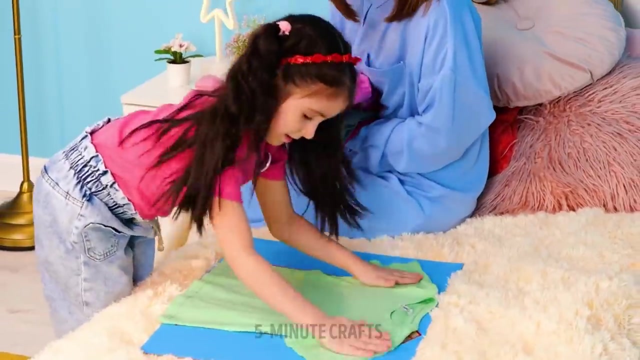 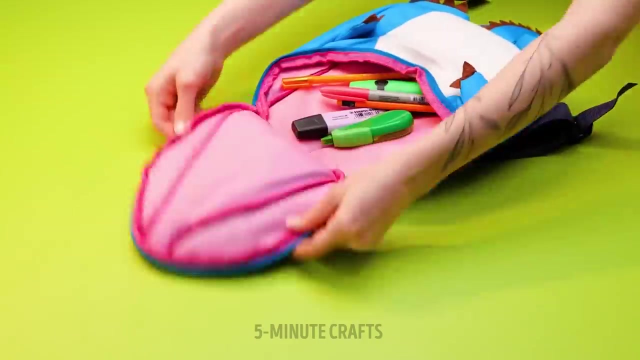 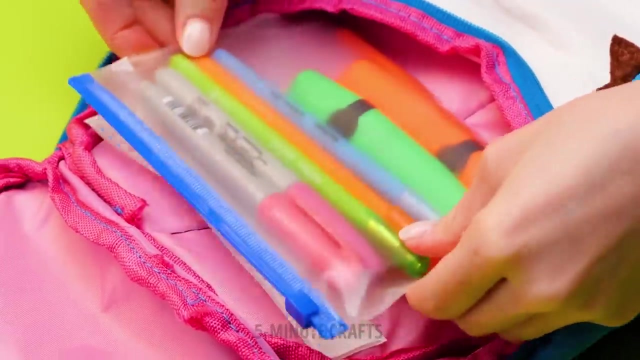 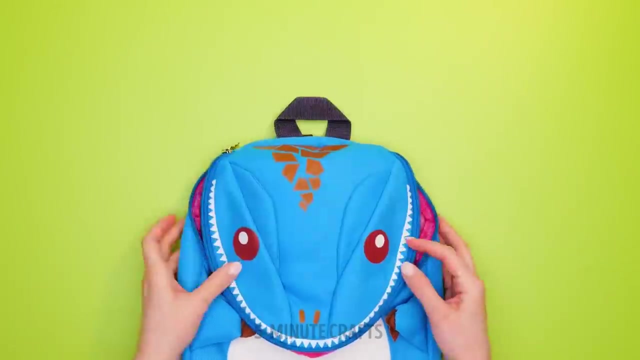 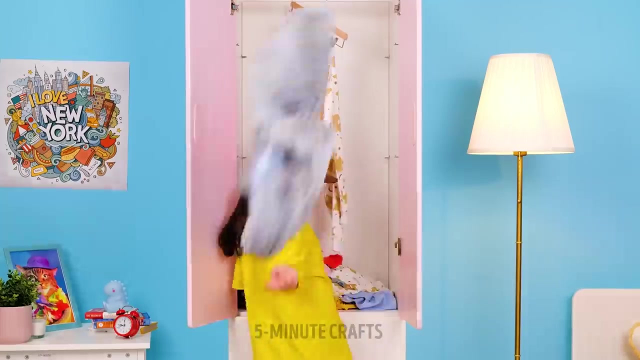 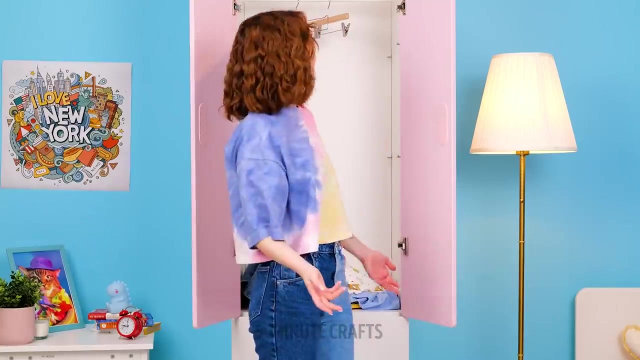 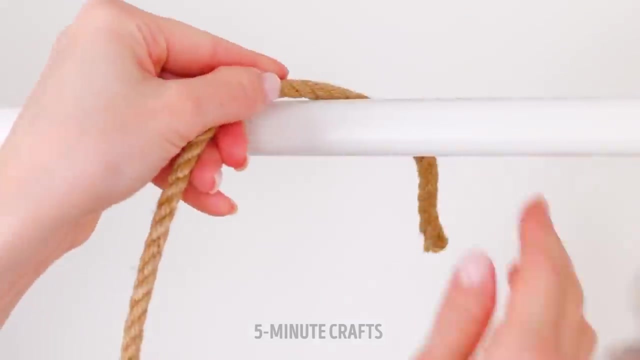 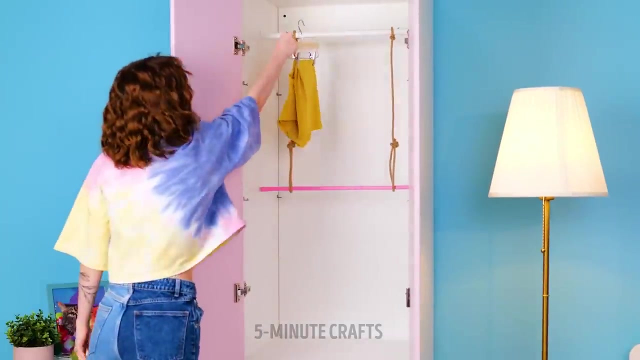 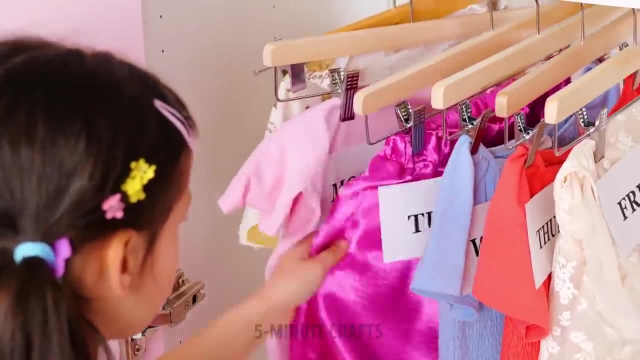 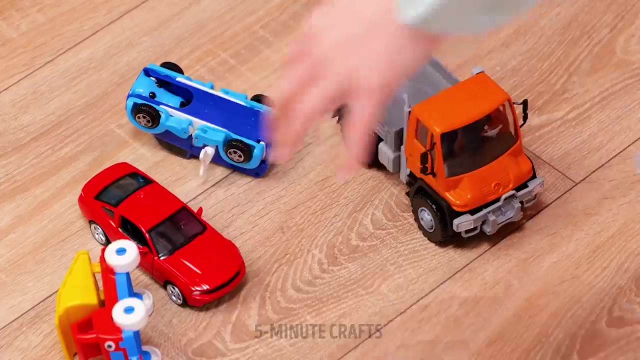 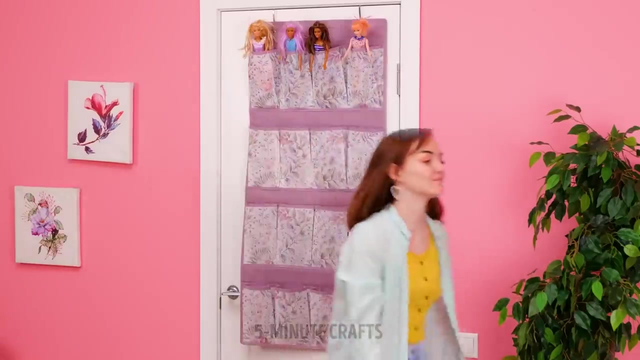 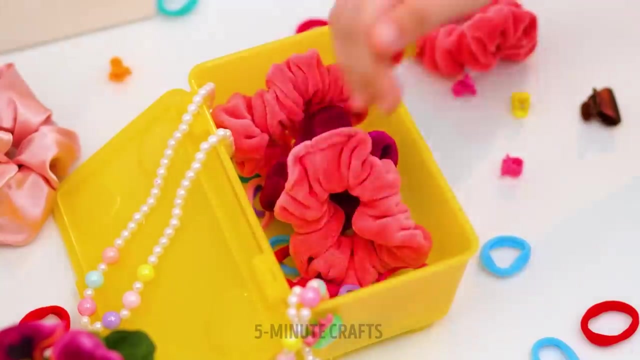 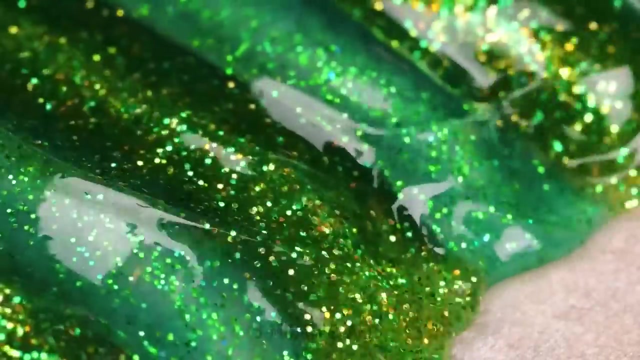 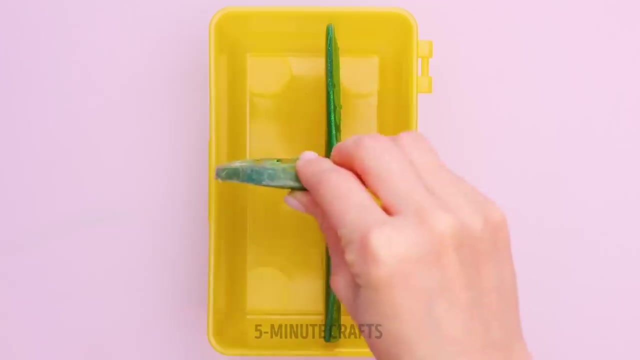 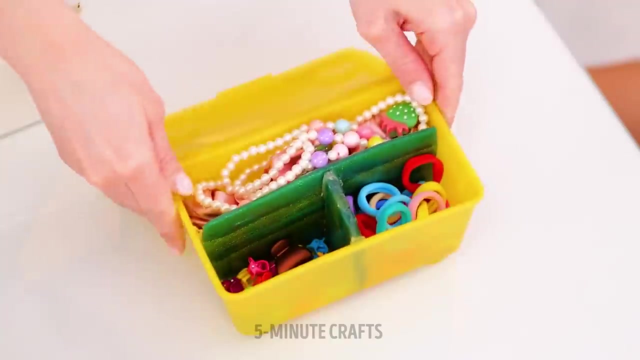 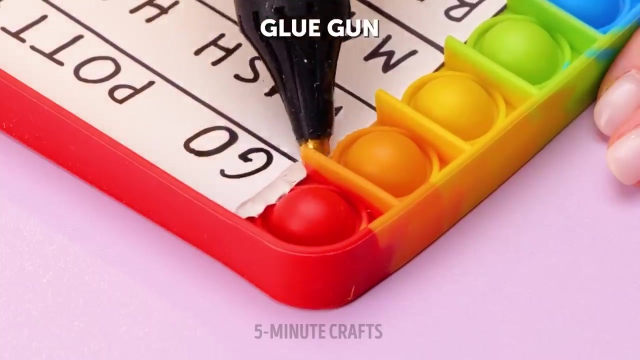 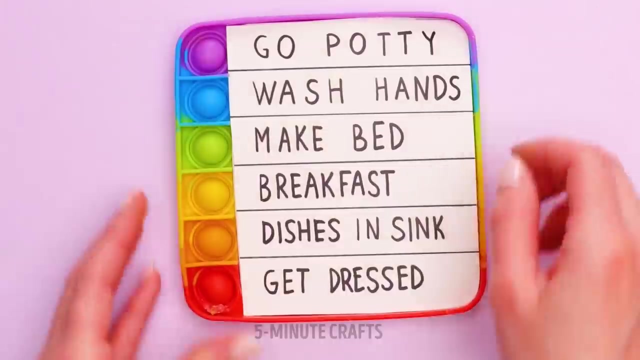 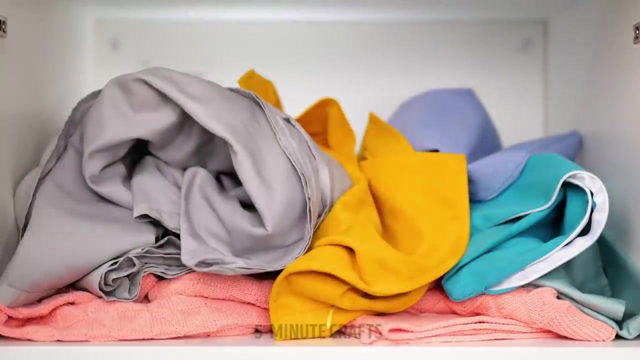 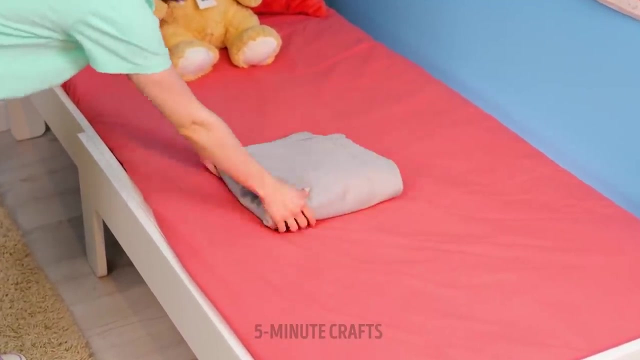 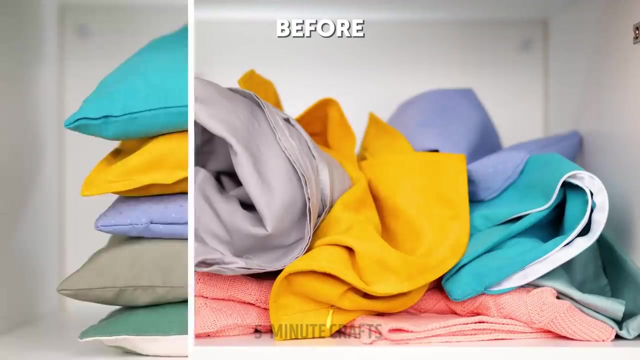 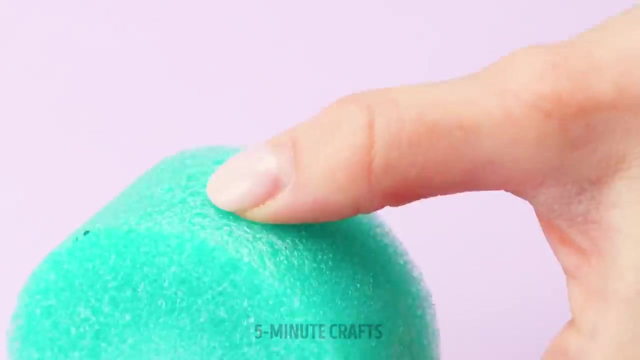 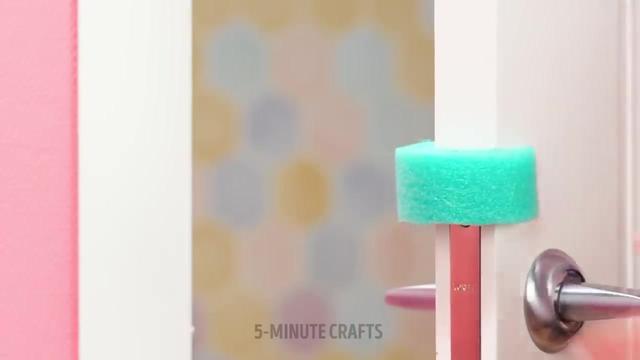 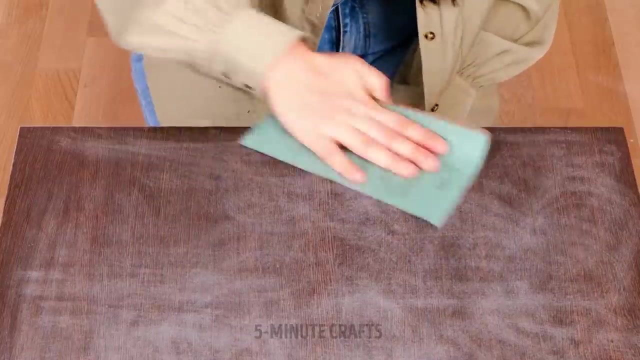 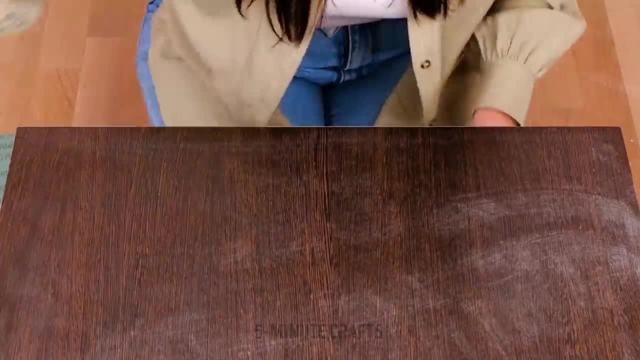 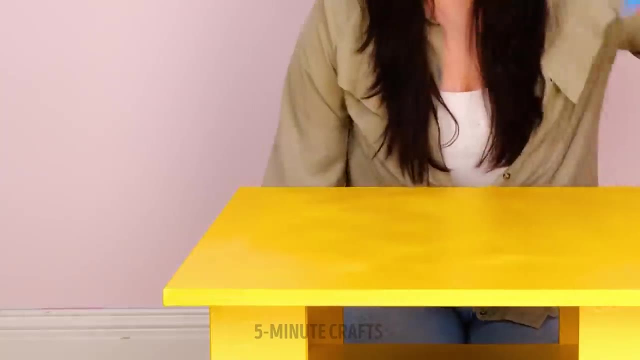 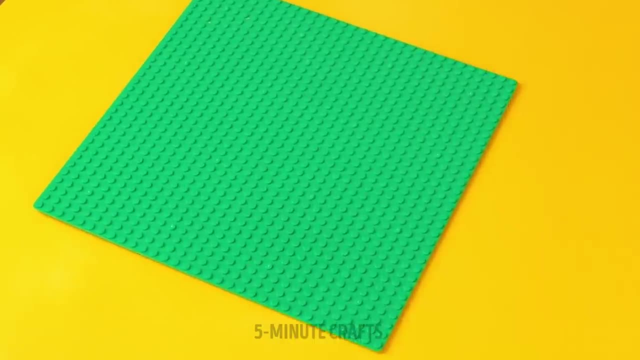 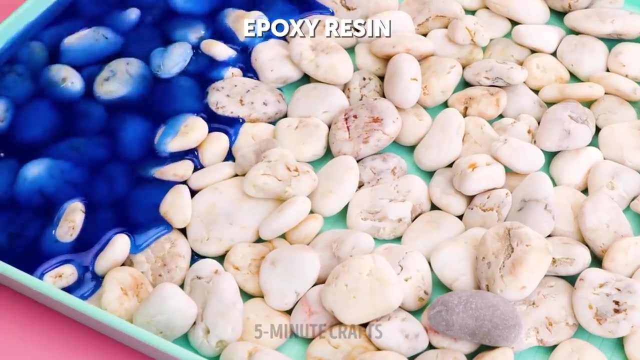 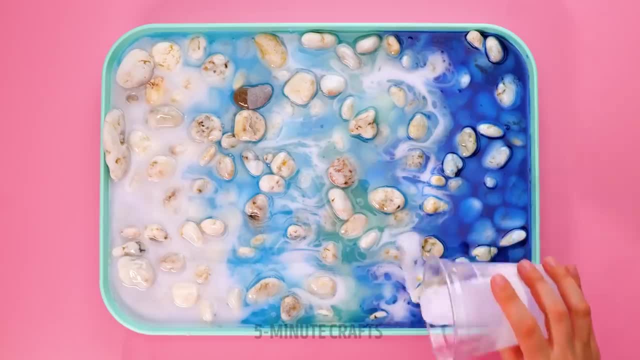 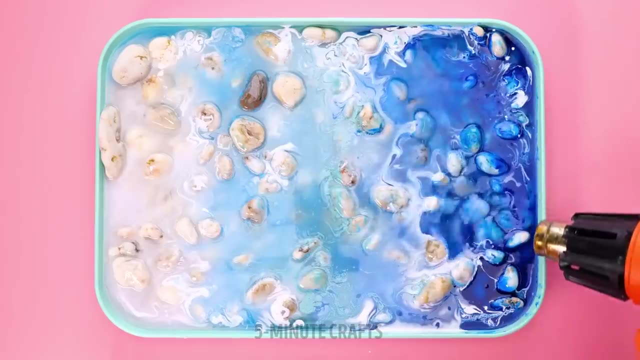 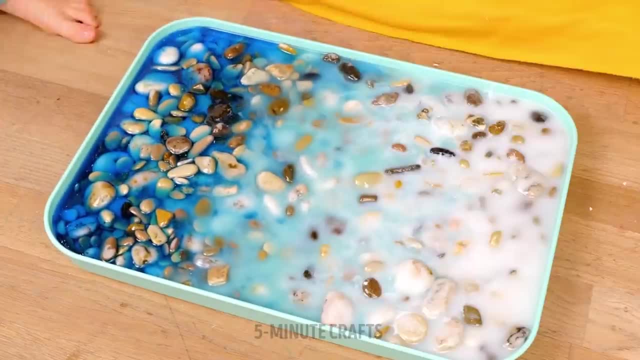 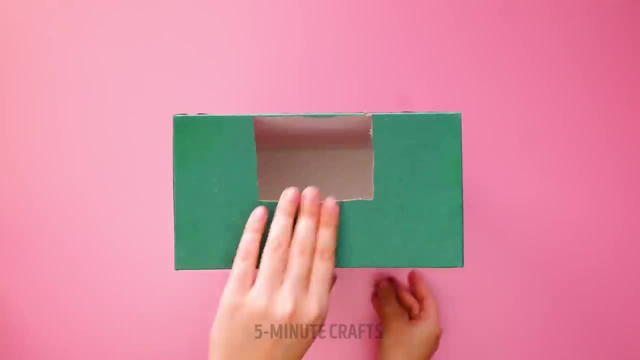 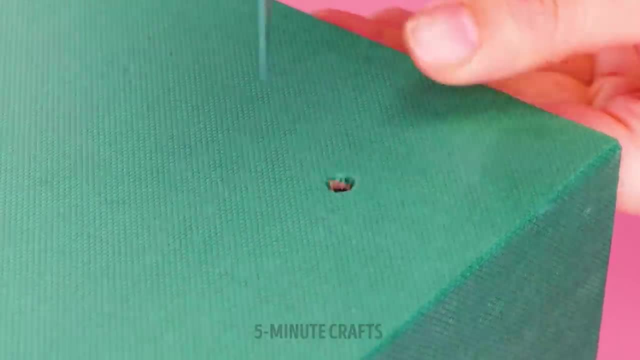 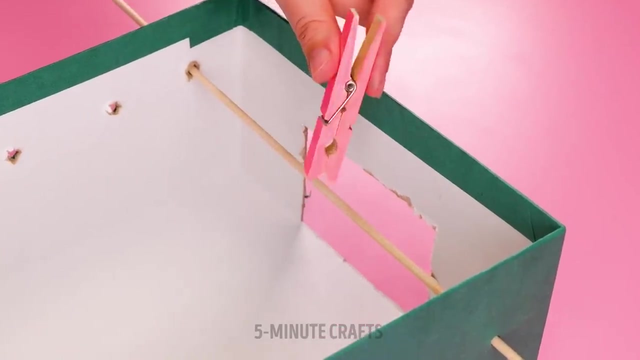 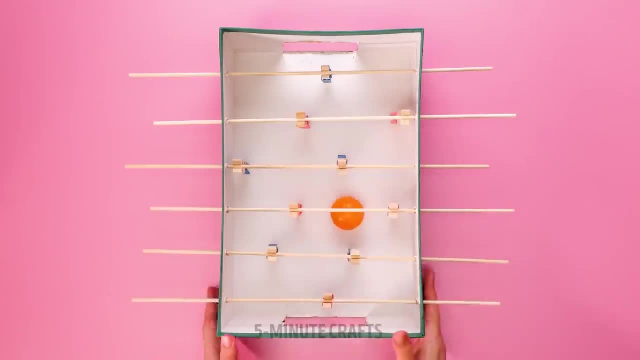 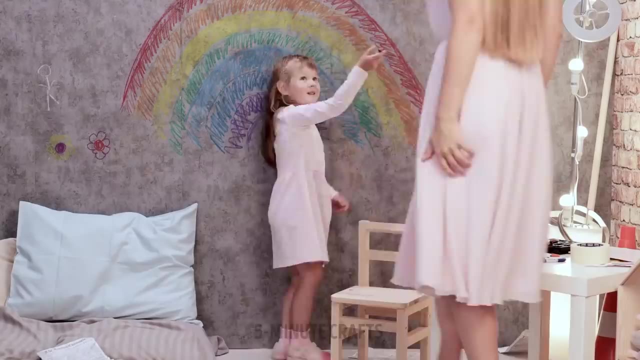 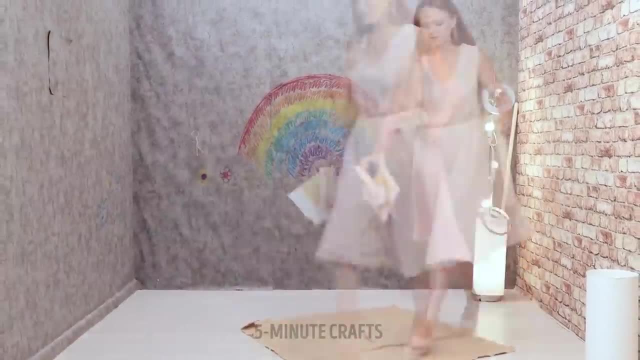 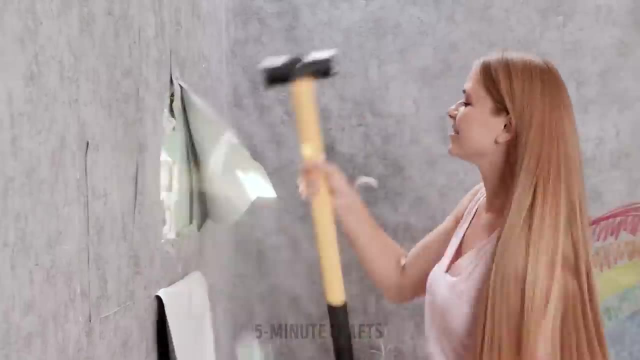 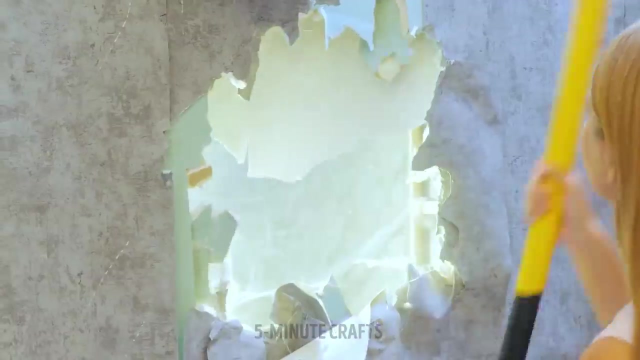 Get in the fast lane, babe. you can make it. I promise I'll be there all the way And if you get a little broken down I'll let you down. just keep your head high. Let's get this out of your way. I can't wait another day. To have you. you shouldn't wait. don't be so afraid. Yeah, I'm a bit too much, but I'm fun and games. When I'm at the top, I just wanna play. If you are looking for one hell of a ride, just come and get it. baby, I'm all yours. 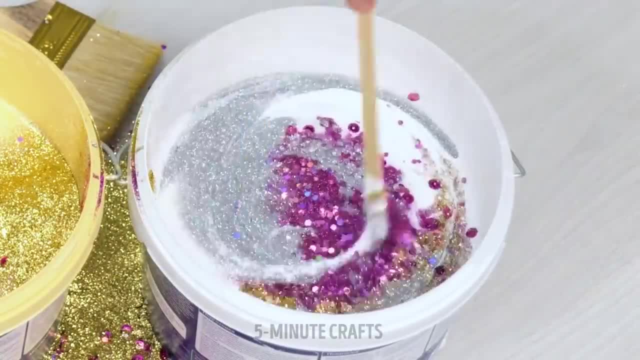 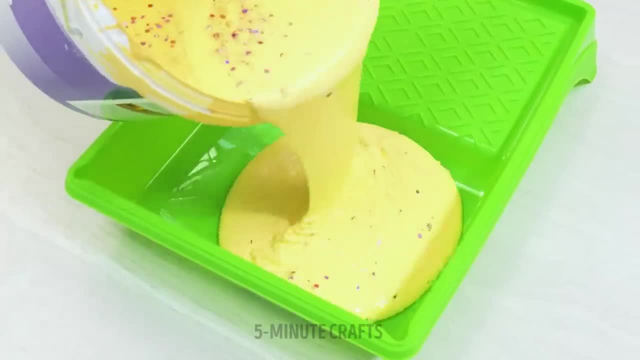 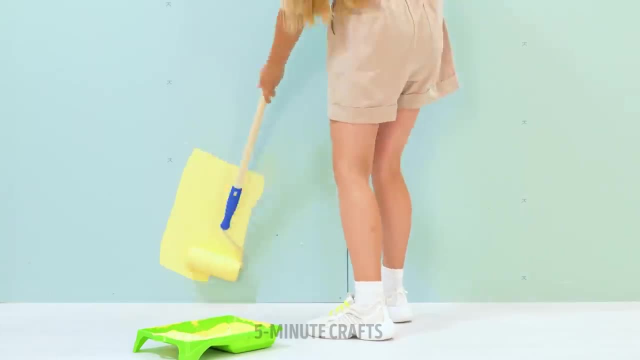 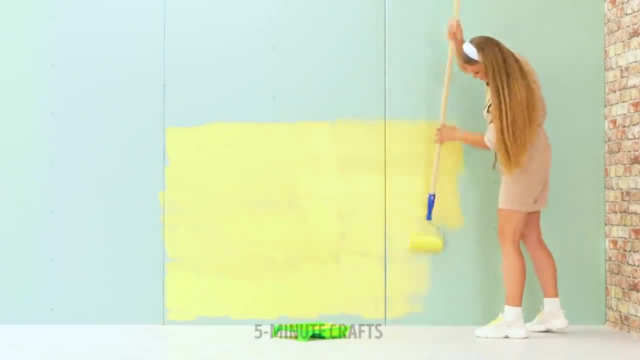 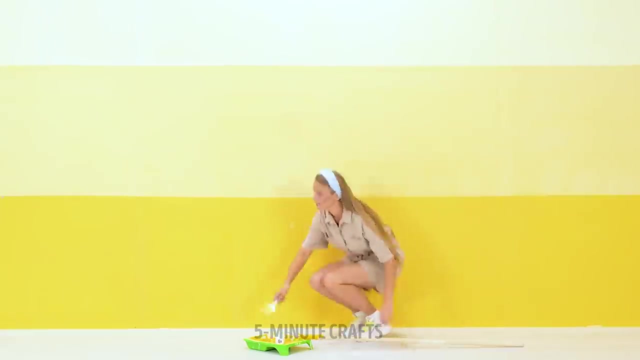 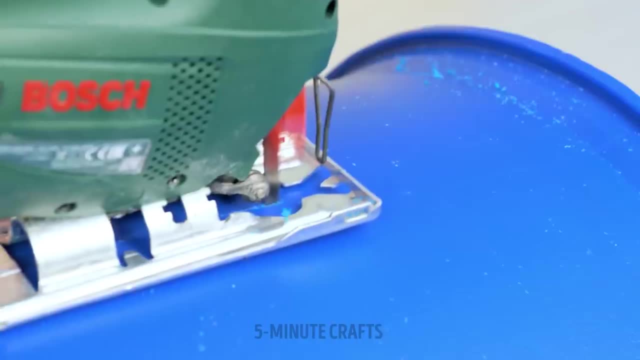 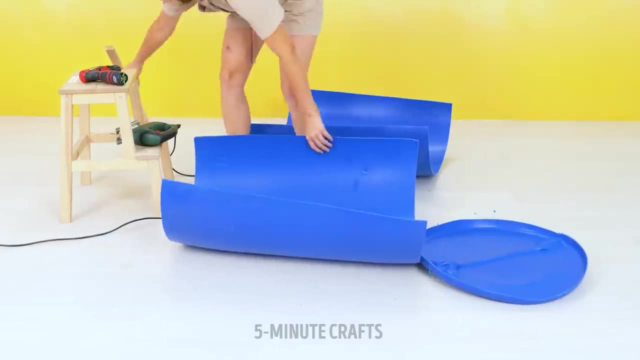 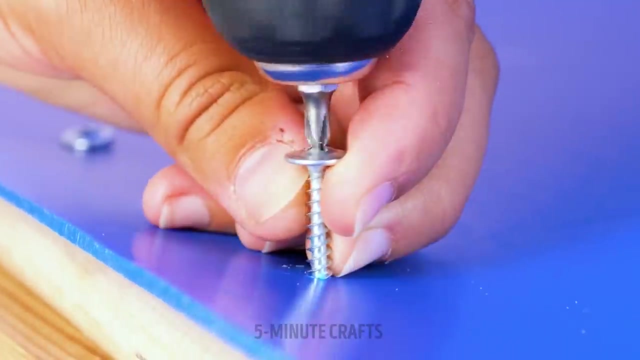 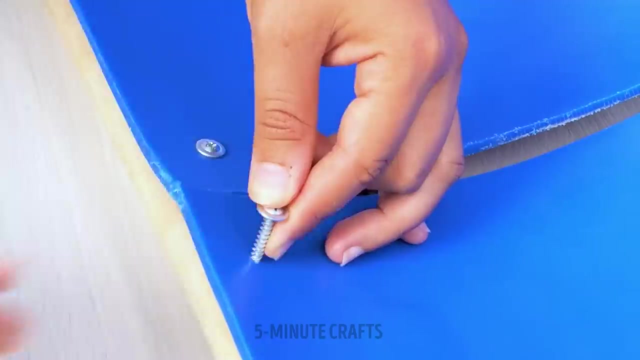 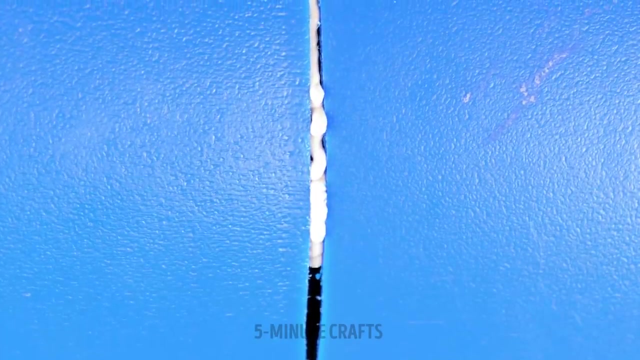 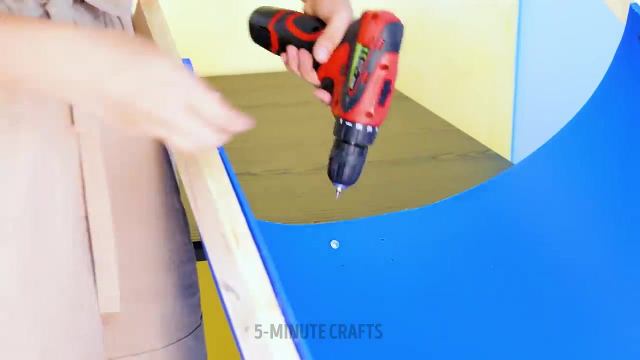 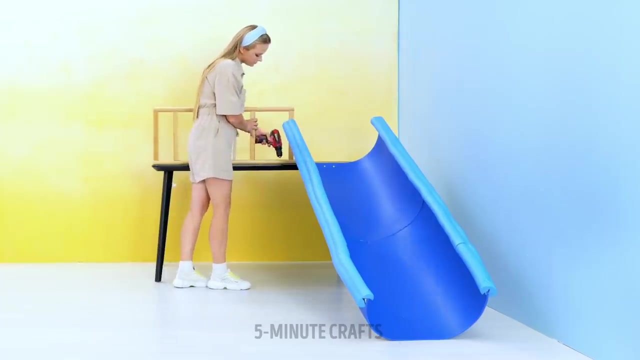 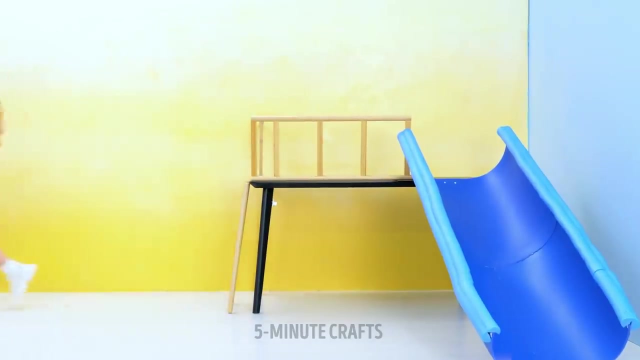 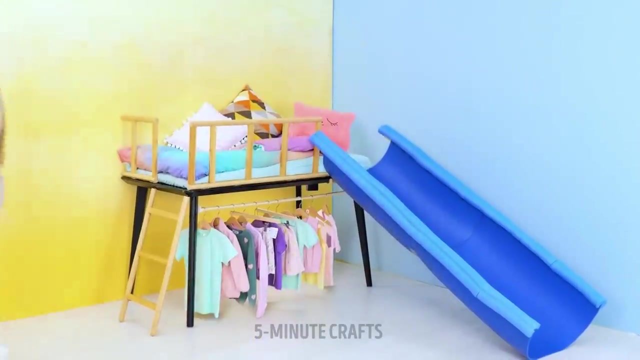 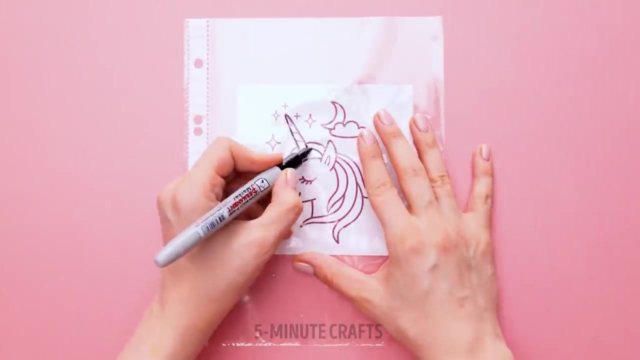 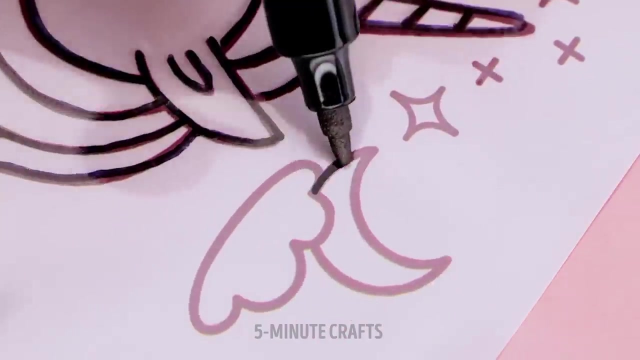 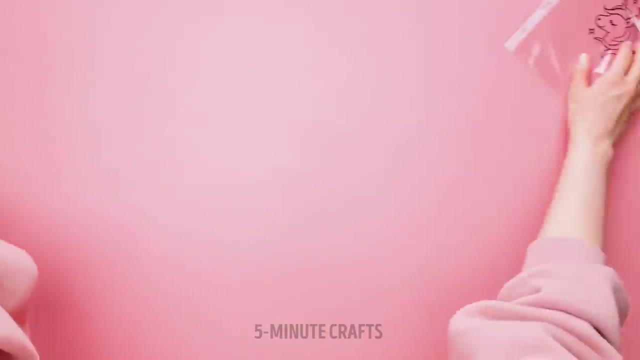 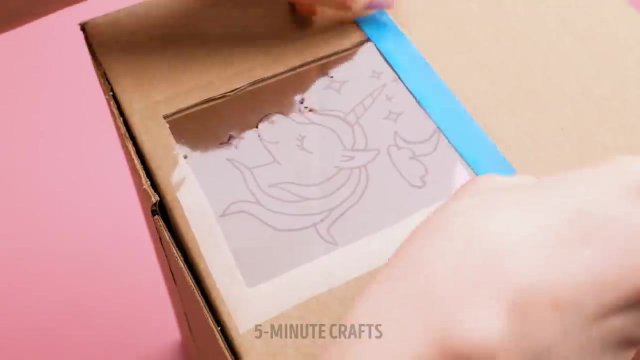 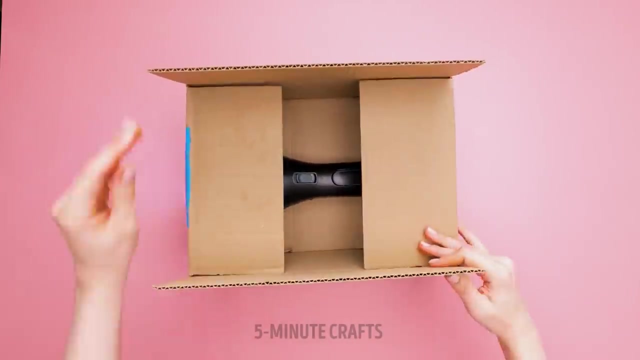 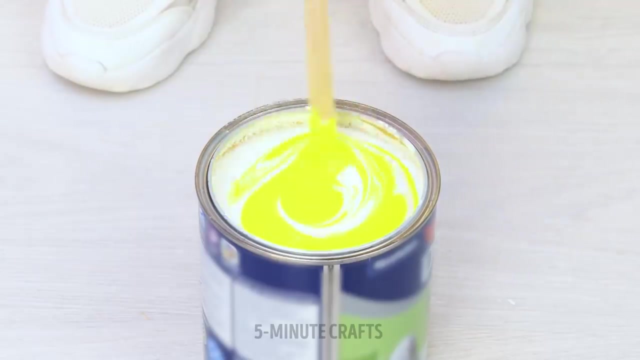 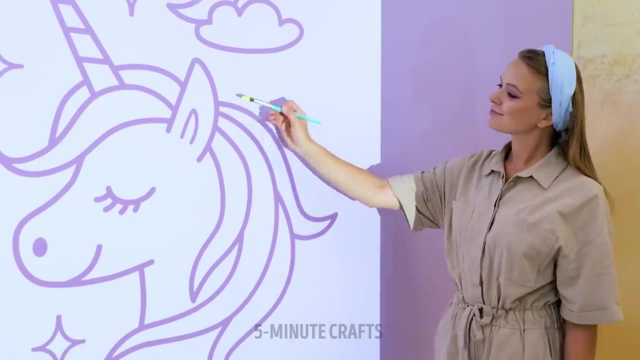 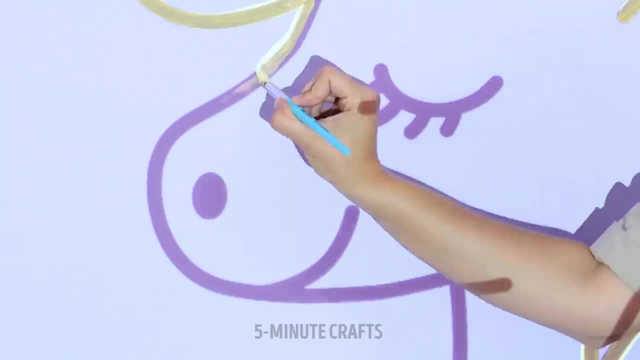 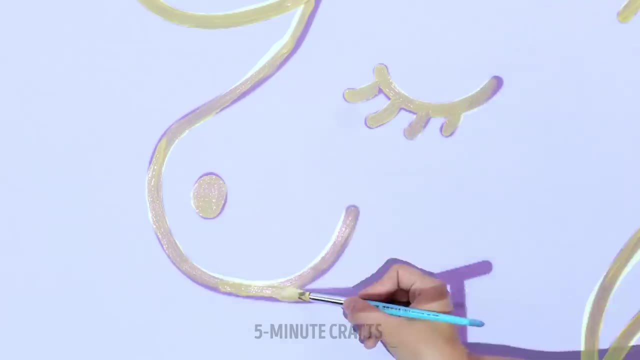 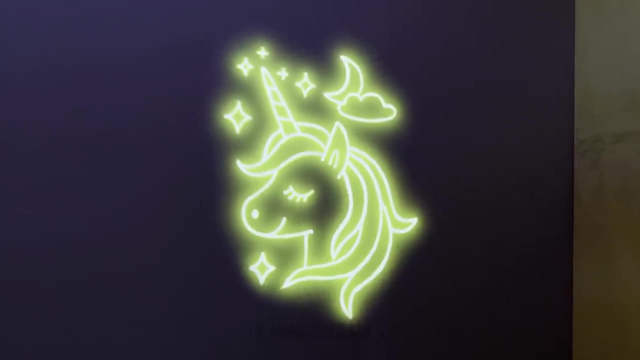 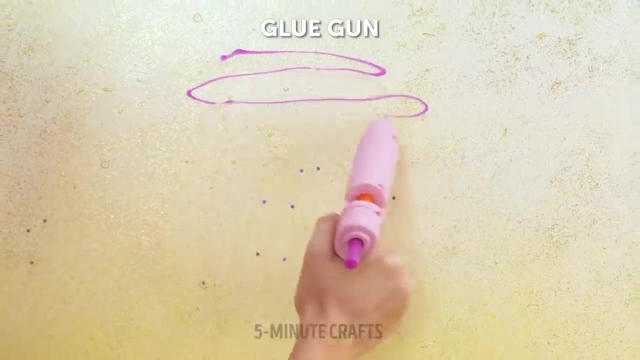 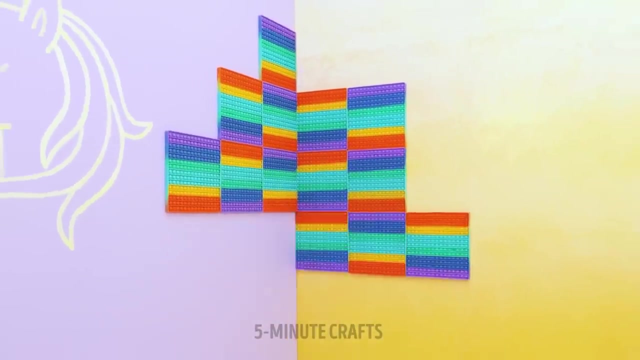 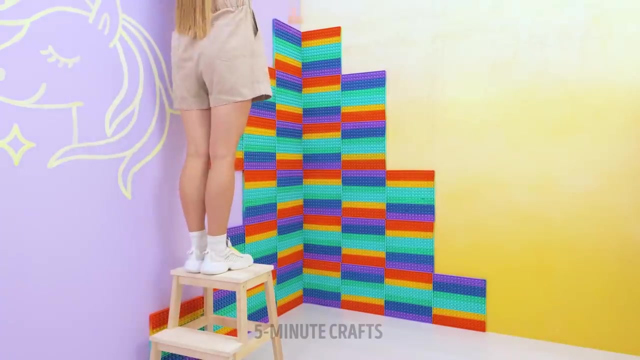 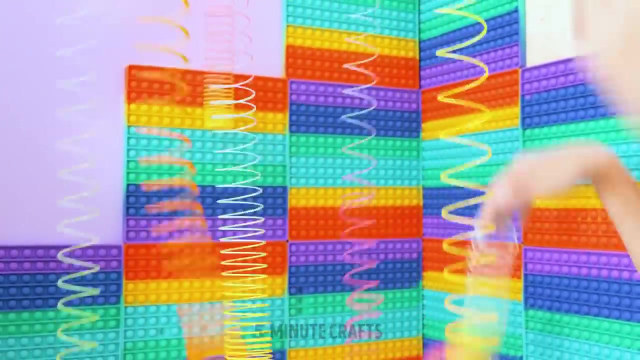 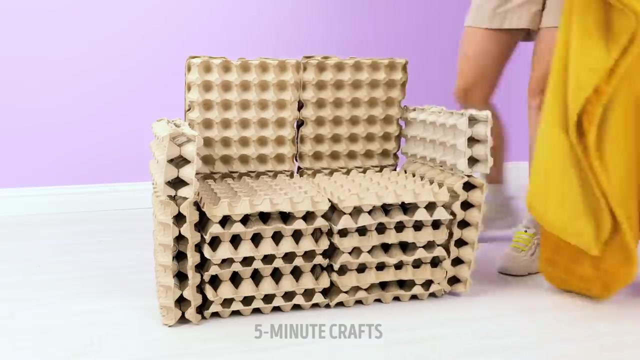 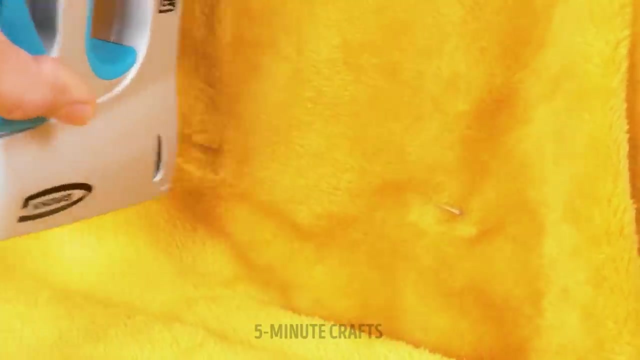 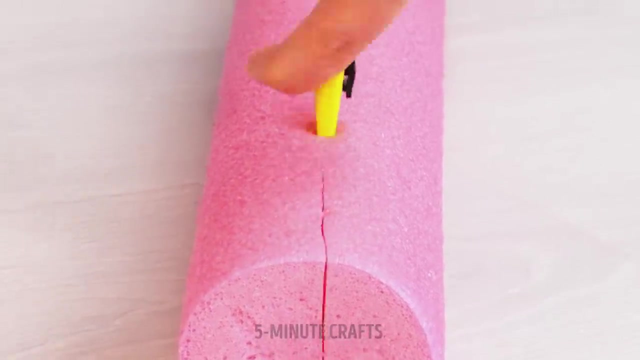 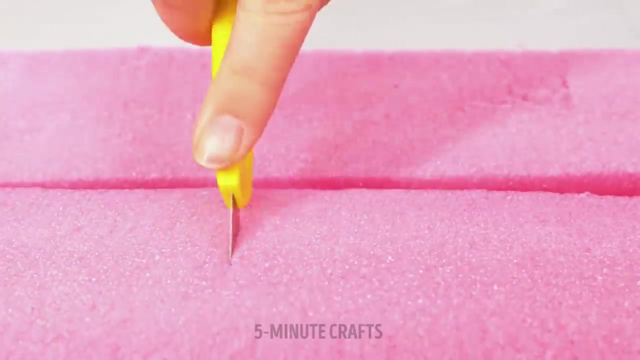 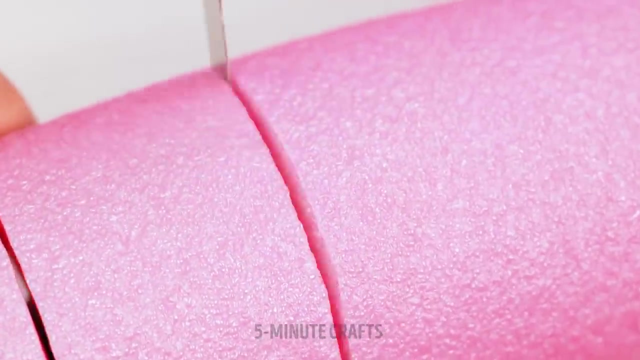 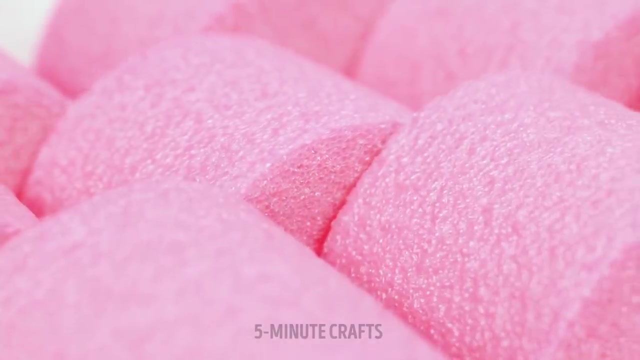 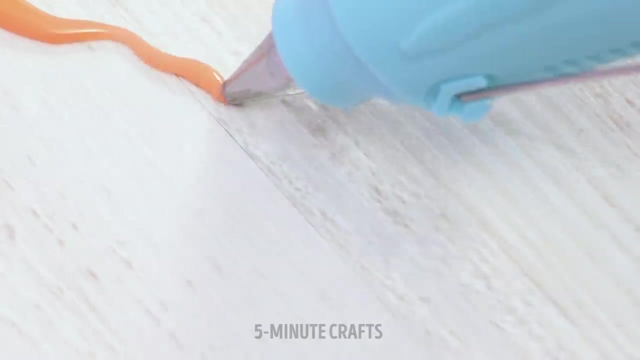 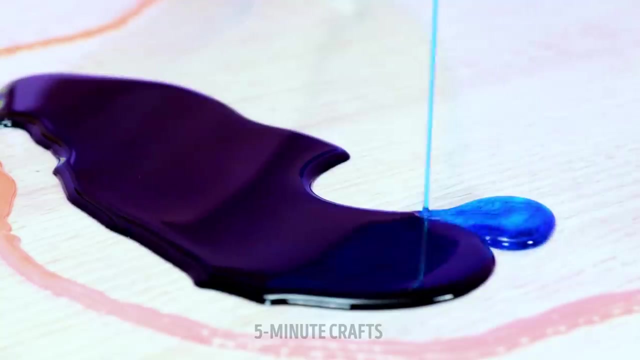 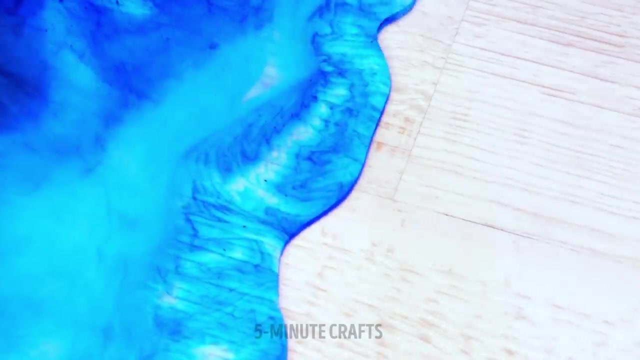 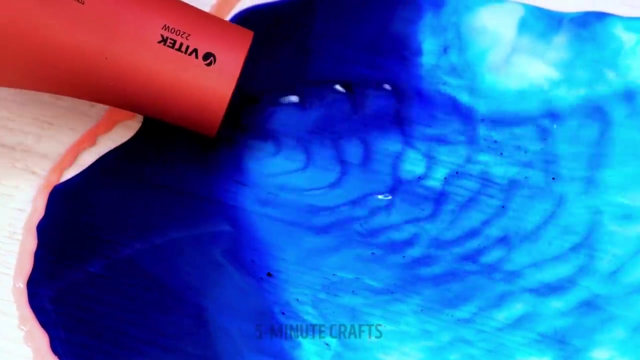 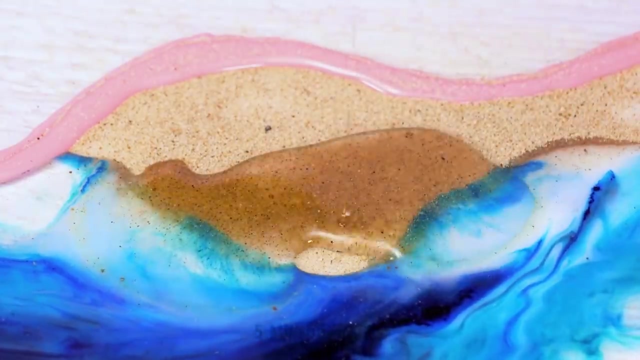 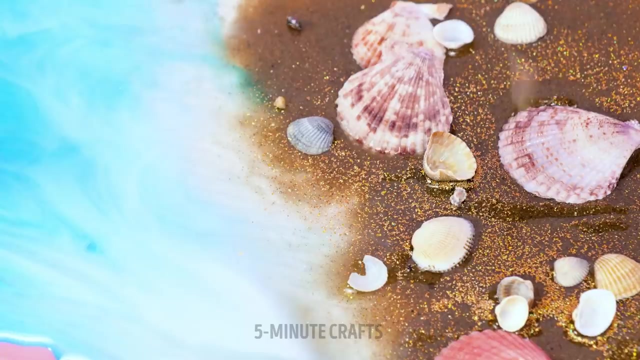 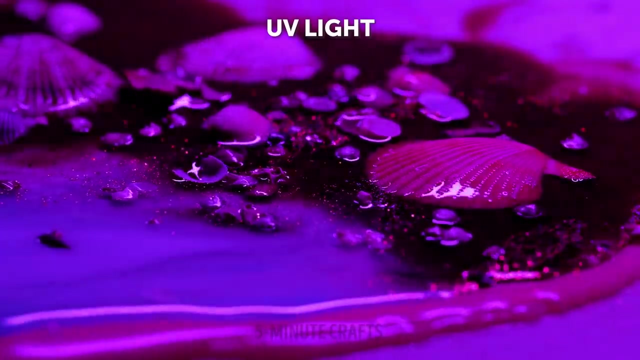 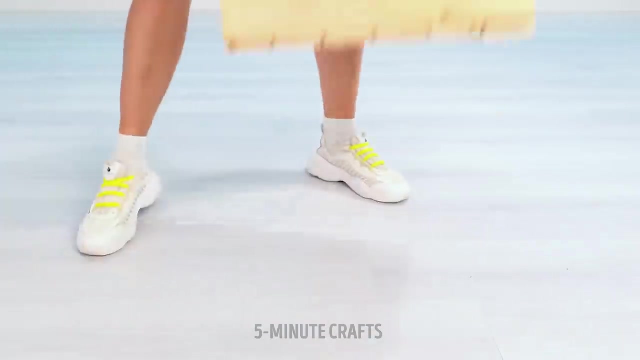 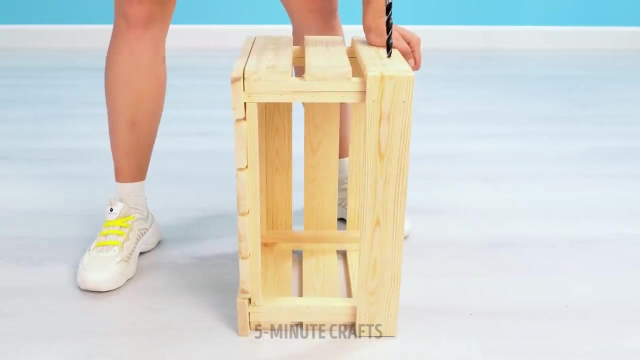 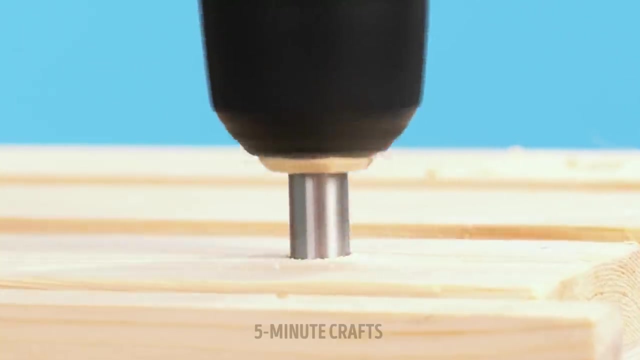 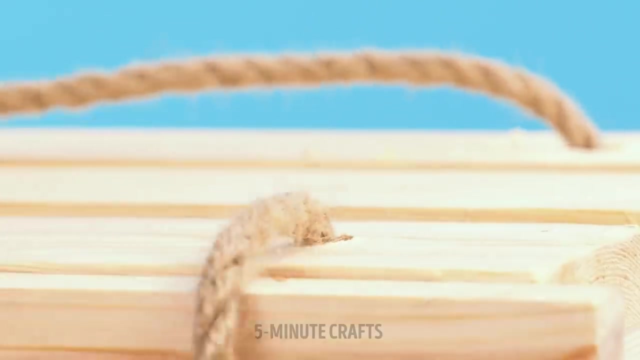 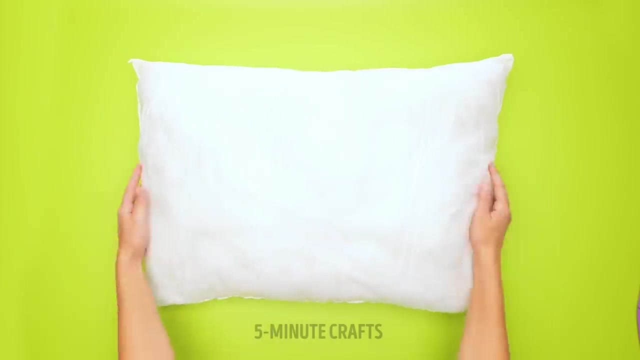 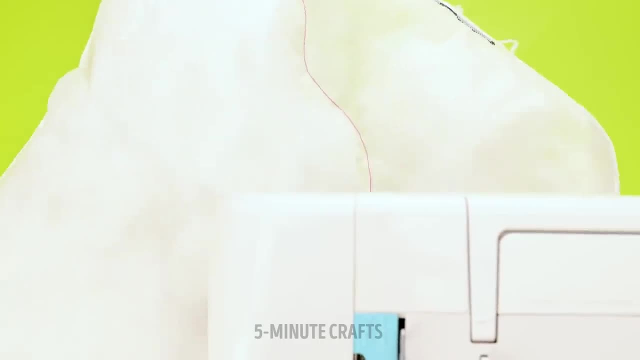 Wanna take a different lane, wanna play my own game, And I don't need you. I'm all yours, So won't you let me go? I'll take this ball and chain That you have put on me And throw it out the window. I think that you should. 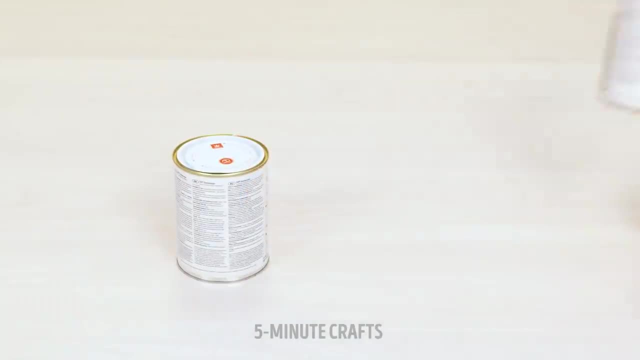 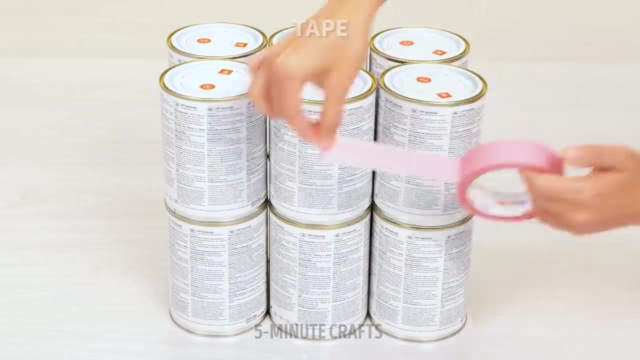 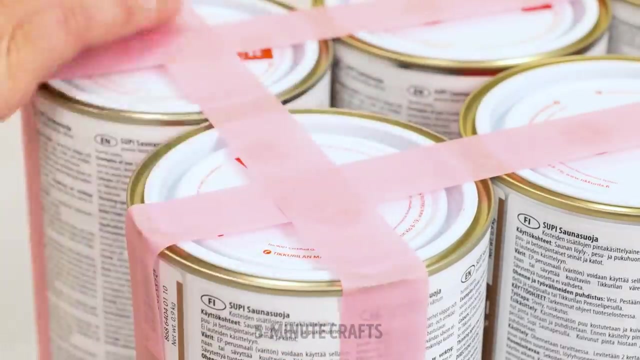 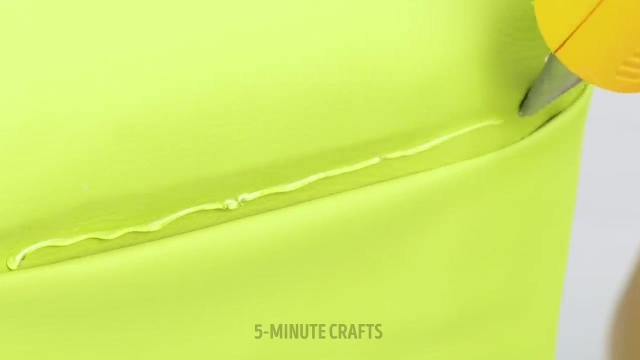 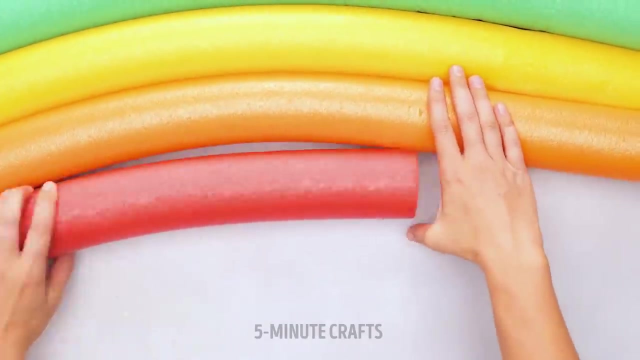 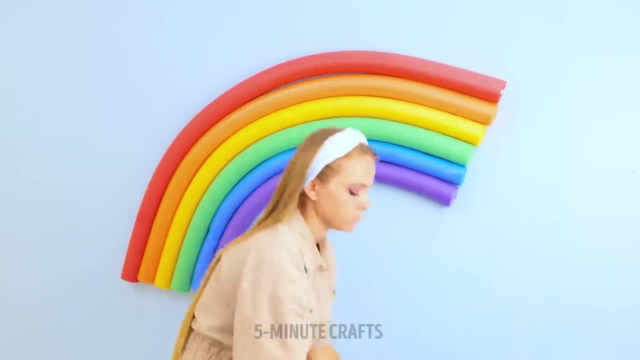 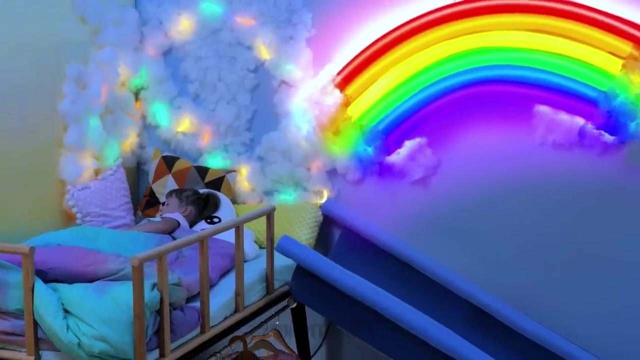 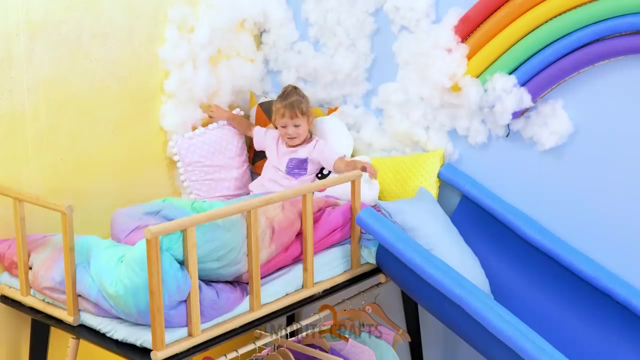 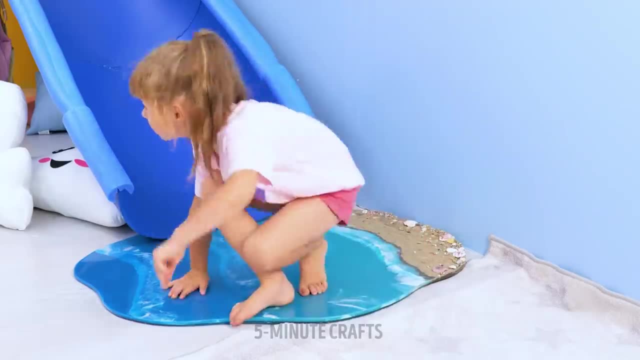 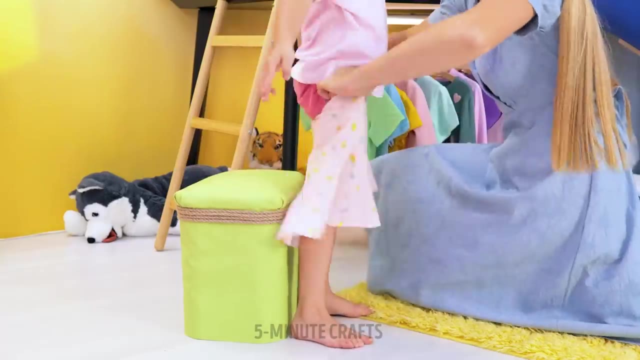 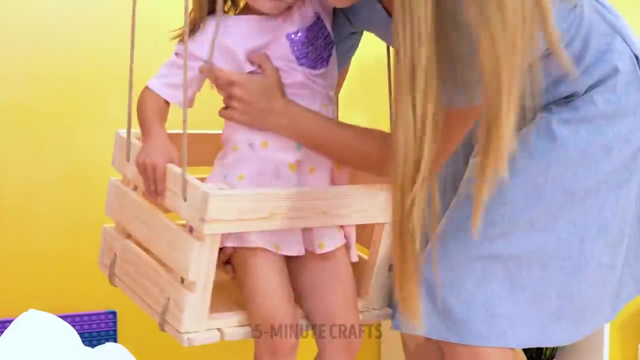 I don't wanna talk to you. I'm better off Not talking to ya, But why you Tryna hold on, To hold on, To hold on? Wanna take a different lane. Wanna play my own game And I don't need you here, So won't you? let me go. 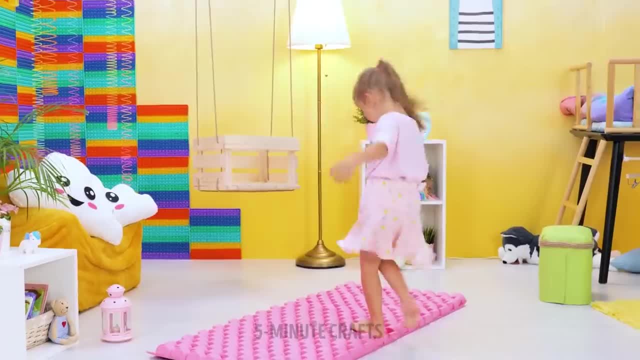 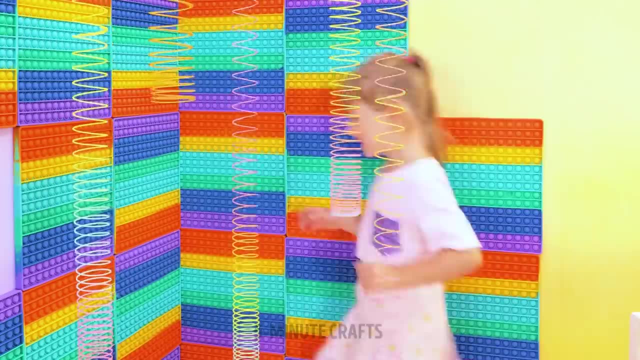 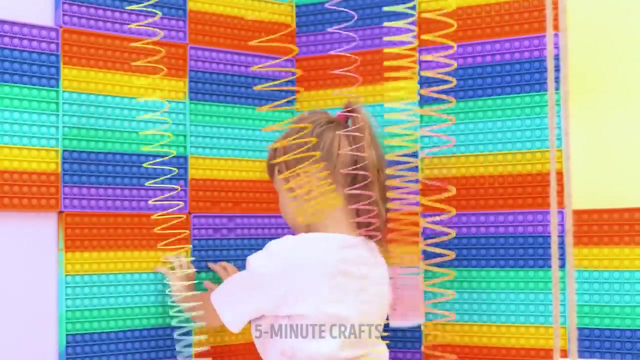 When I take this ball and chain That you have put on me And throw it out the window, I think that you should Let go, Cause you know this is not meant to be Let go. Maybe I should Tell now That you are not the right one for me. 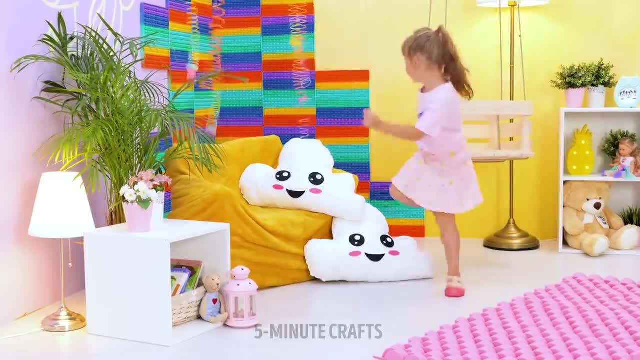 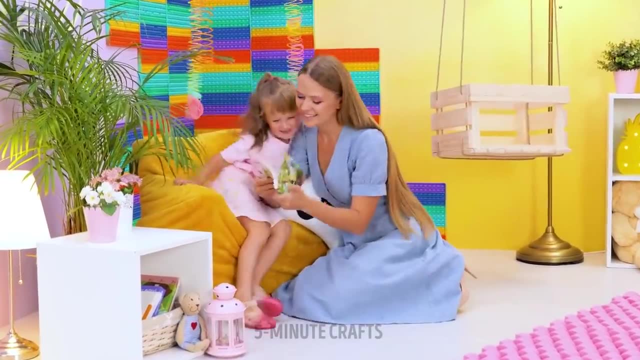 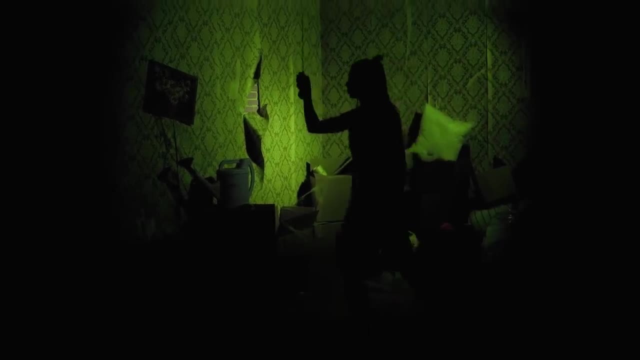 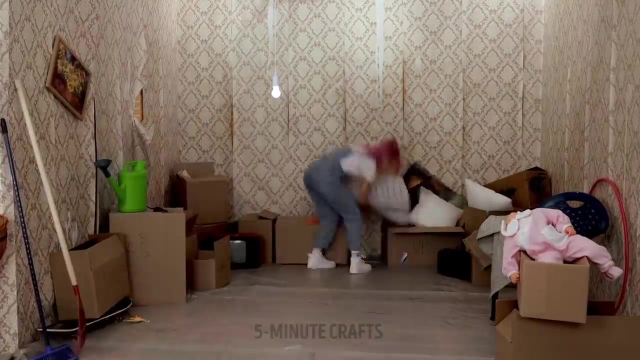 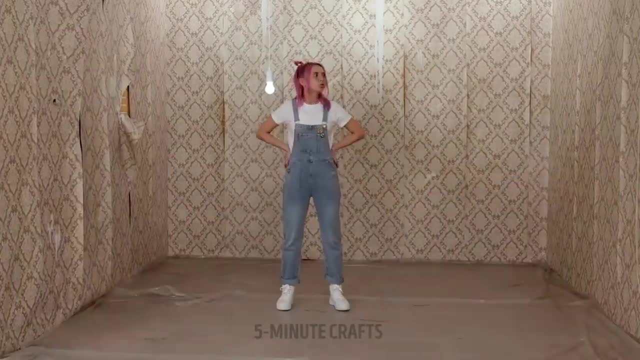 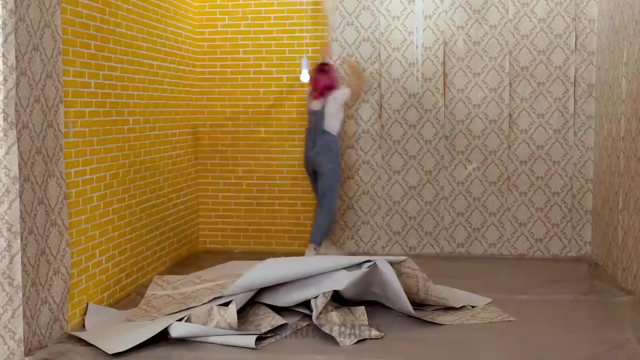 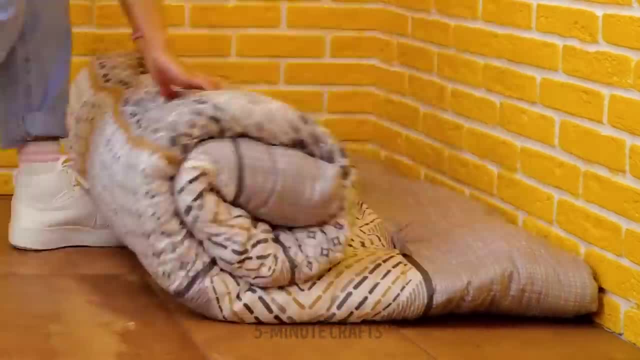 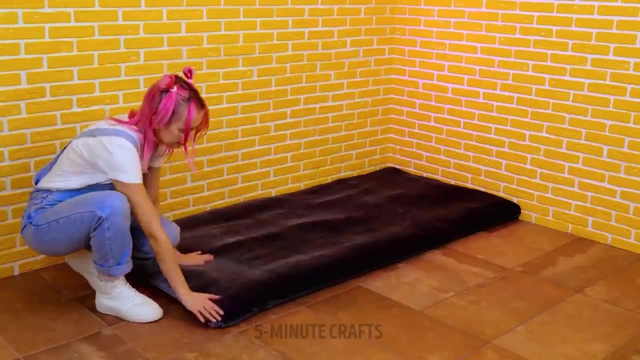 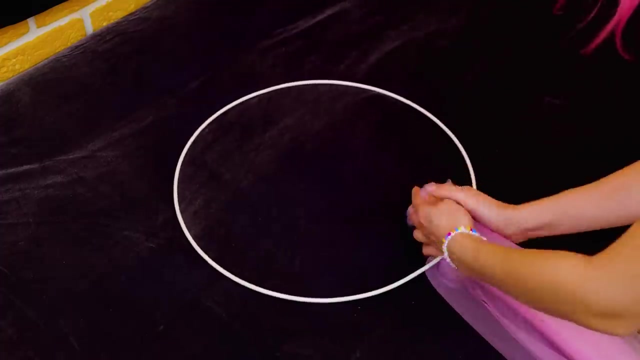 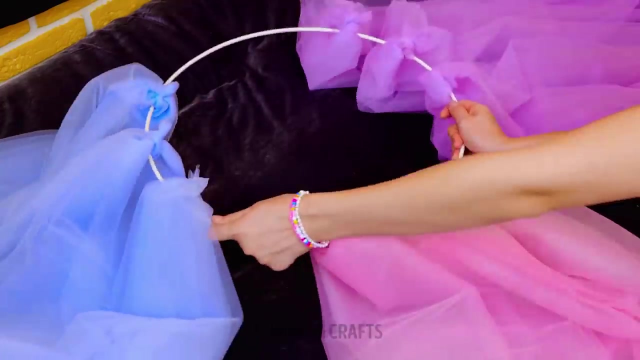 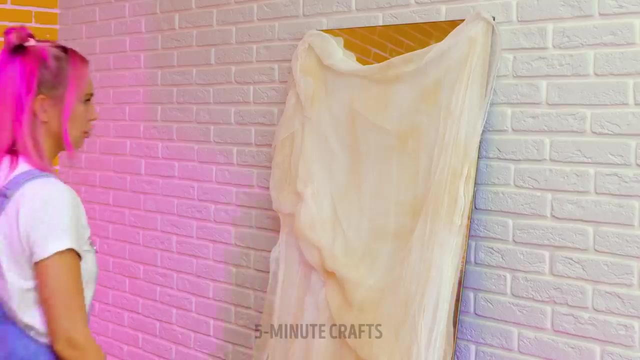 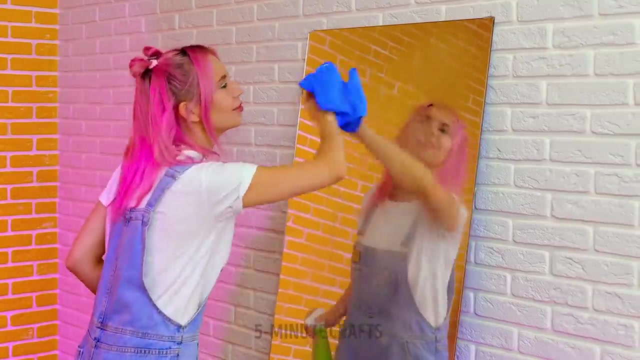 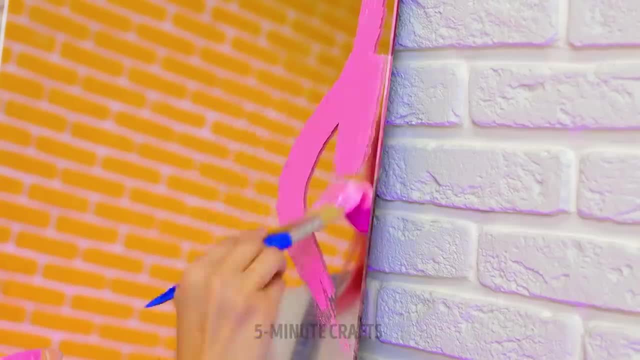 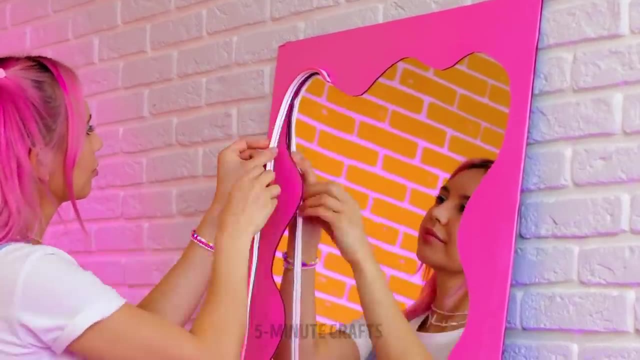 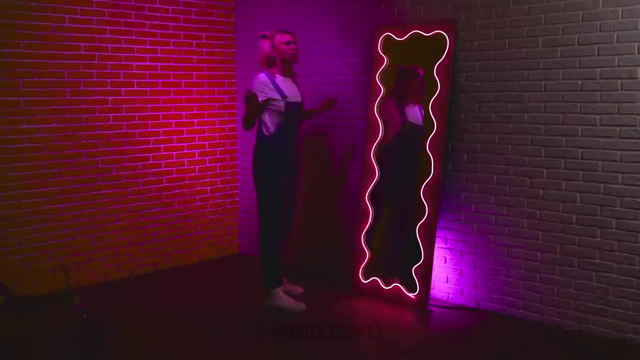 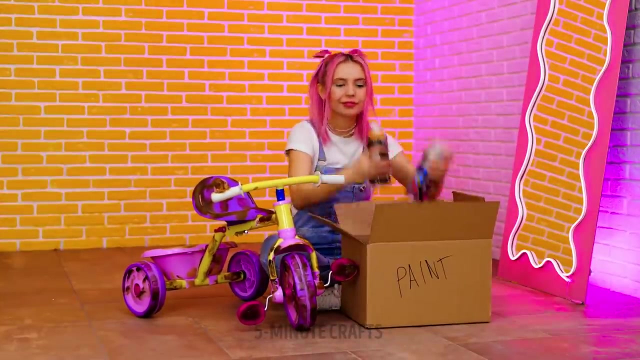 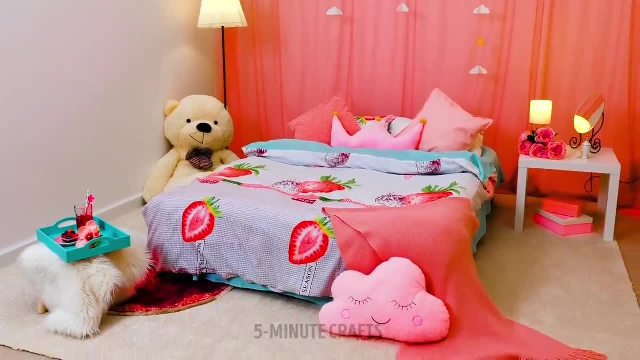 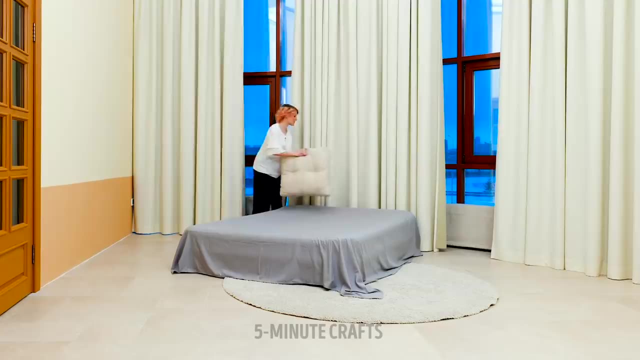 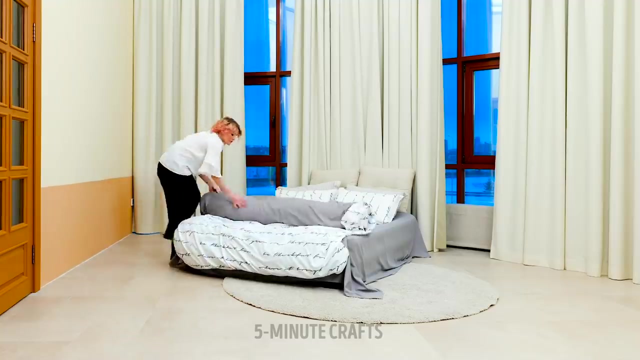 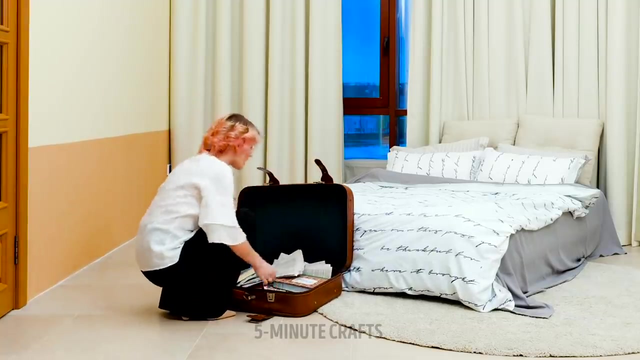 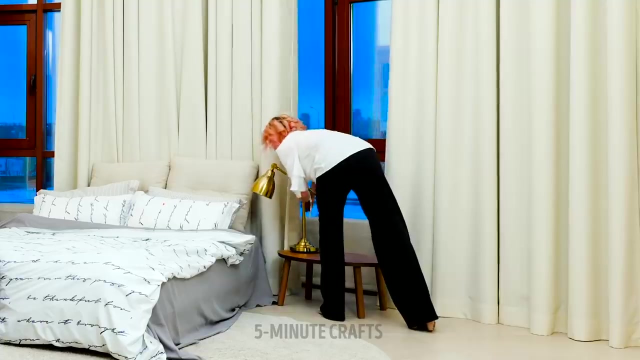 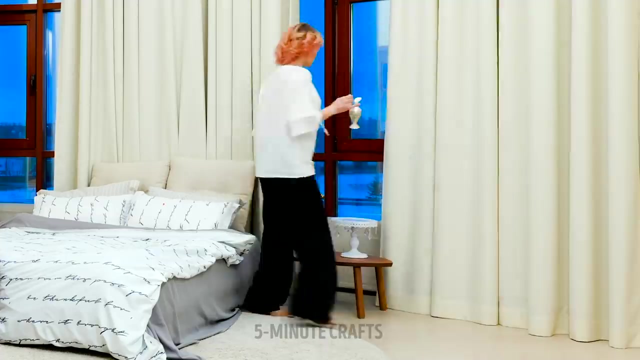 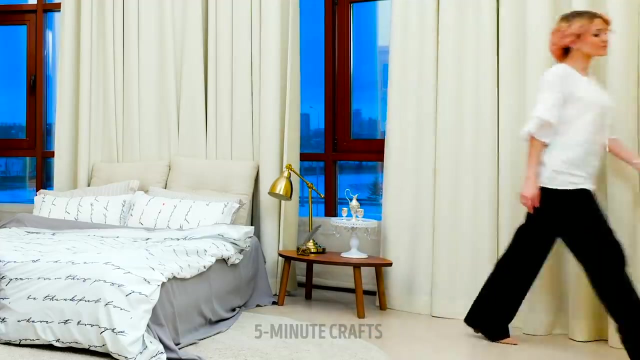 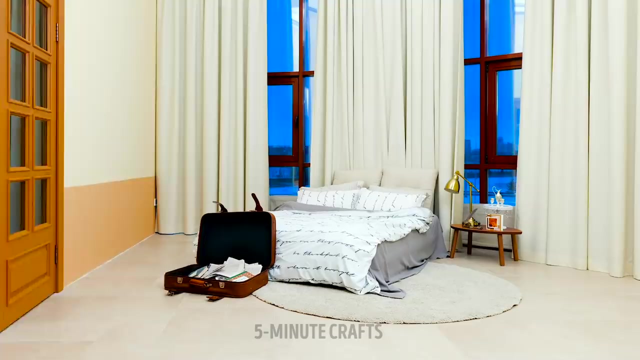 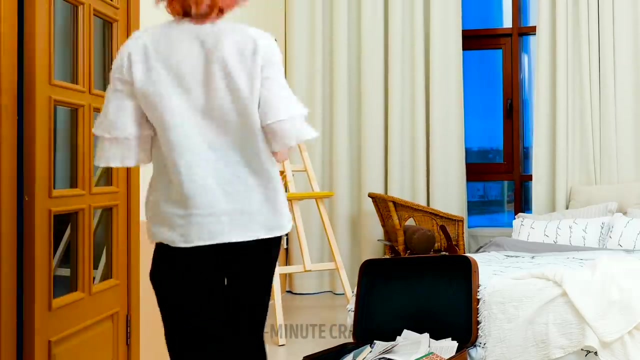 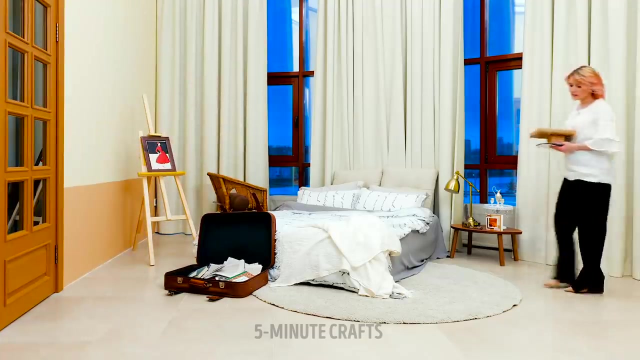 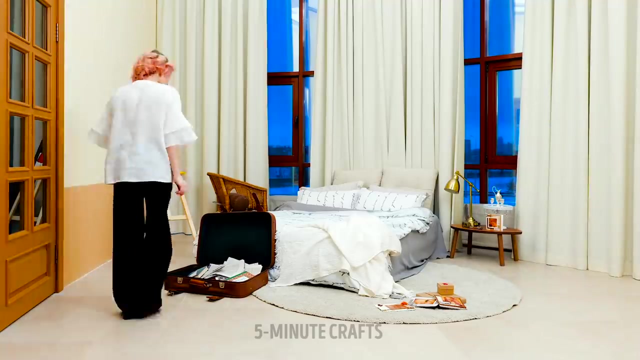 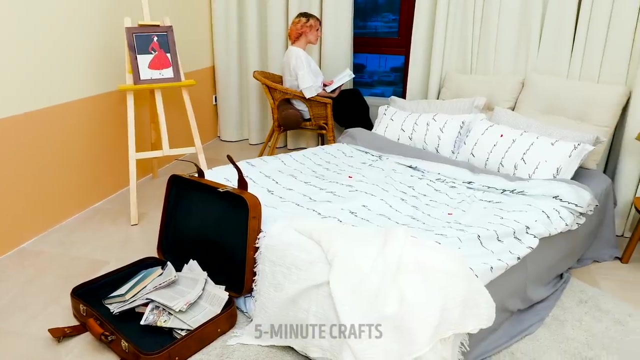 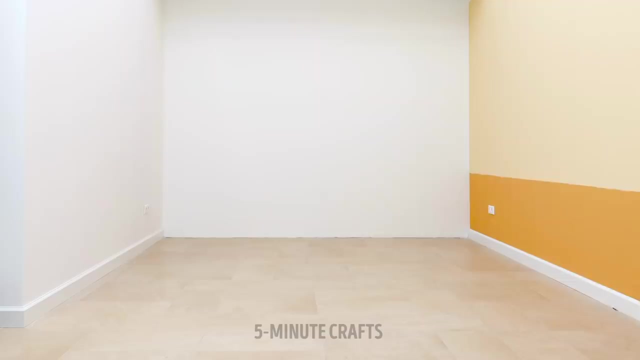 In the dark, And even if the sky was falling down, You never noticed anyone around. I don't wanna be the one to say No, I told you so, But I told you so. Keep on acting out like strangers. Scream out loud, Scream out loud: I will go if nothing changes. 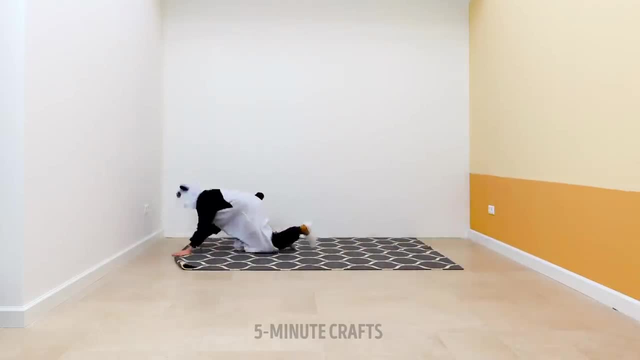 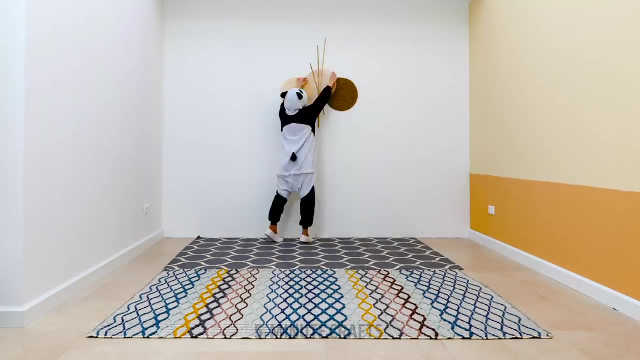 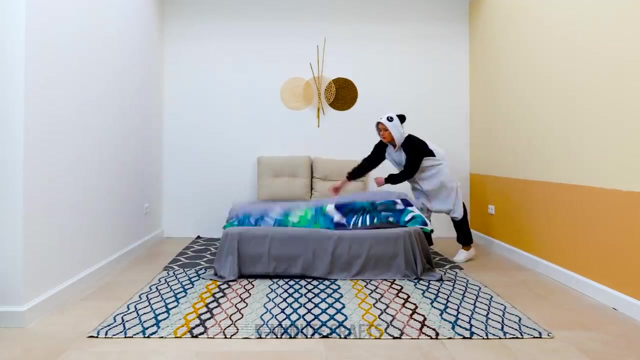 So change your heart. Ooh, your mind is a ghost town Echoing inside your walls, Five feet underground. now, Nothing's gonna save us from our doubts, Nothing's gonna make us spell it out. I don't wanna be the one to say No, I told you so. 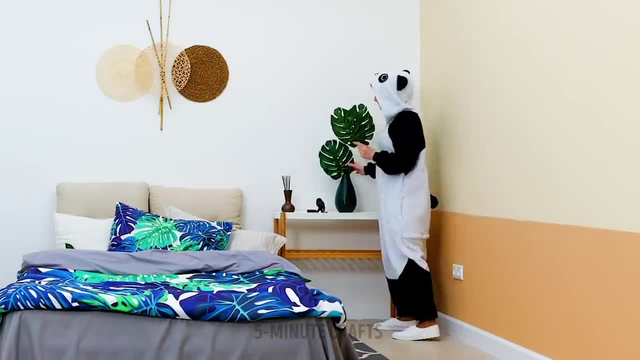 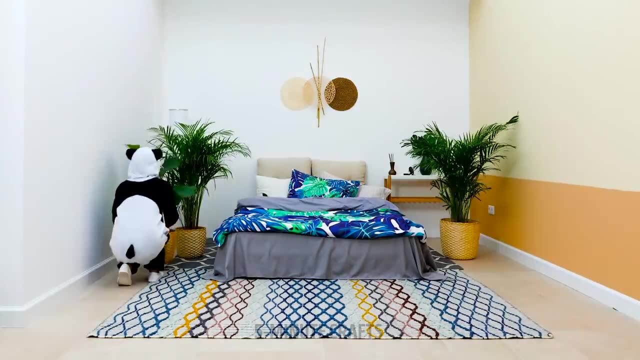 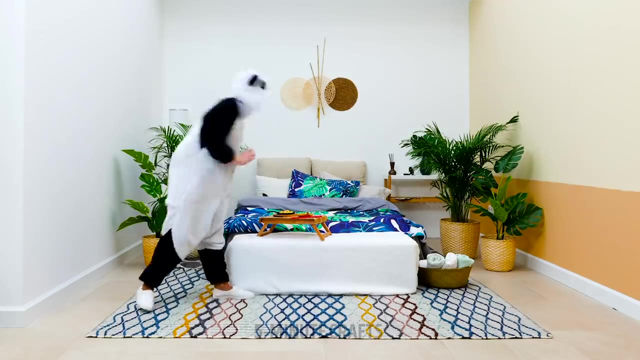 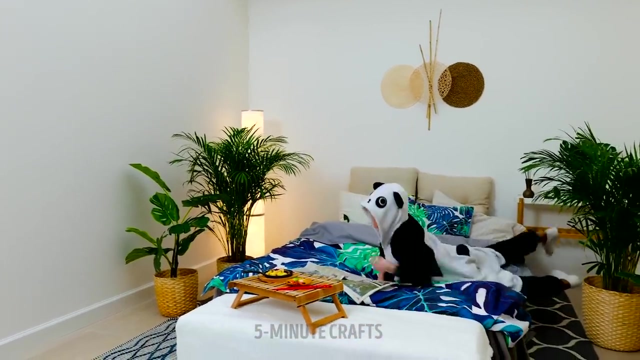 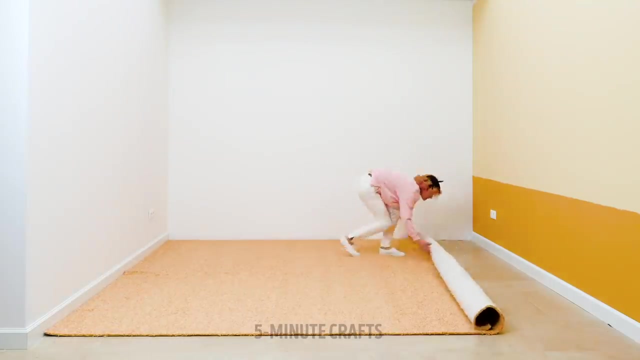 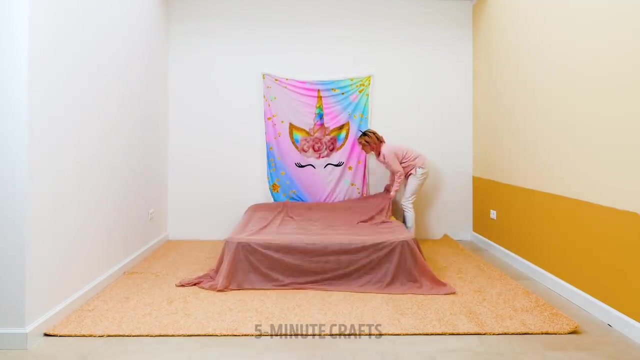 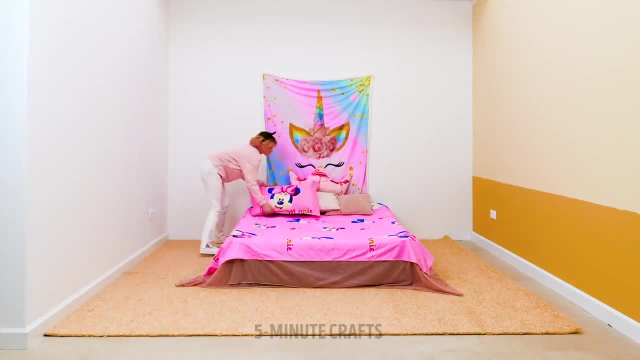 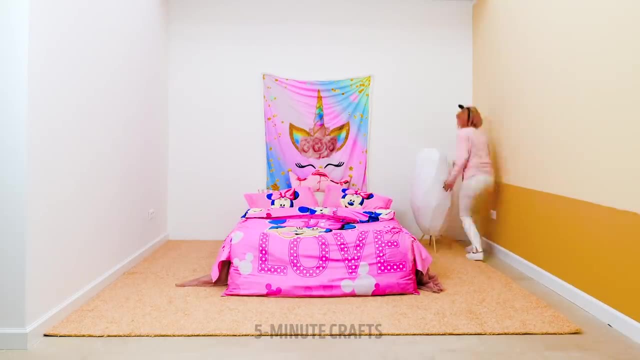 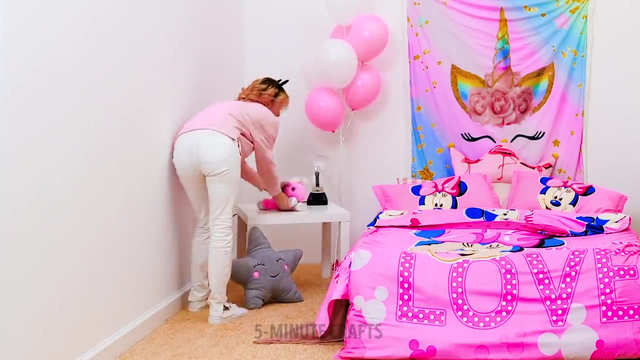 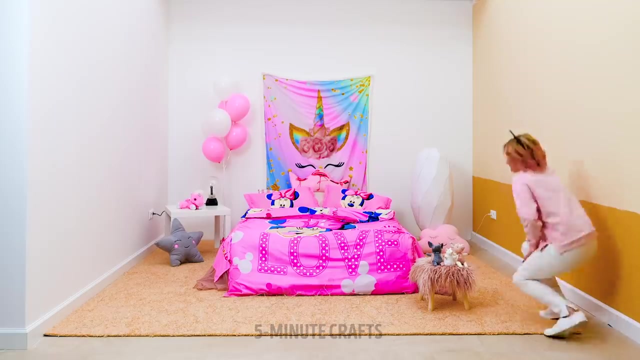 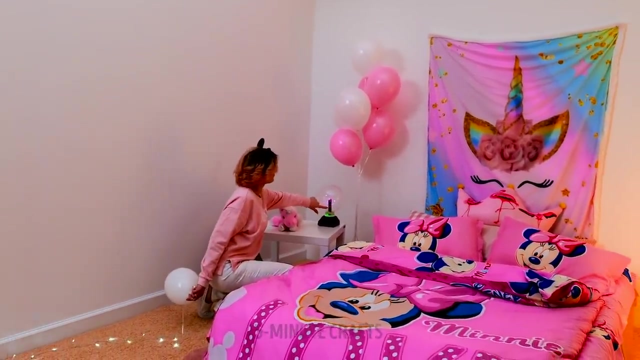 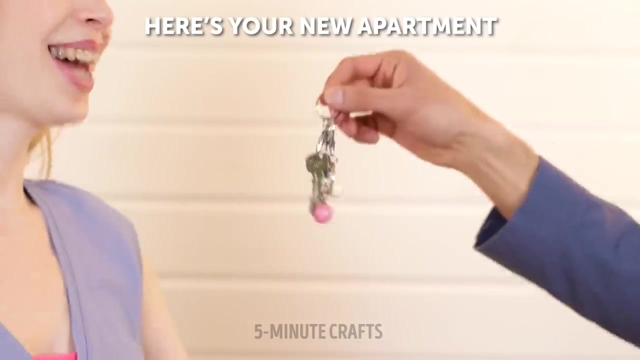 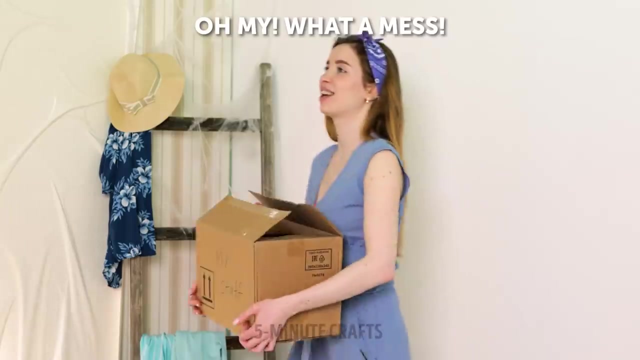 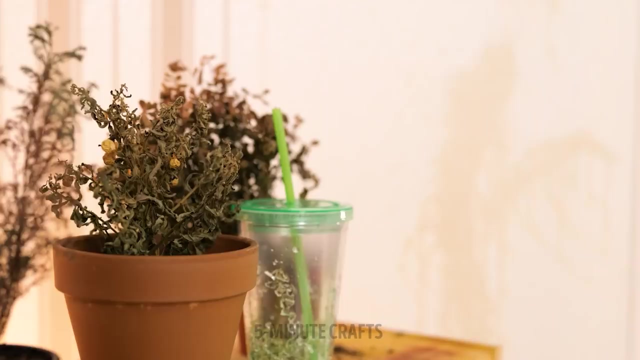 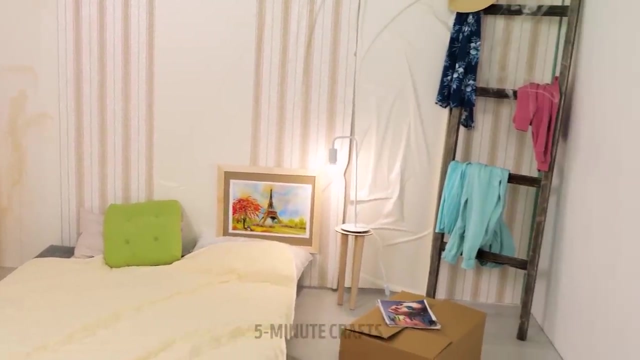 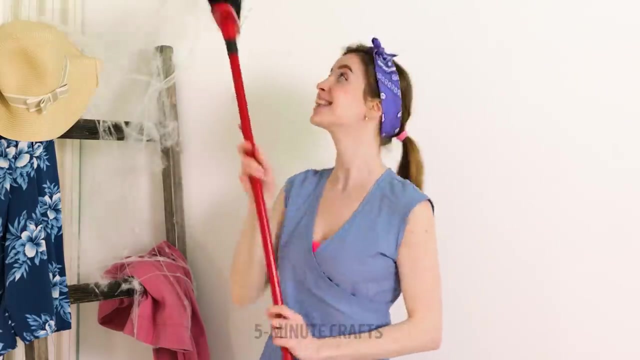 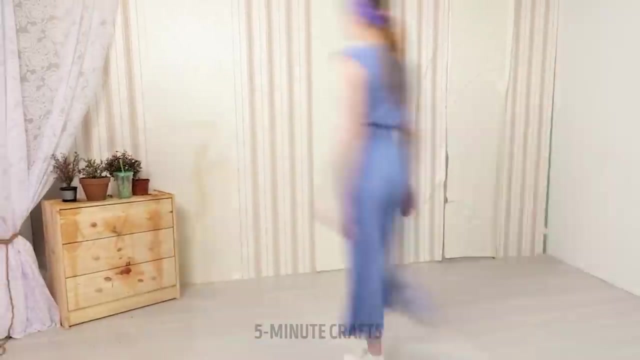 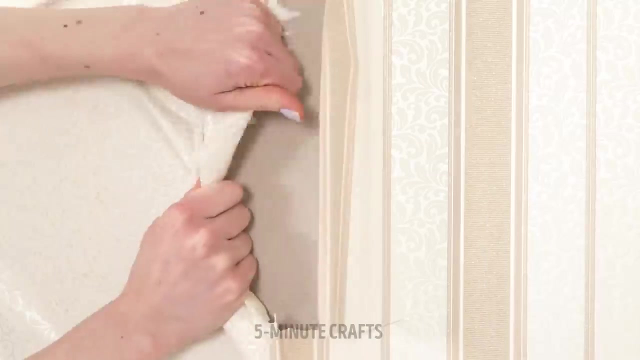 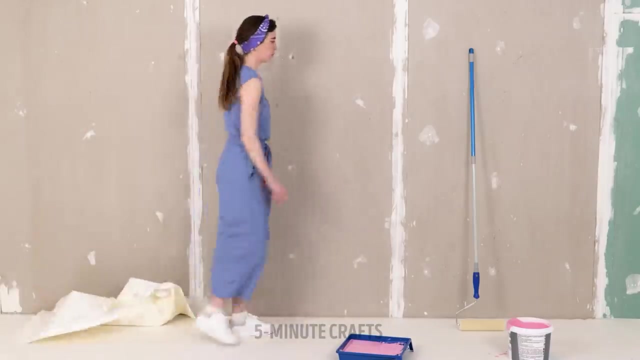 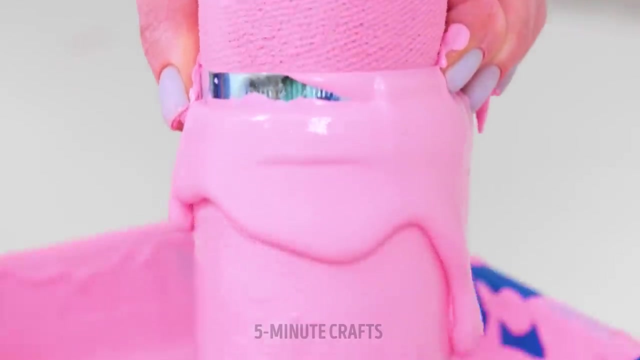 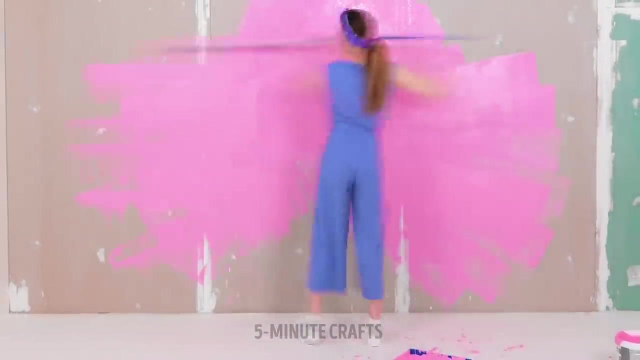 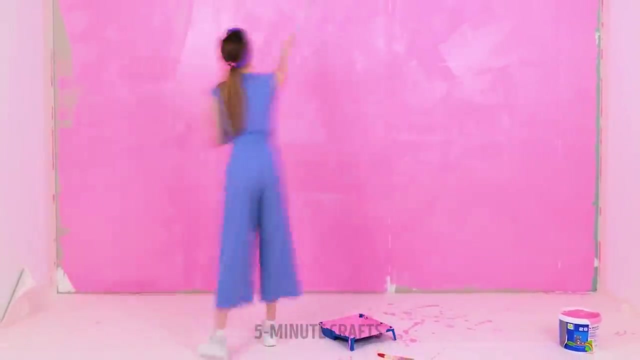 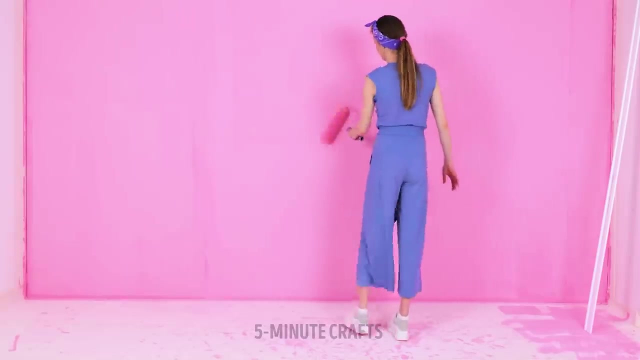 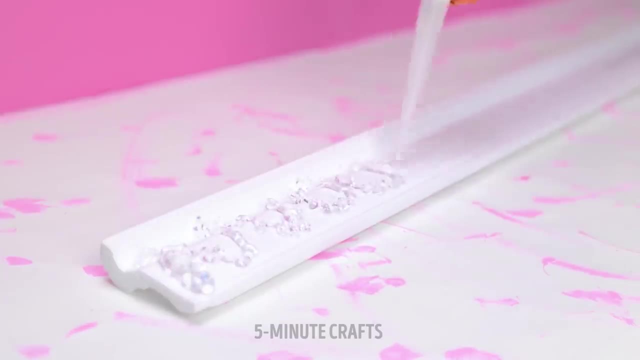 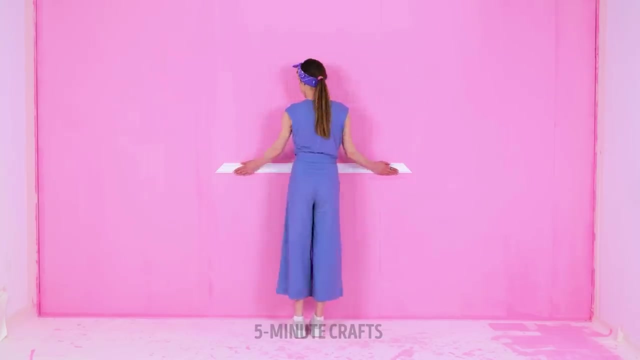 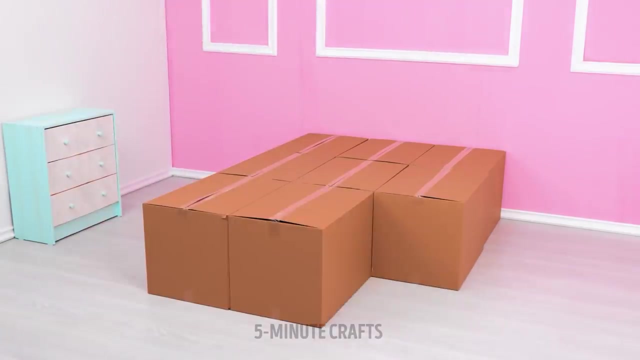 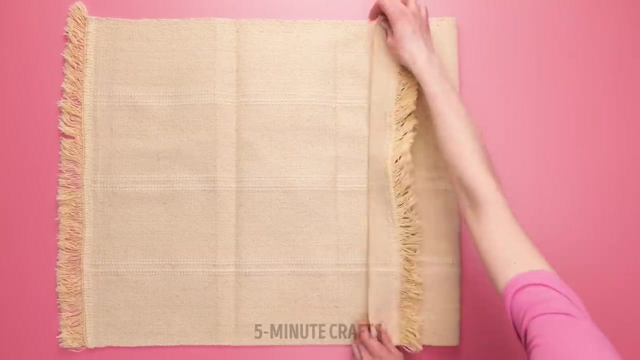 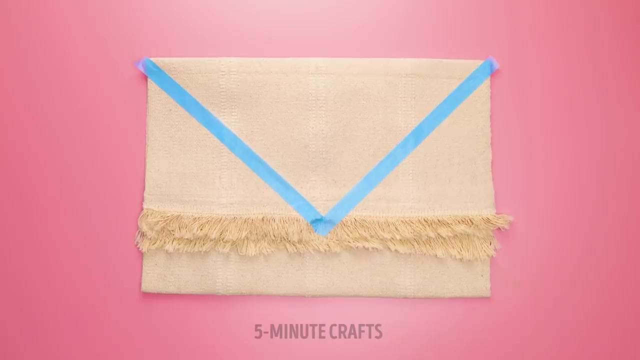 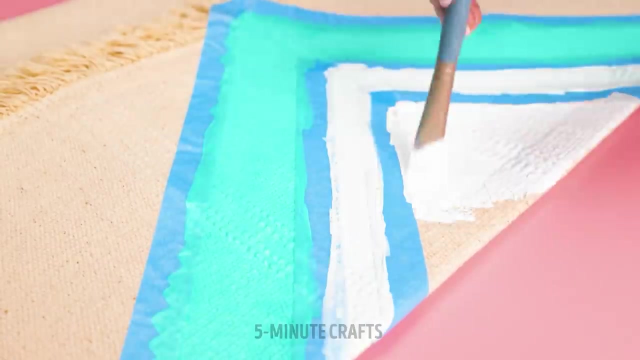 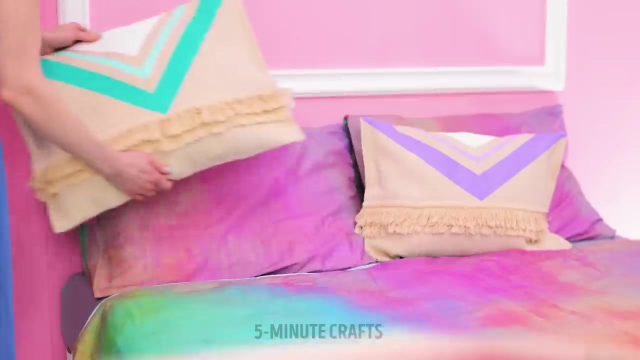 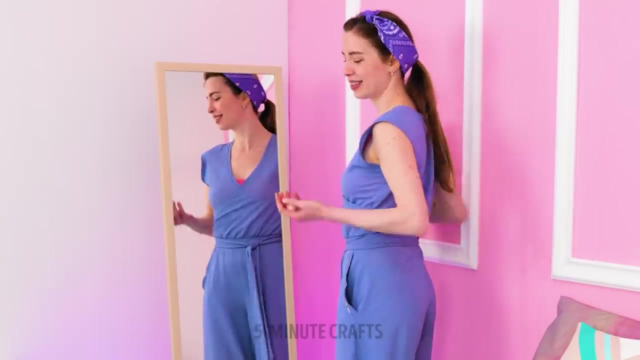 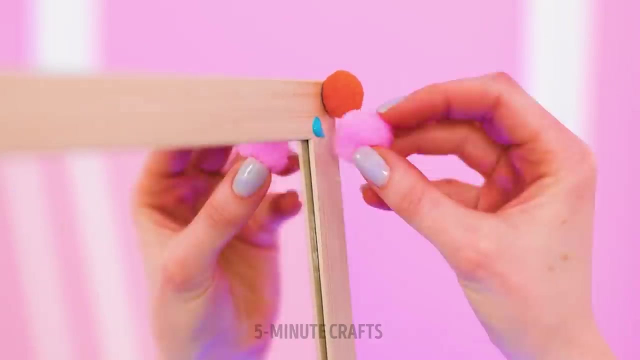 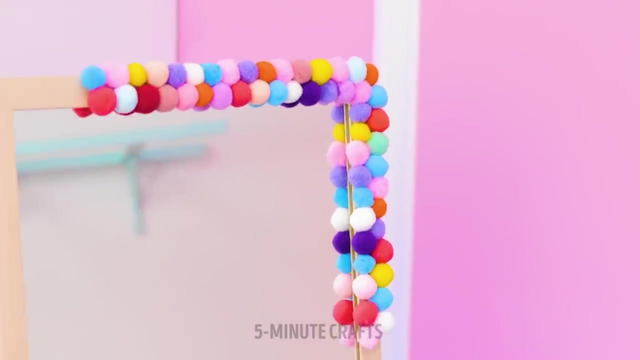 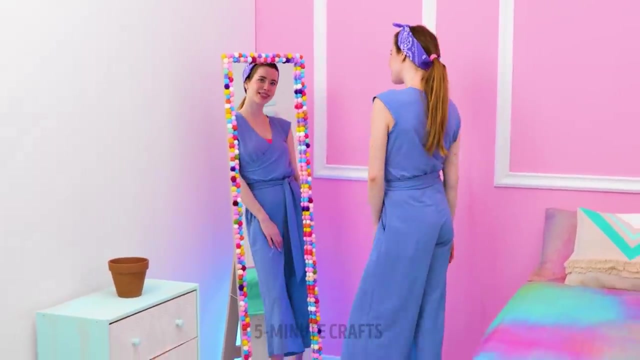 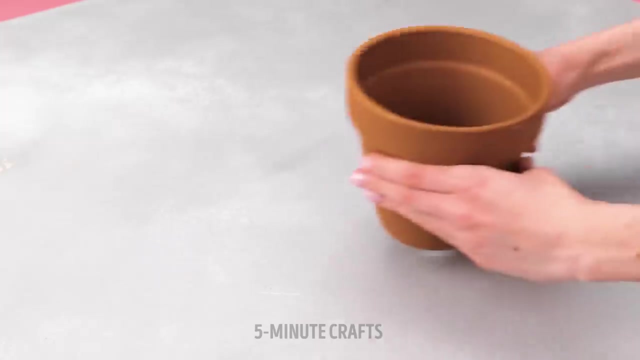 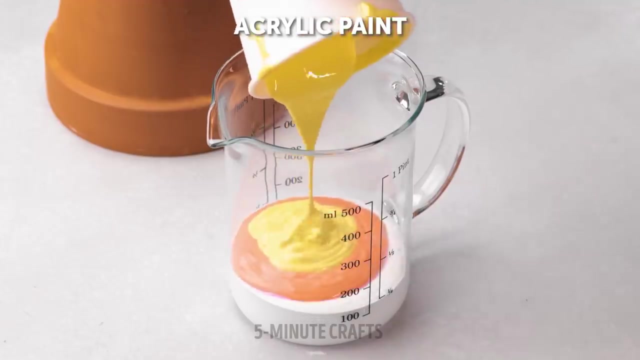 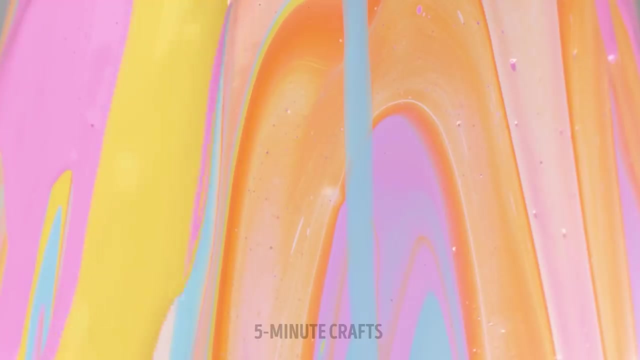 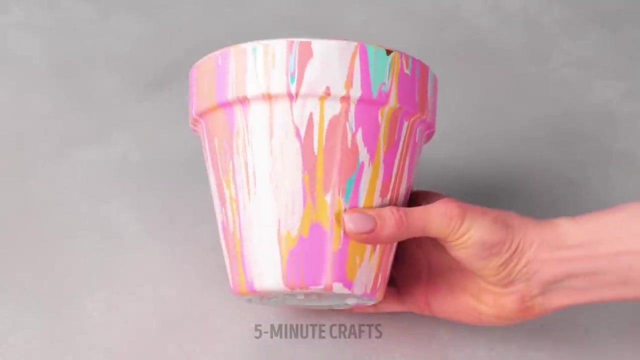 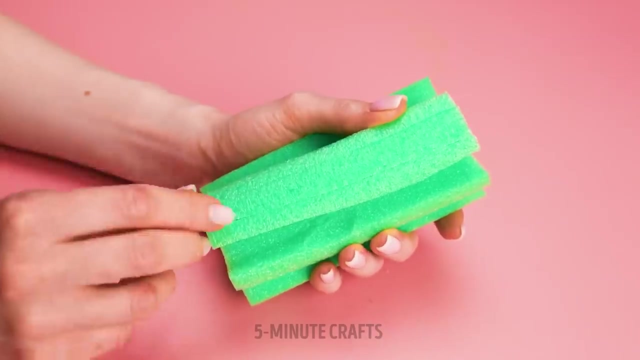 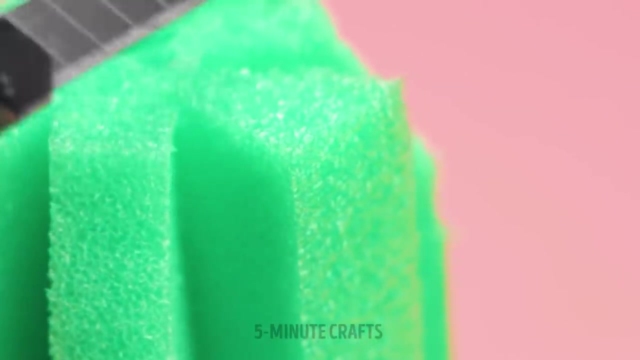 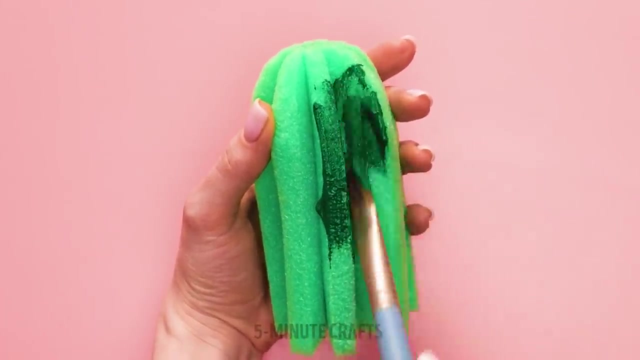 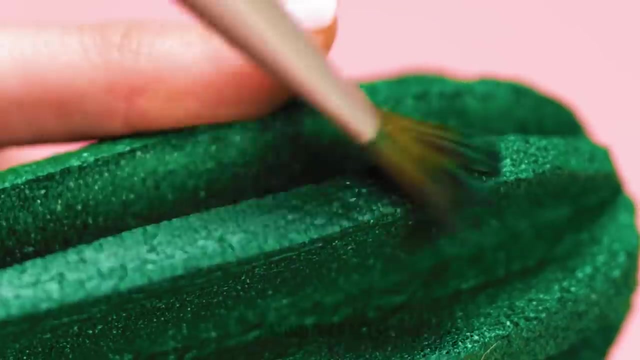 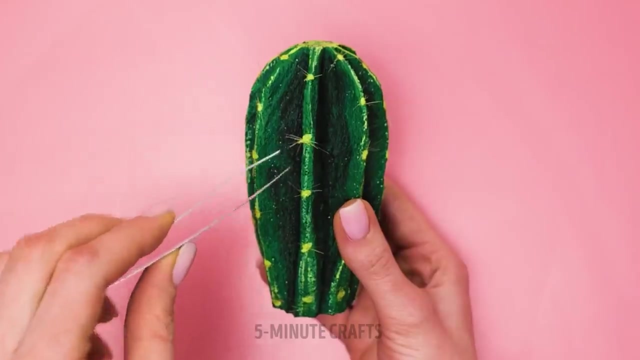 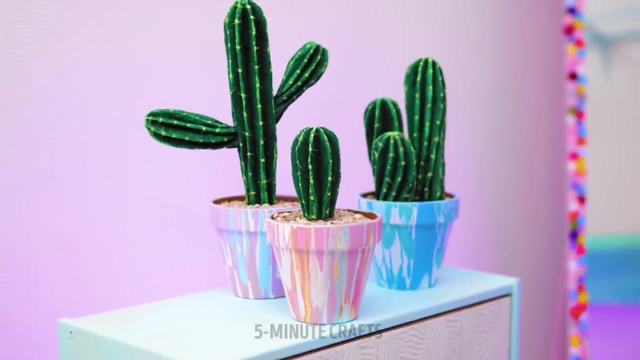 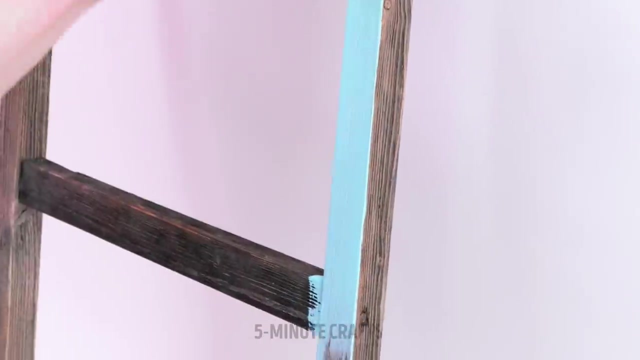 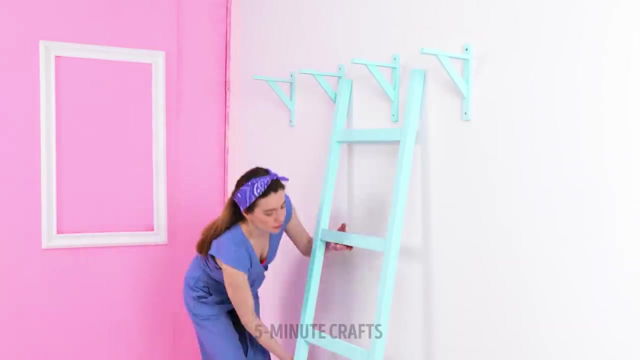 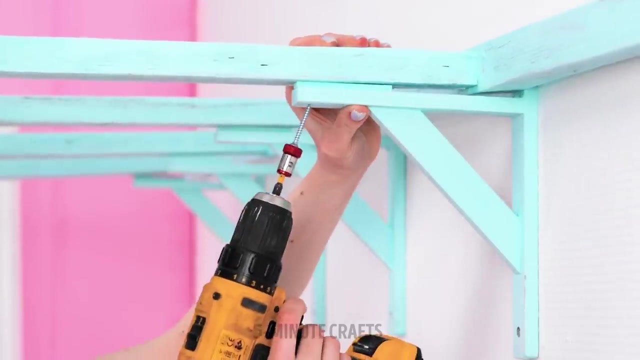 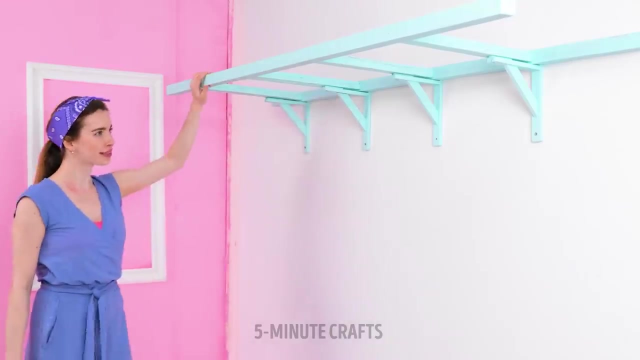 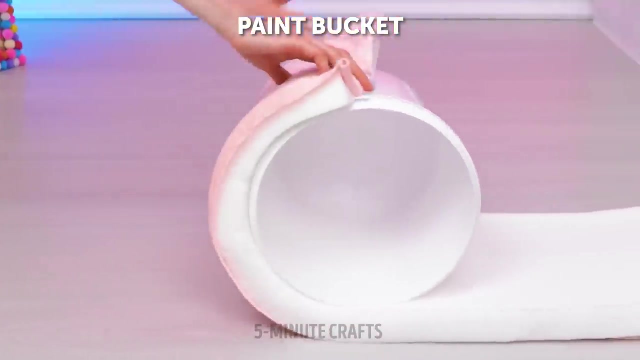 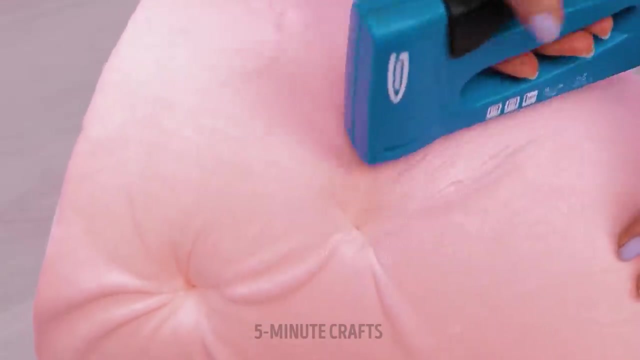 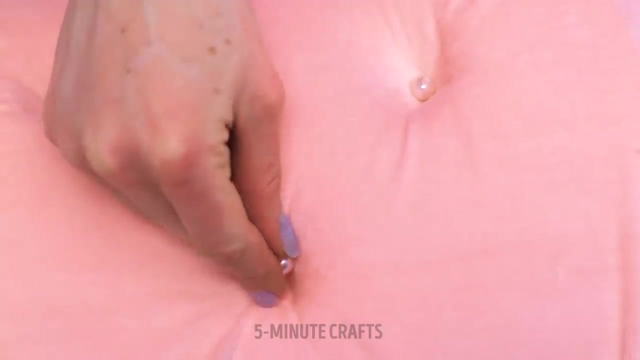 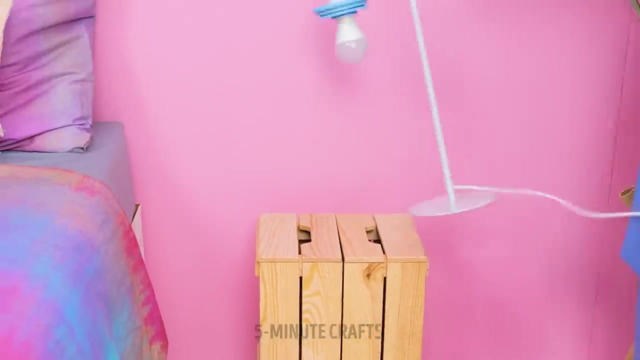 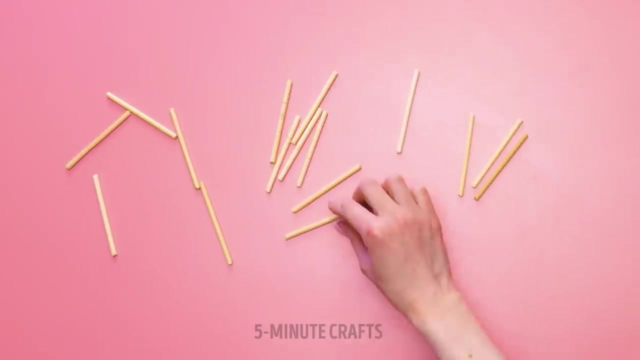 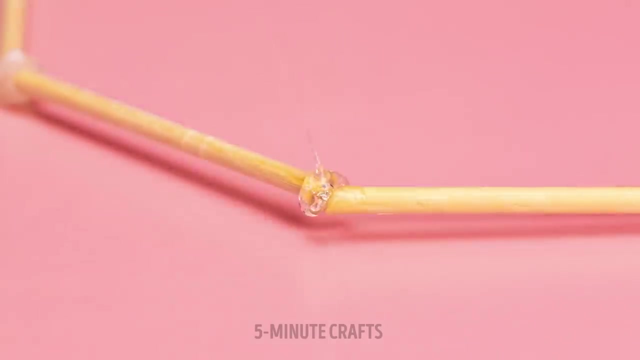 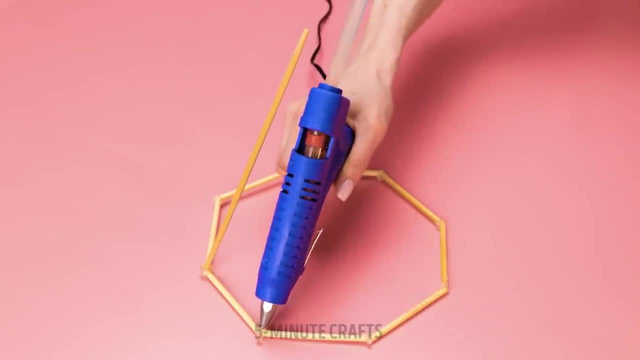 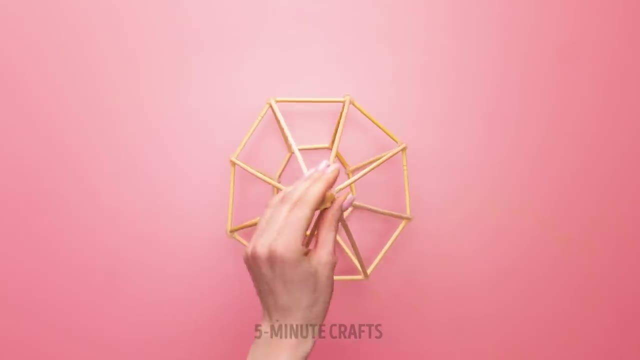 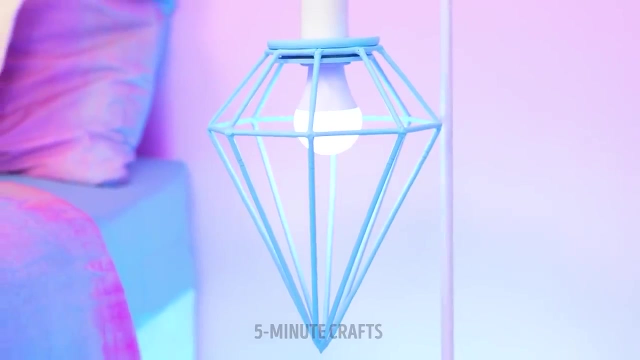 But then I turn around and let it go. I see you watching me from a distance. I see you can't decide what to feel. But if you dig a little deeper, boy, You know you really wanna get to know me. Let's get this over with. Wait, I can't wait another day. 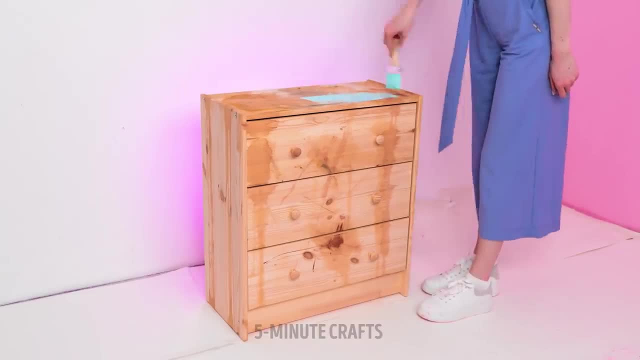 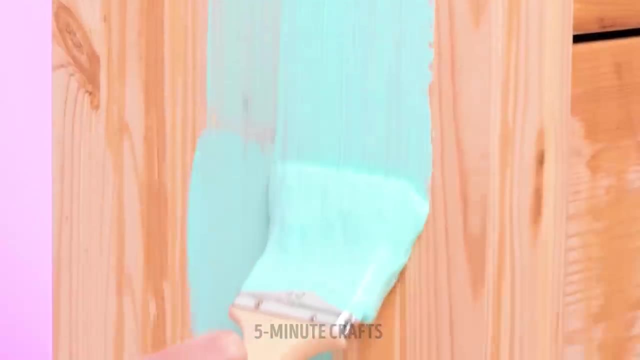 To tell you you shouldn't wait. Don't be so afraid. Yeah, I'm a bit too much, but I'm fun and games. When I'm at the top, I just wanna play. If you are looking for one hell of a ride, Just come and get it, baby, I'm all yours. 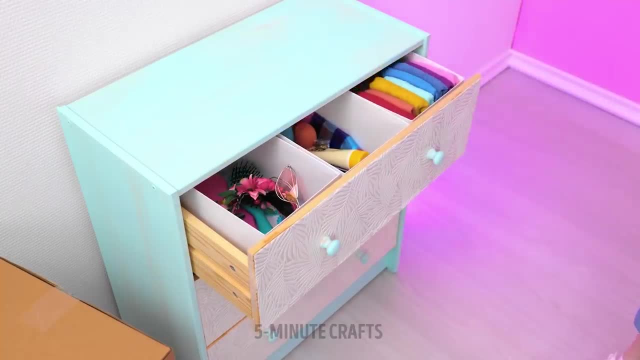 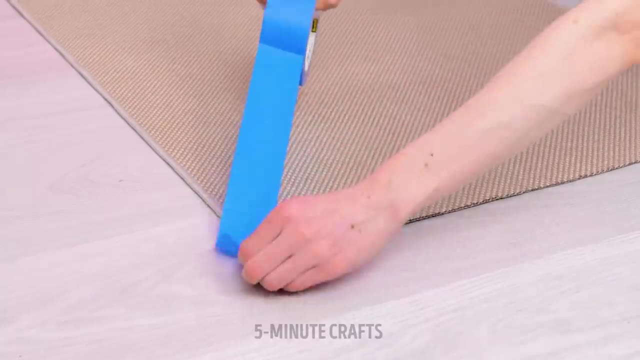 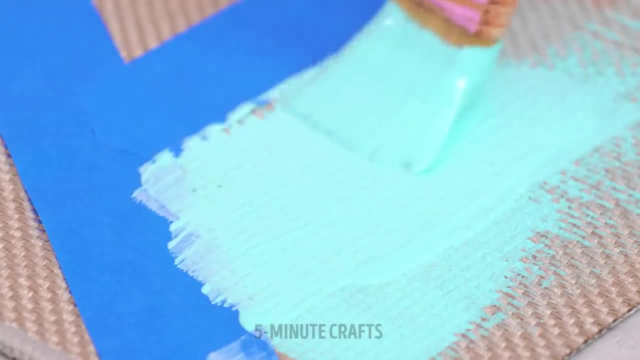 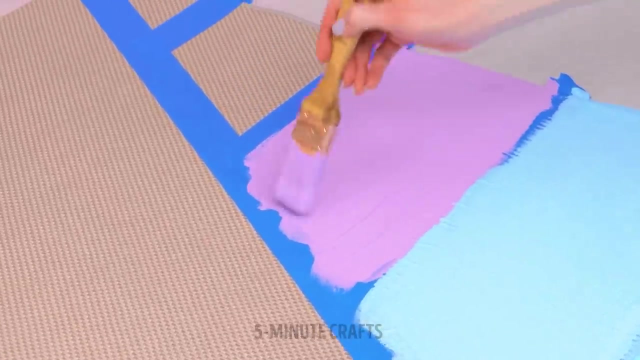 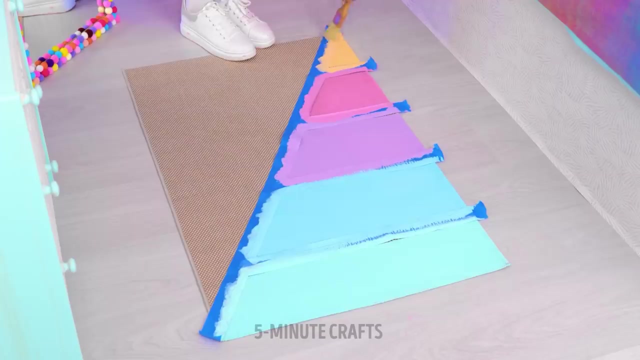 It won't be easy, but it'll be fun. Sometimes it goes the whole way up and down. I think you're ready now to leave the ground. Get in the fast lane. babe, you can make it. I promise I'll be there all the way And if you get a little broken down, 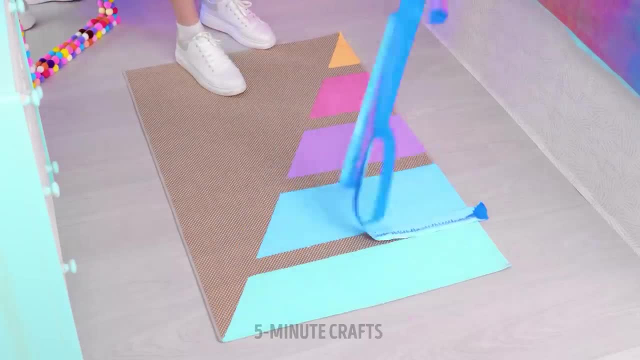 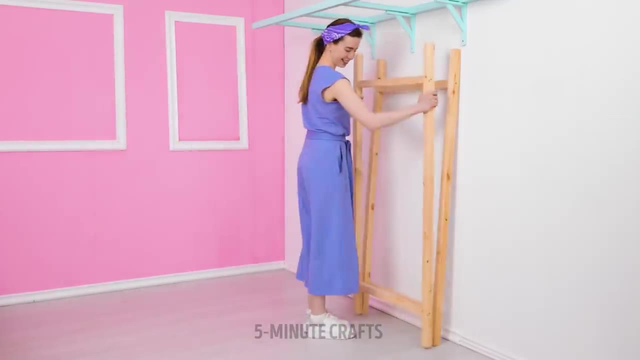 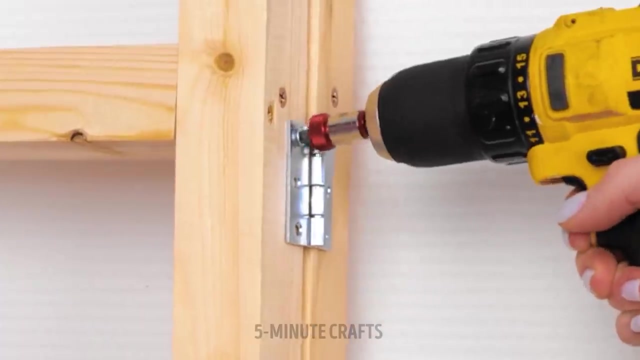 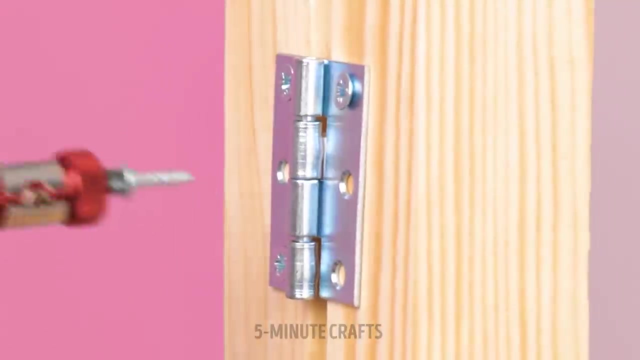 I'll let you go. just keep your head high. Let's get this over with. Yeah, I'm a bit too much, but I'm fun and games When I'm at the top. I just wanna play If you are looking for one hell of a ride. 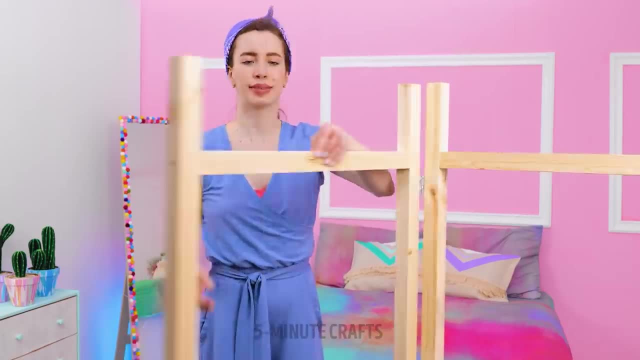 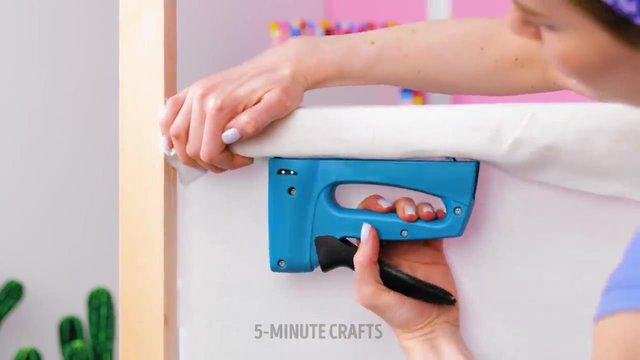 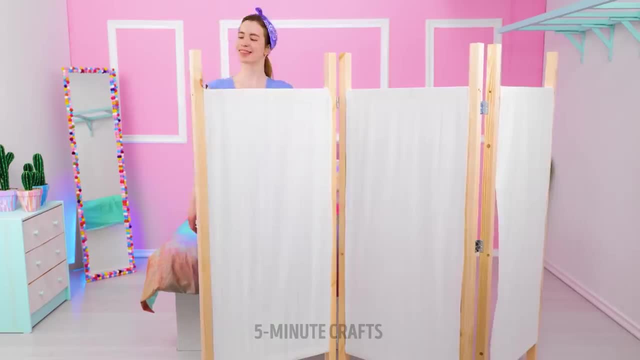 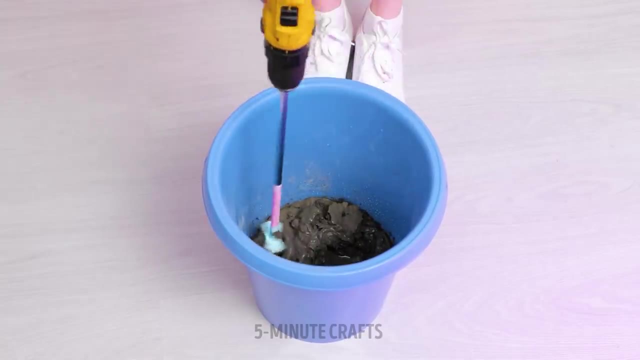 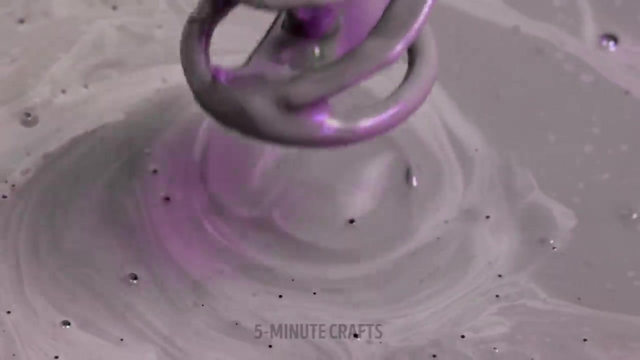 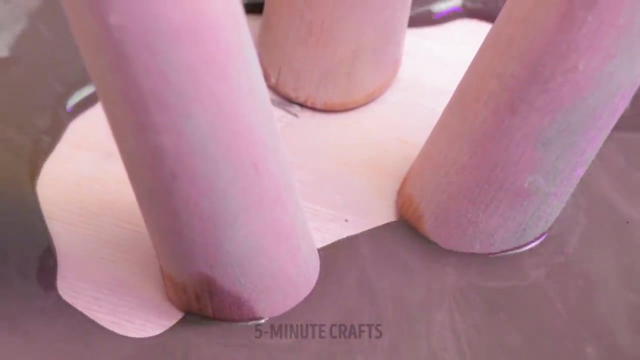 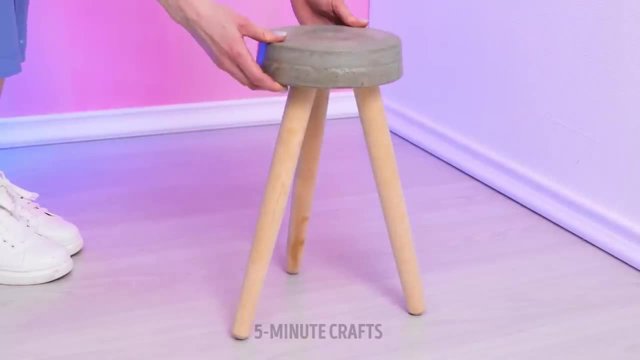 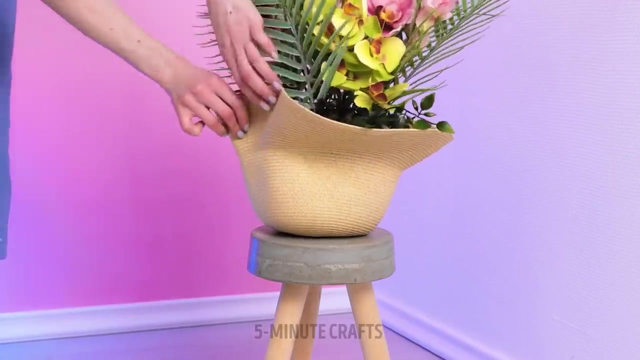 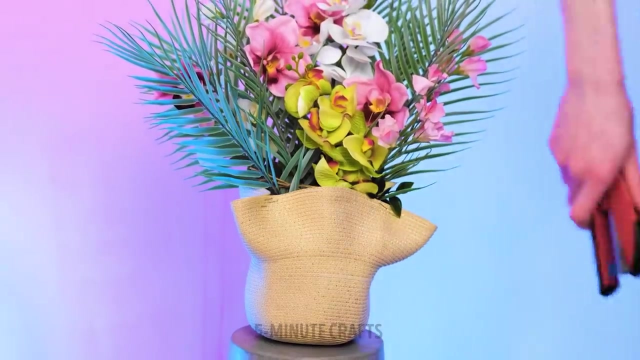 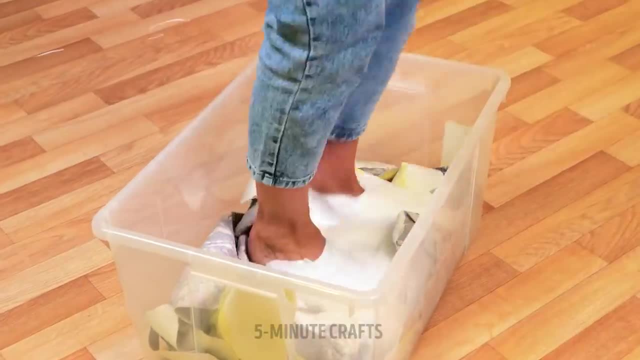 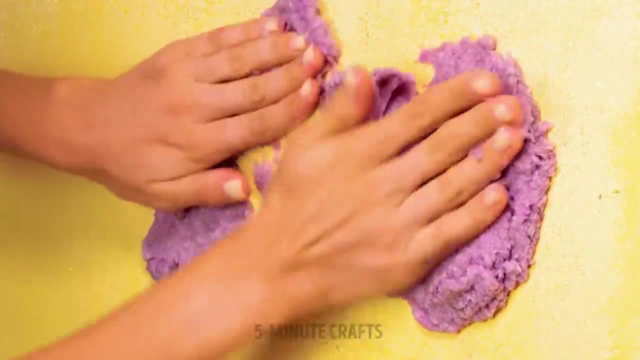 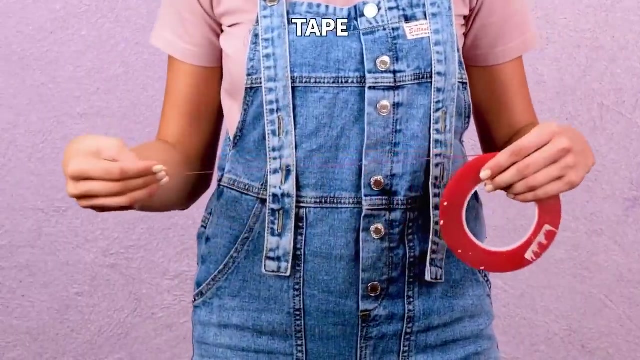 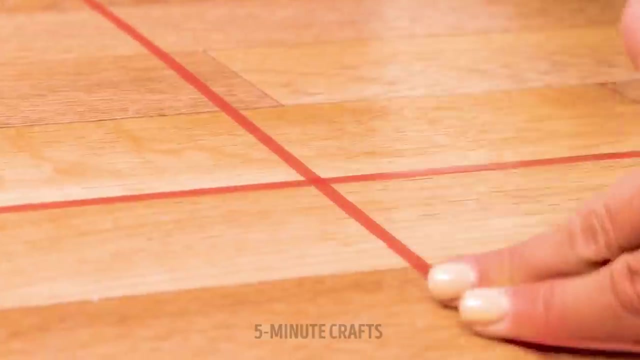 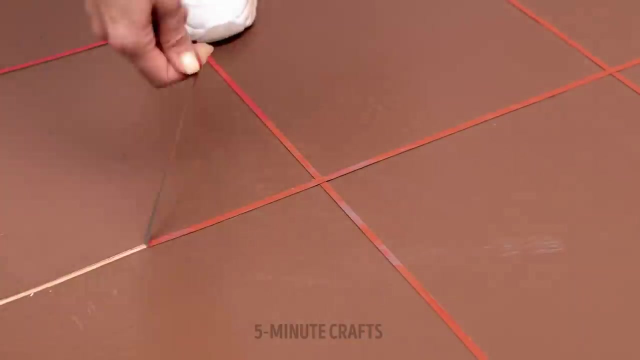 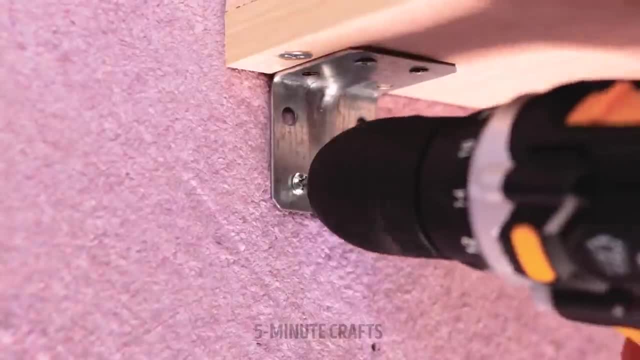 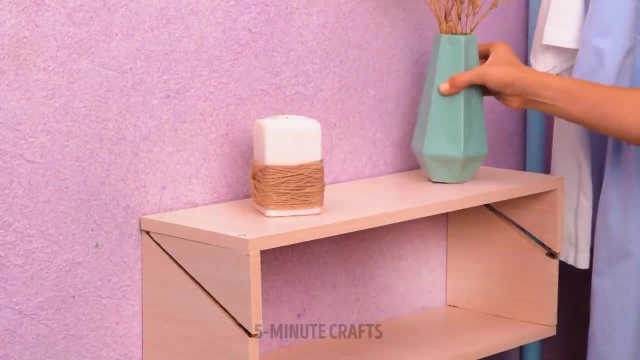 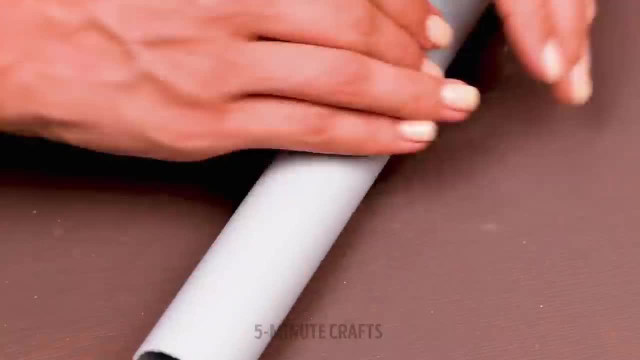 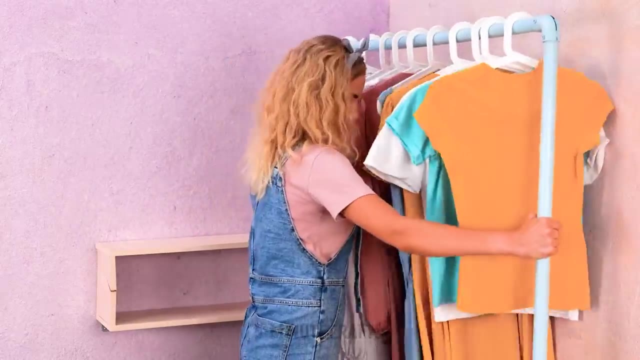 Just come and get it, baby, I'm all yours. Just come and get it, baby, I'm all yours, And I don't need you here. so won't you let me go When I take this ball and chain that you have put on me? 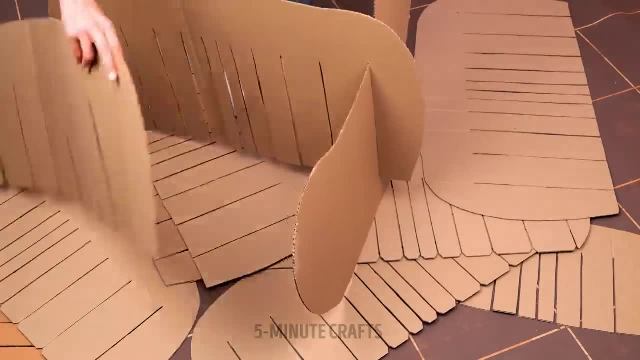 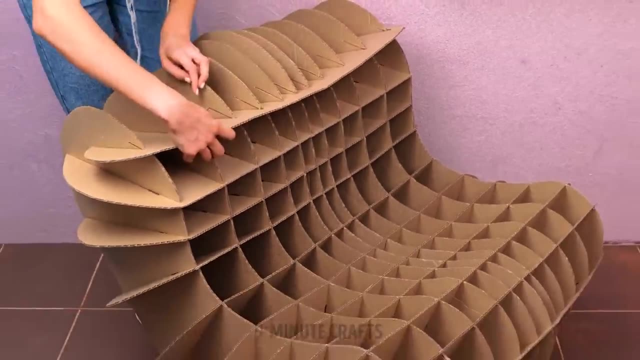 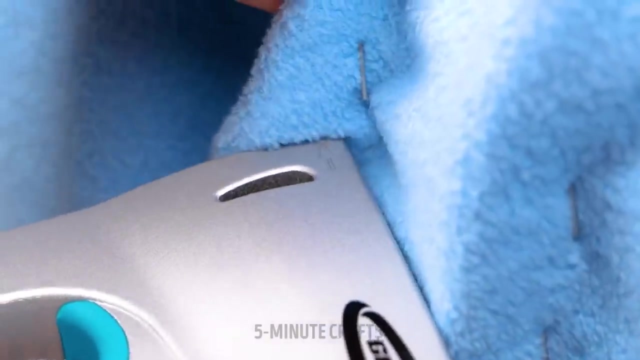 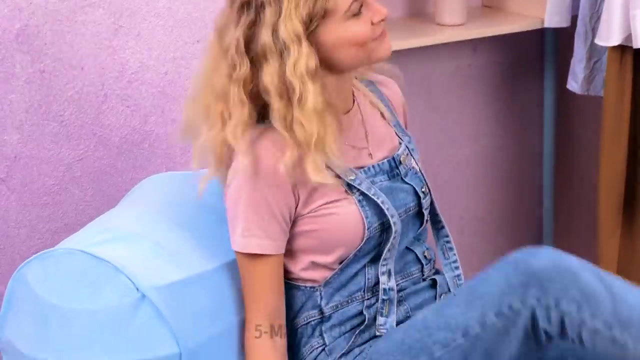 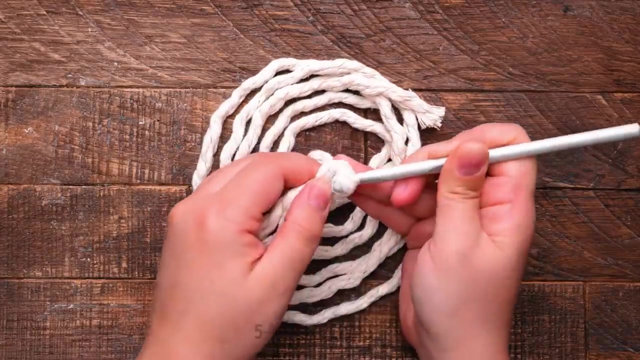 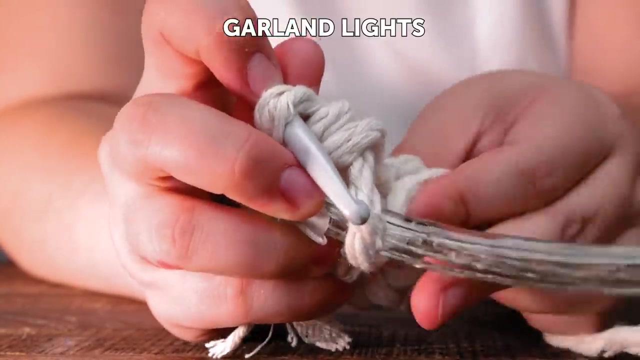 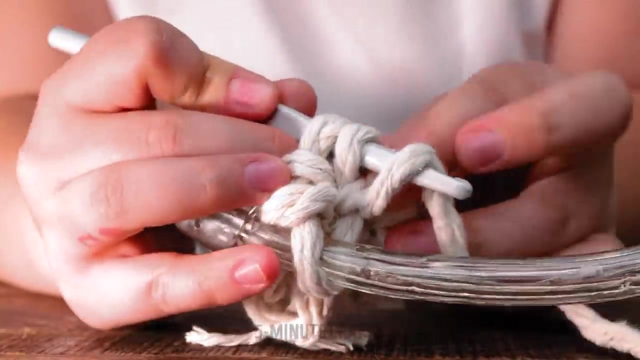 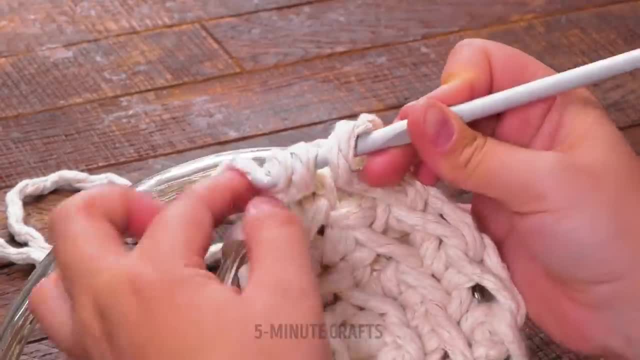 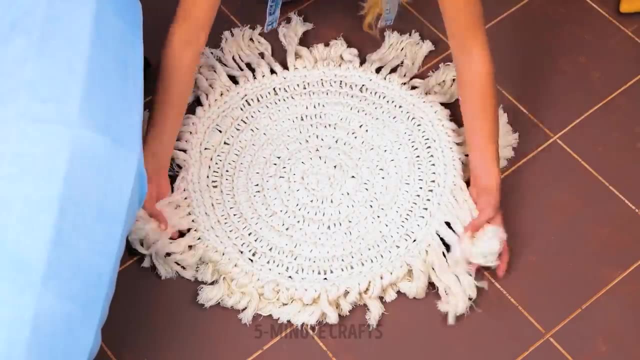 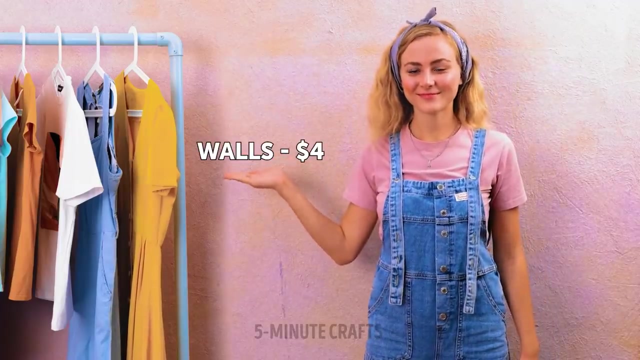 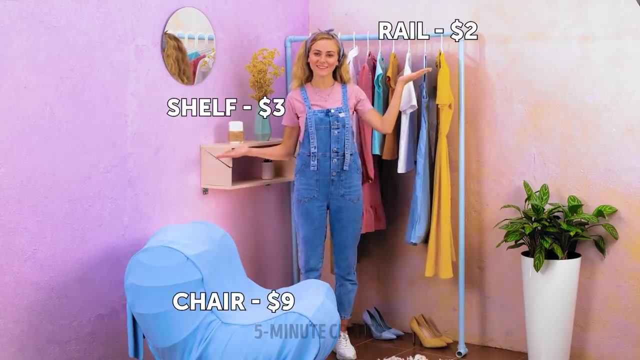 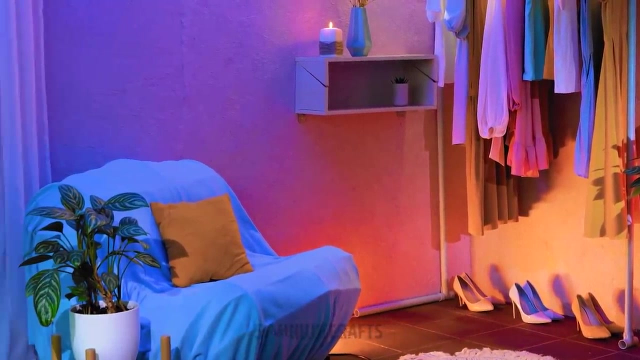 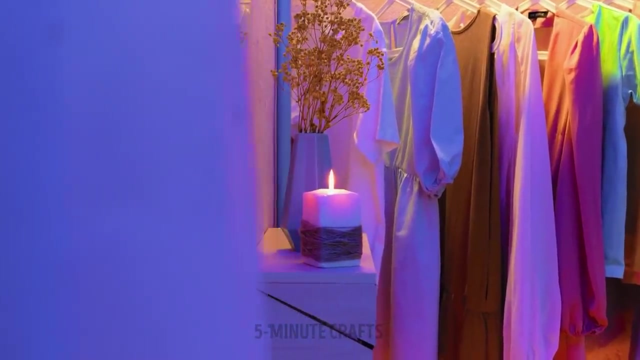 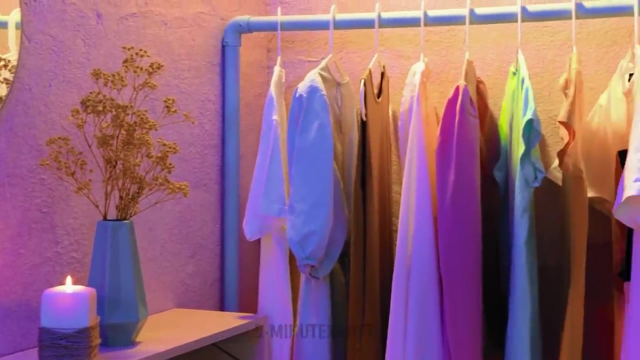 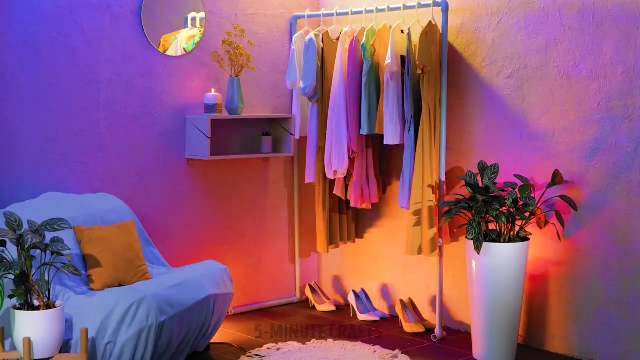 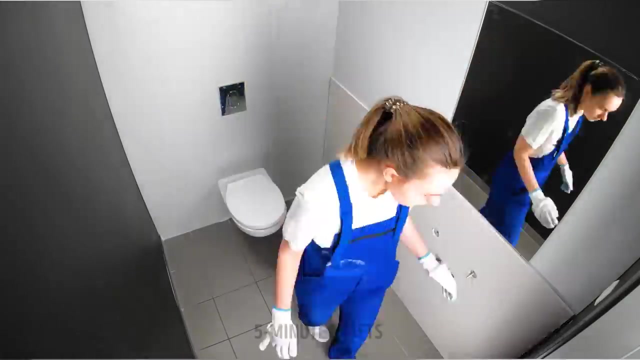 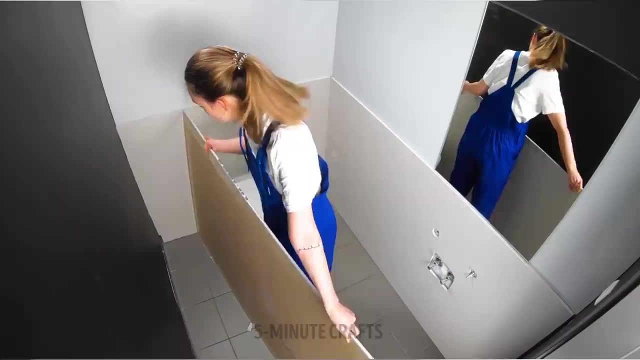 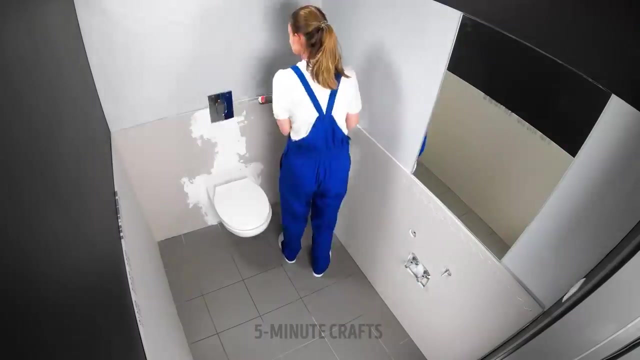 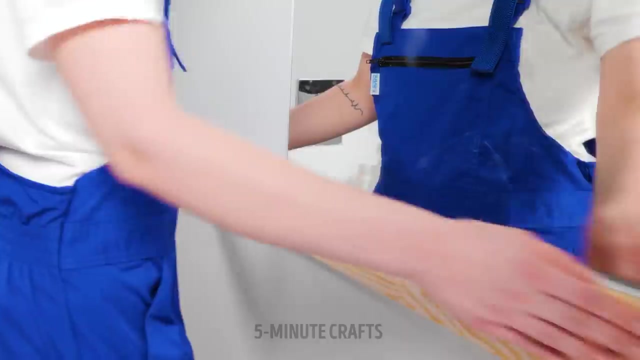 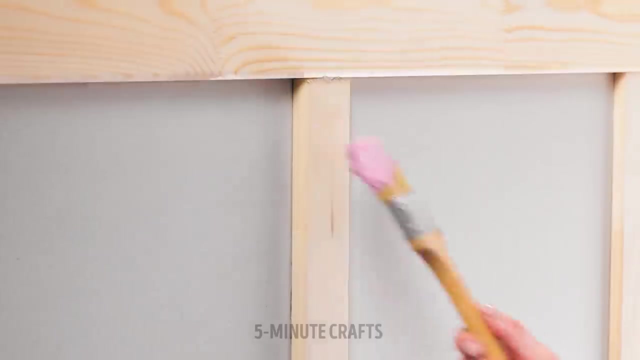 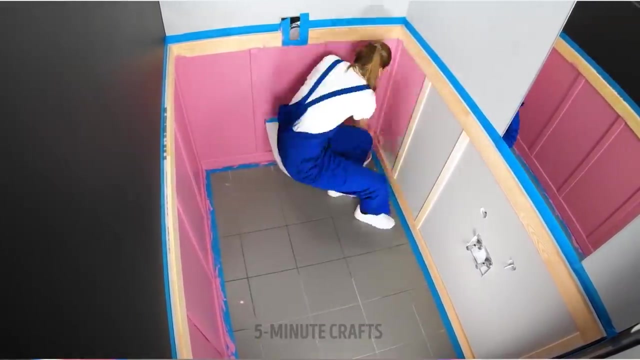 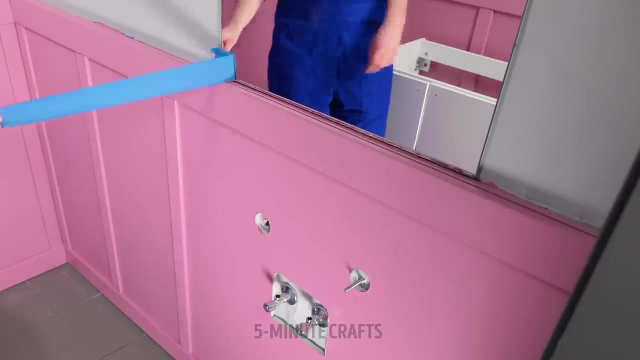 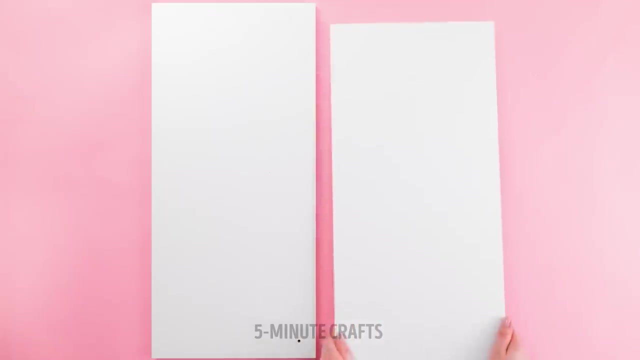 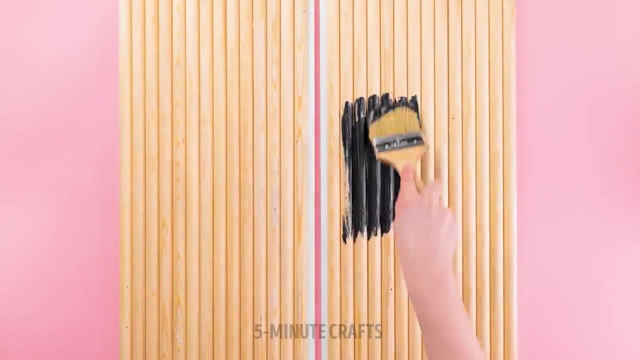 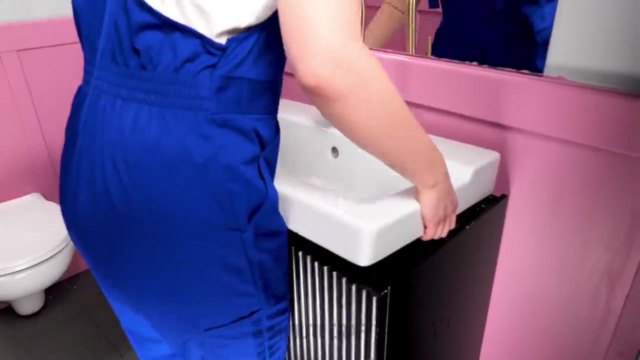 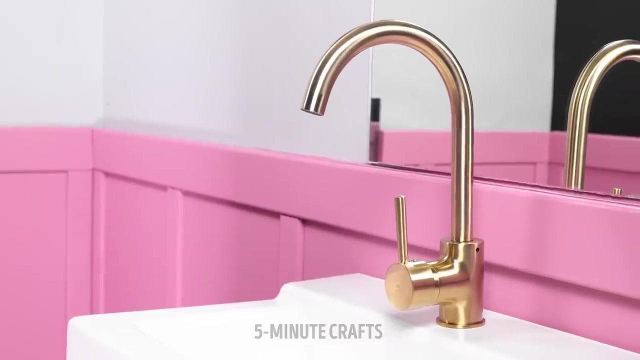 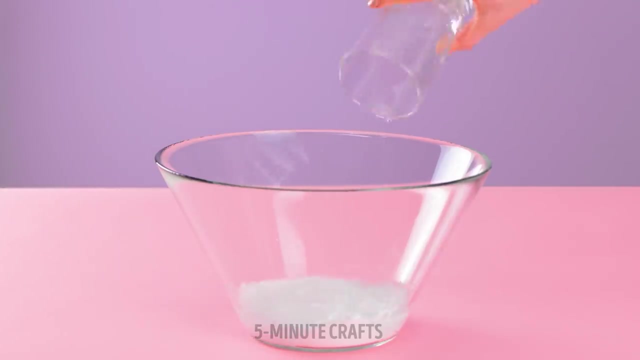 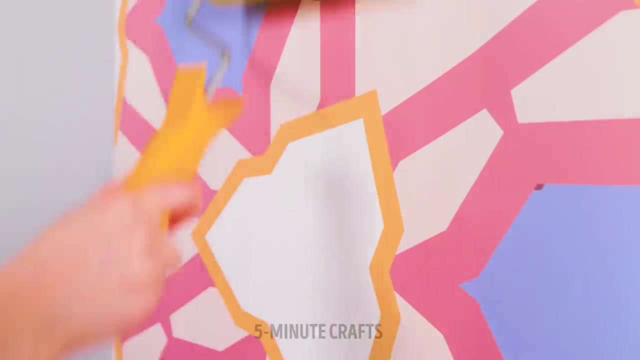 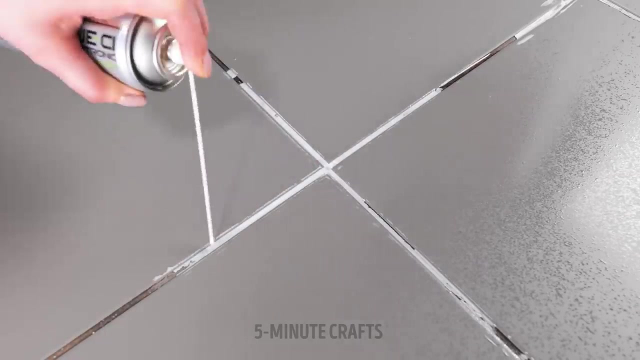 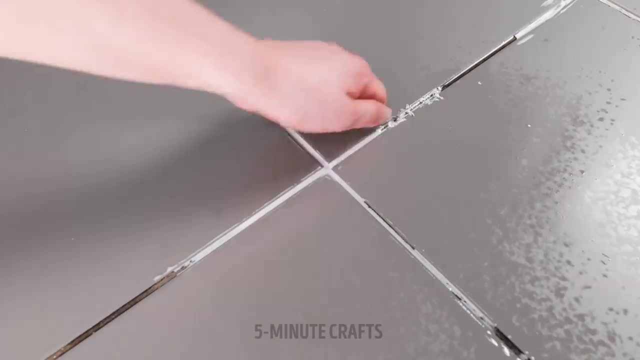 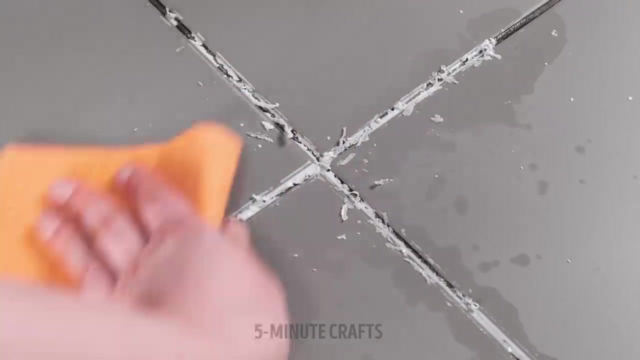 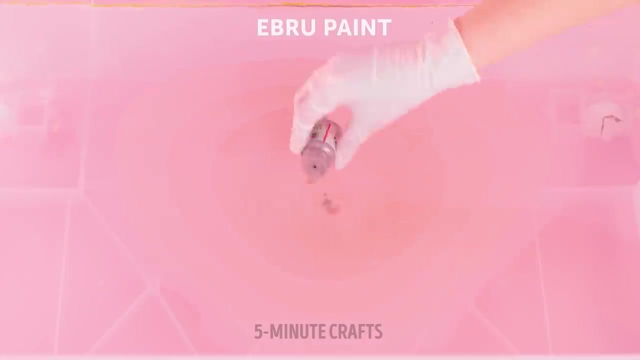 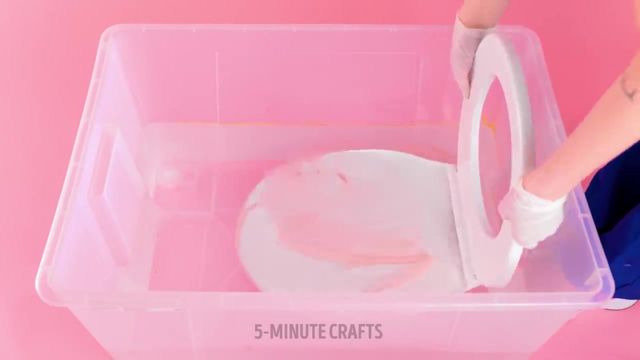 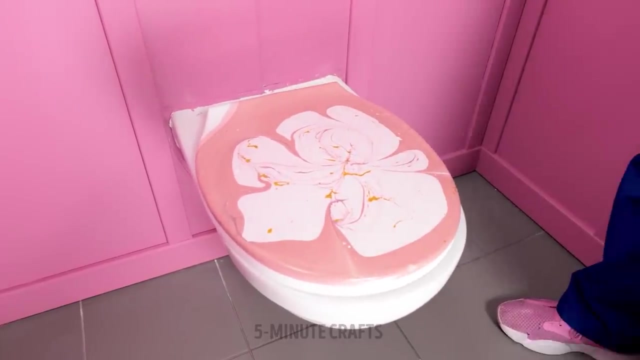 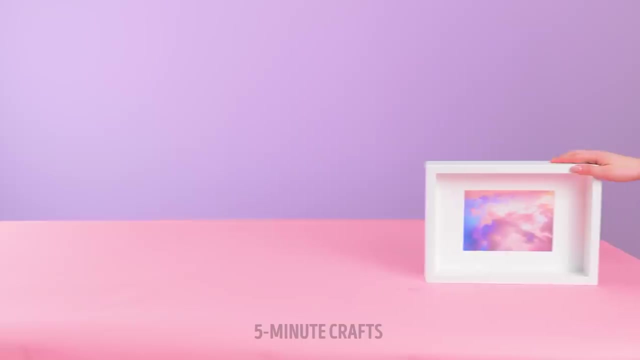 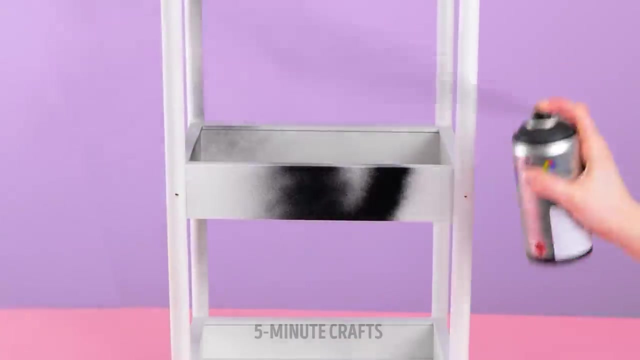 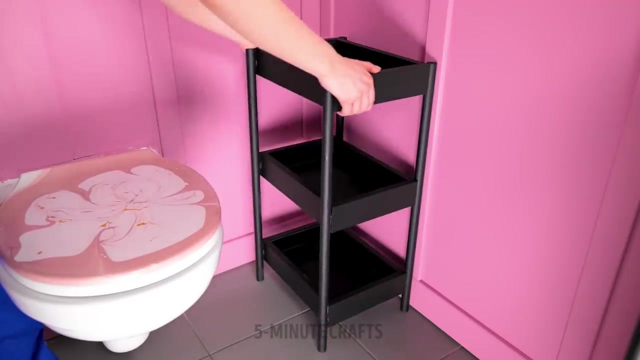 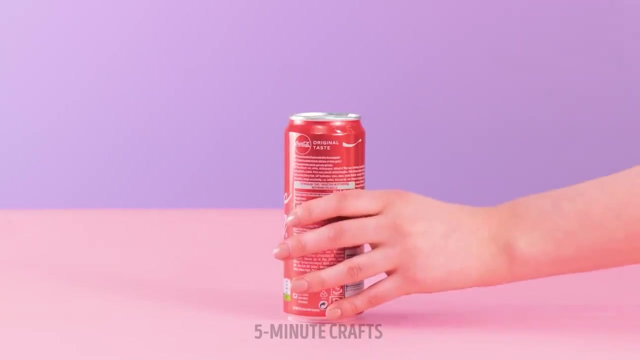 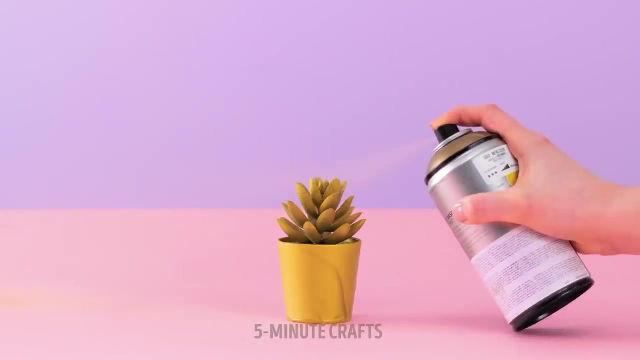 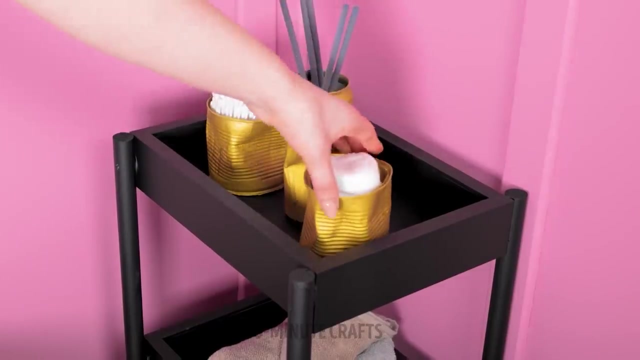 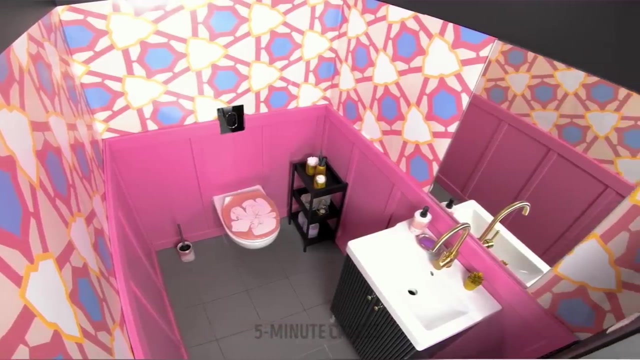 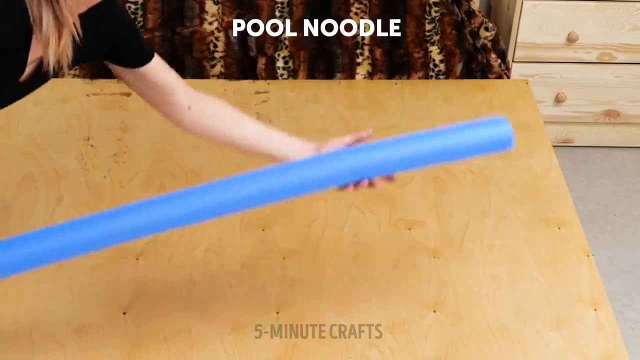 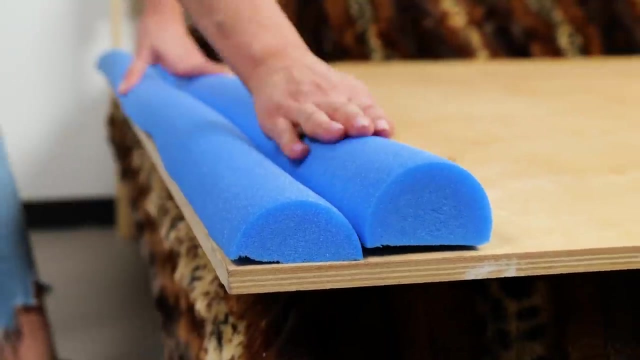 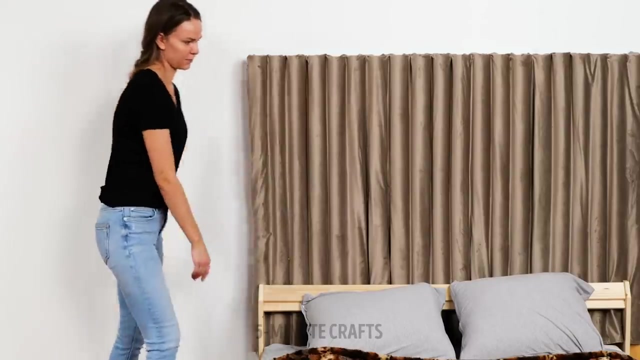 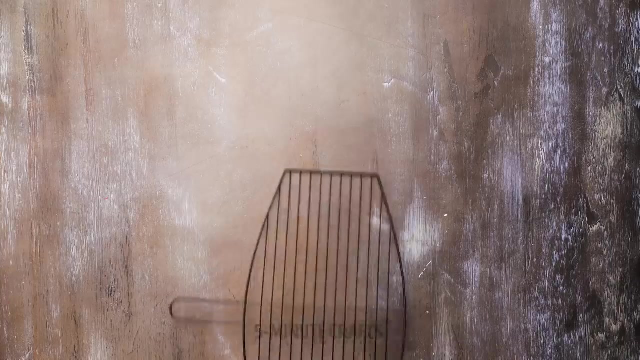 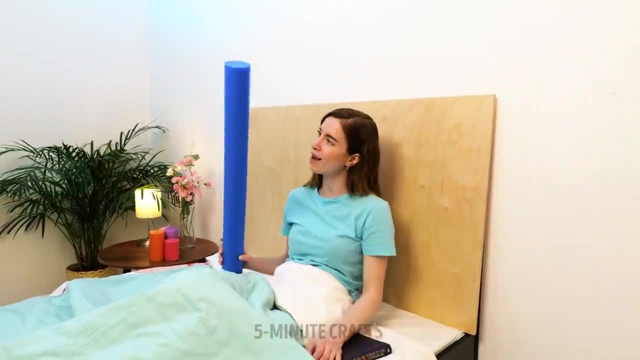 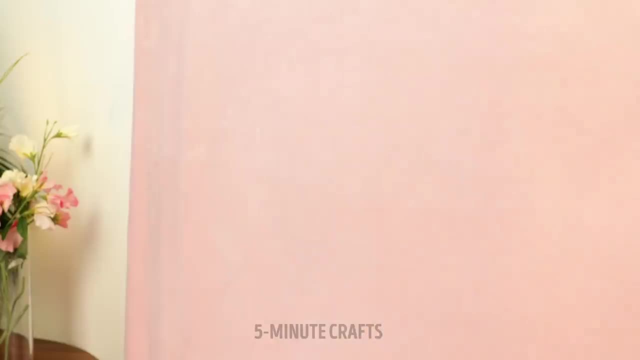 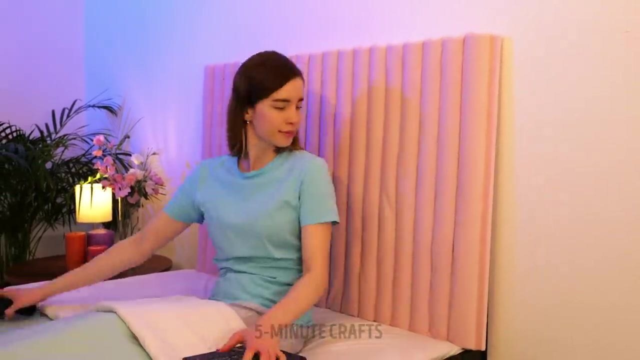 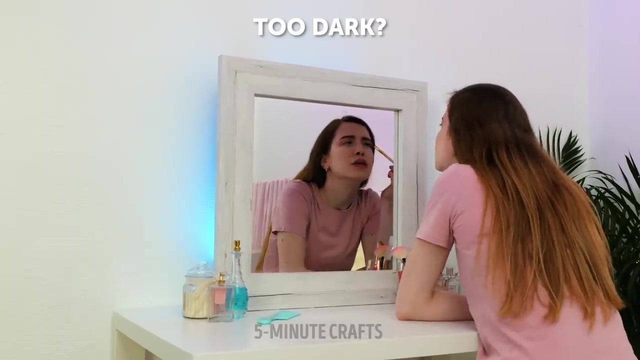 I will go if nothing changes. So change your heart. Ooh, your mind is a ghost town Echoing inside your walls, Five feet underground. now, Nothing's gonna save us from our doubts, Nothing's gonna make us. I spell it out. 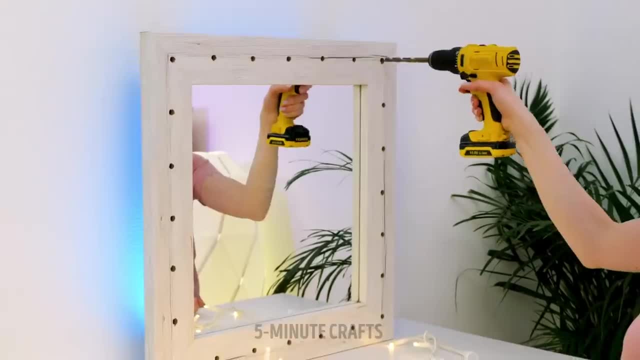 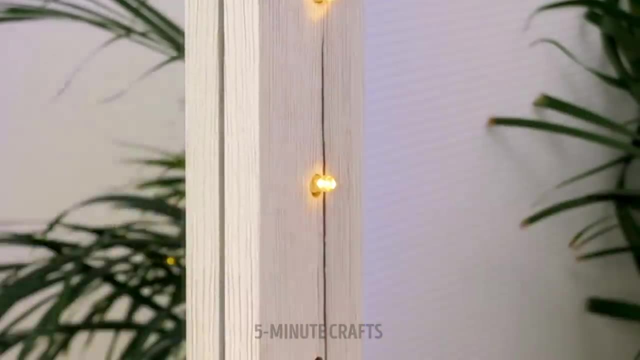 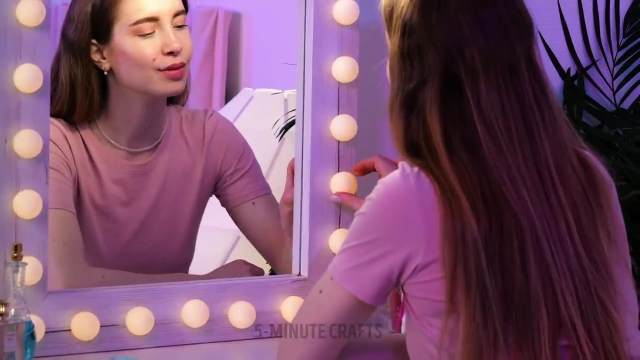 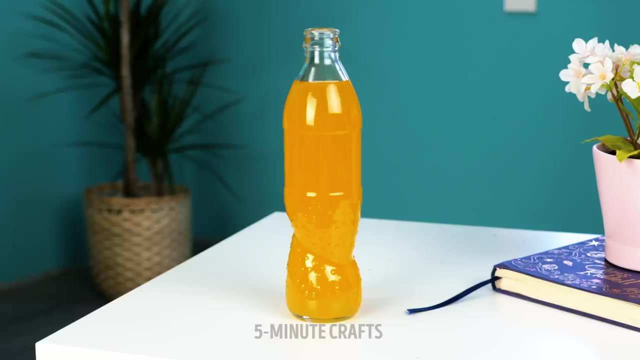 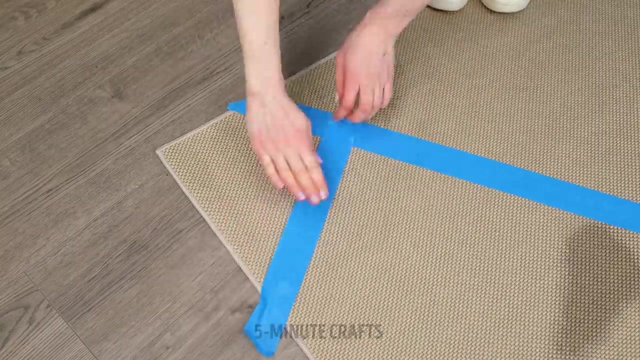 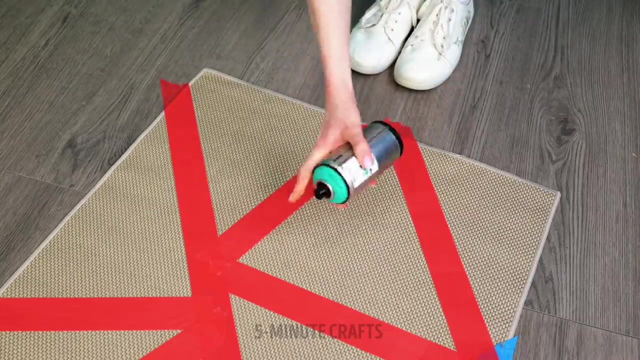 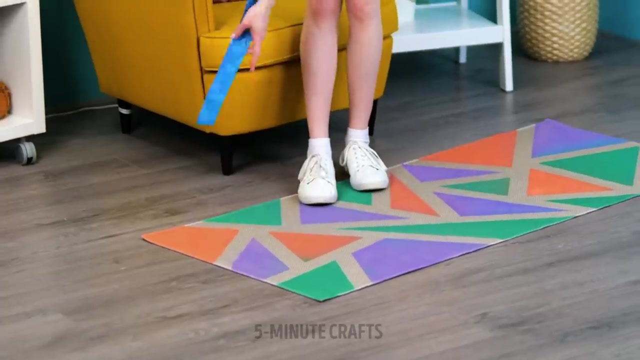 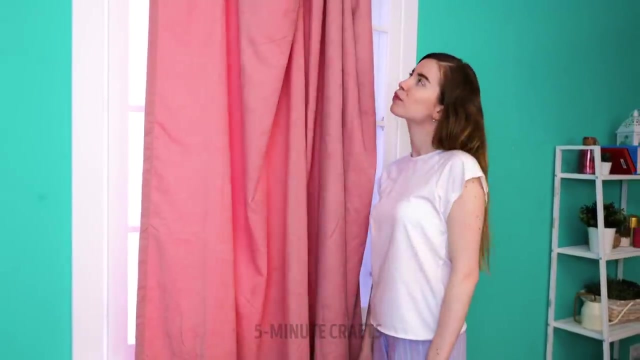 I don't wanna be the one to say: Oh, I told you so, But I told you so. My kingdom of lockdown, You never give me any chance. Watch me on my way out. Nothing's gonna save us from our doubts. 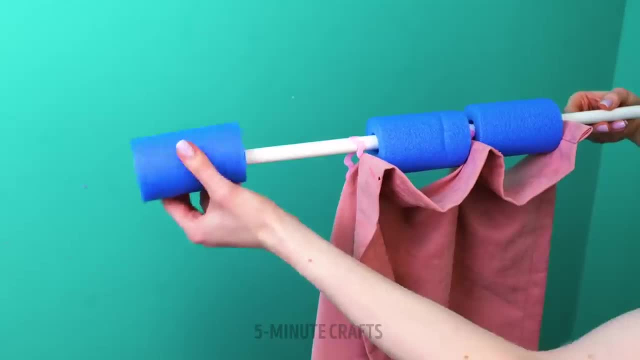 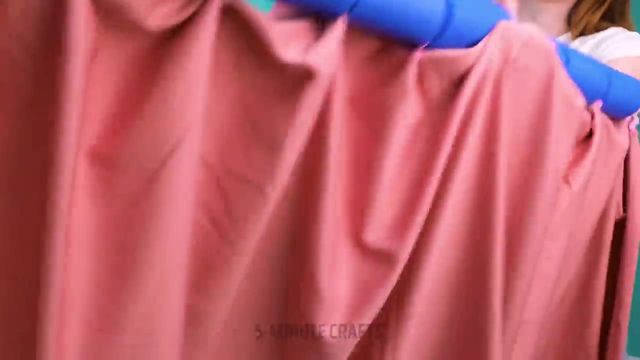 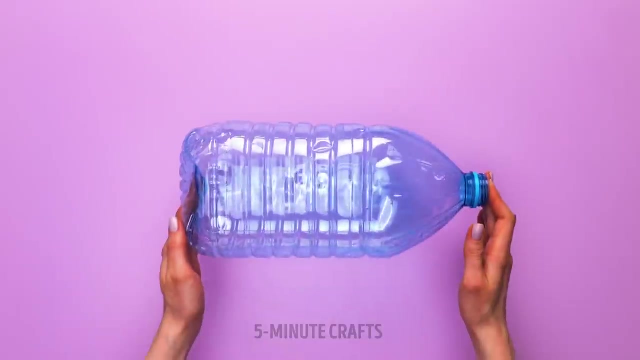 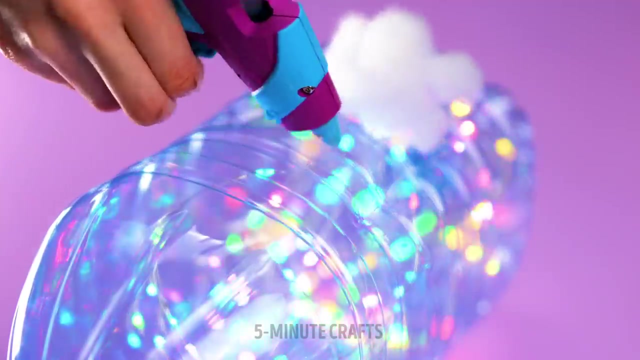 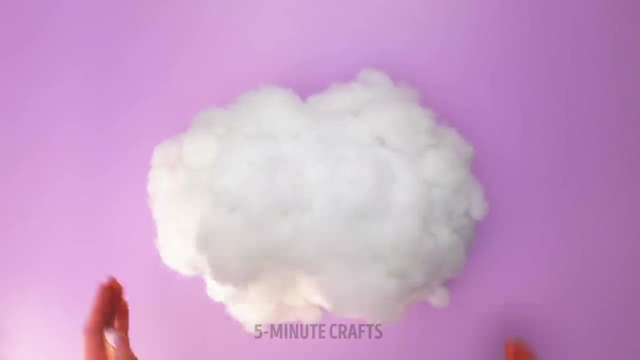 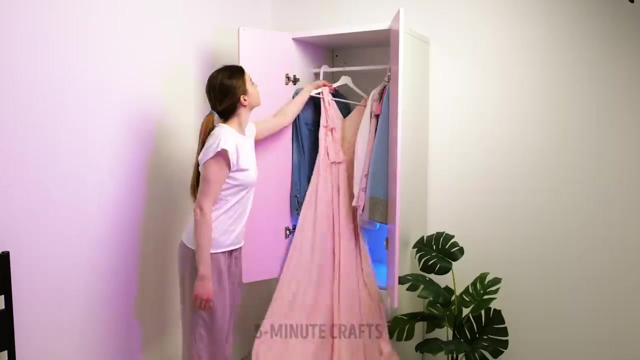 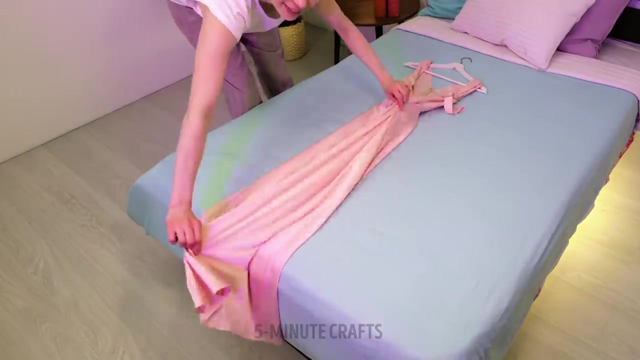 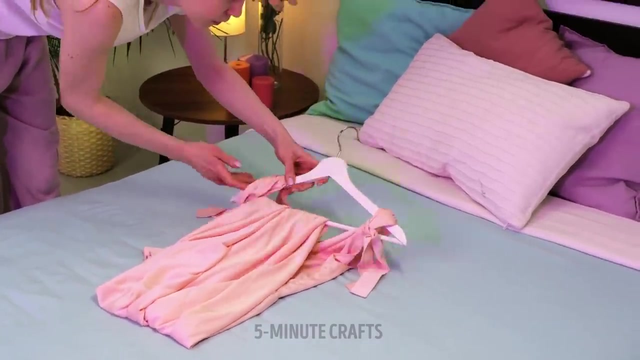 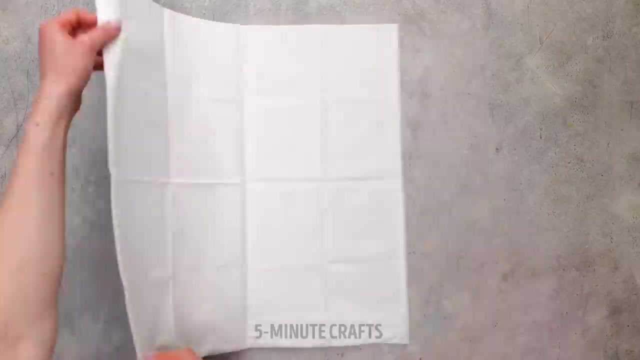 Nothing's gonna make us. I spell it out. I spell it out. I don't wanna be the one to say, Oh, I told you so, But I told you so, But I told you so We'll be right back.